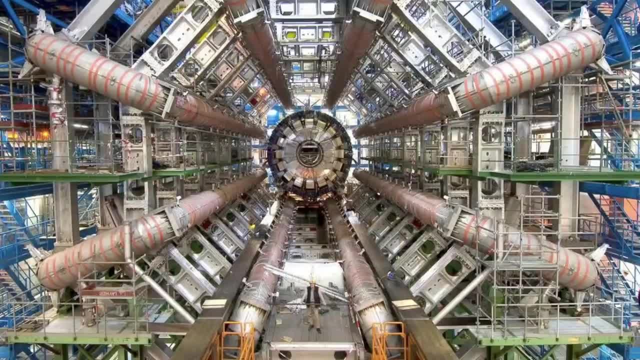 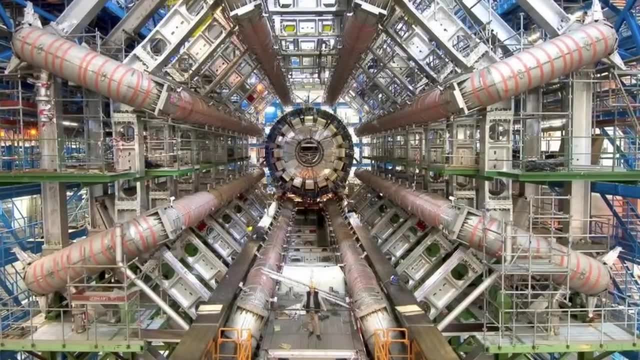 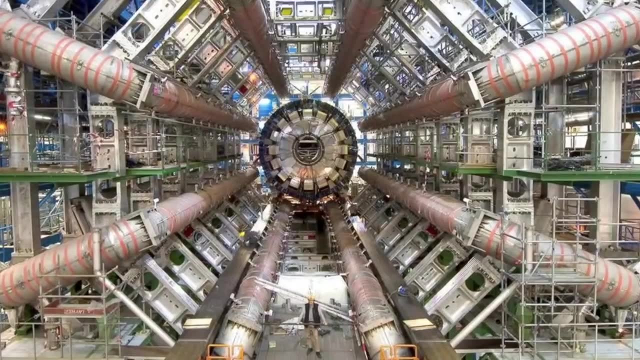 distant worlds with their own moons. Scientific instrumentation today is a bit more complicated. Things like this- the Large Hadron Collider in Europe- crack open atoms. try to find new kind of physics to reconcile the problems in our existing theories of physics. But the data that comes? 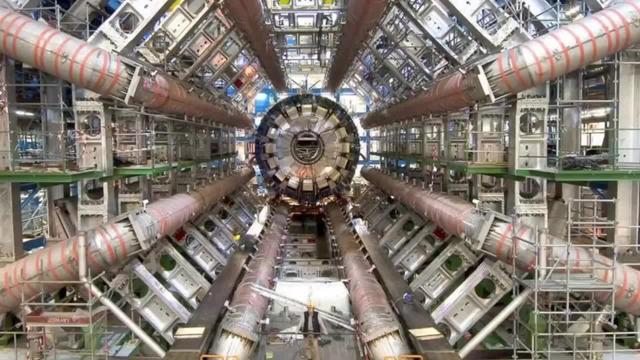 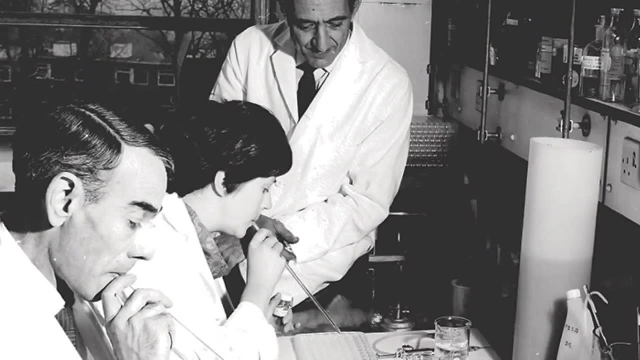 out of something like the Large Hadron Collider is not really useful without parallel advances in statistical computing, in data analysis algorithms and in the hardware that makes it possible to move all this data around, And together with that we require some parallel cultural evolution in how to use the data. 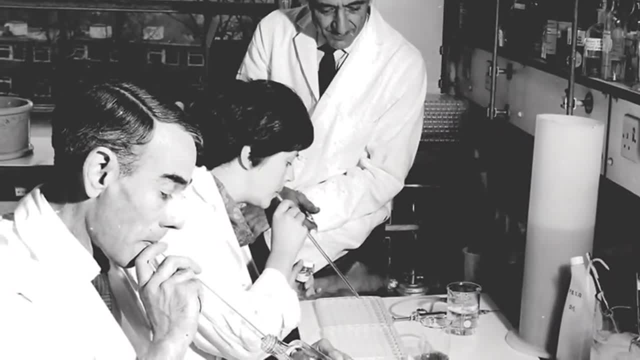 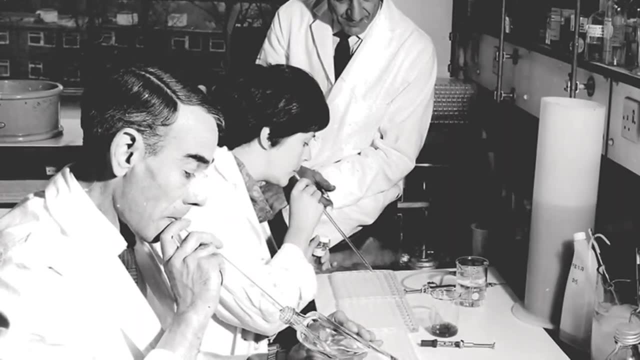 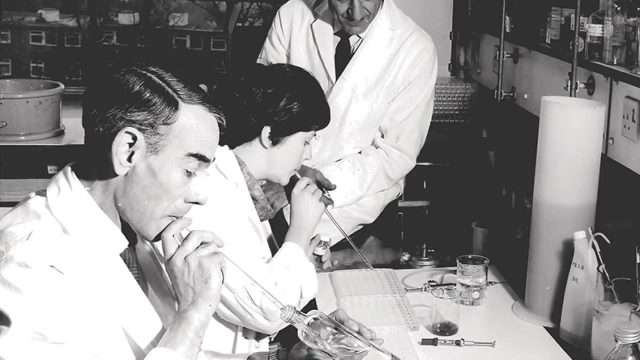 processing and scientific computing responsibly, so that it actually gives us answers and not just illusions. Here you see scientists of a previous era pipetting with their mouths, something that would be considered completely unsafe and even grounds for firing in many laboratories. Lots of statistical computing is, unfortunately, like pipetting with your mouth. 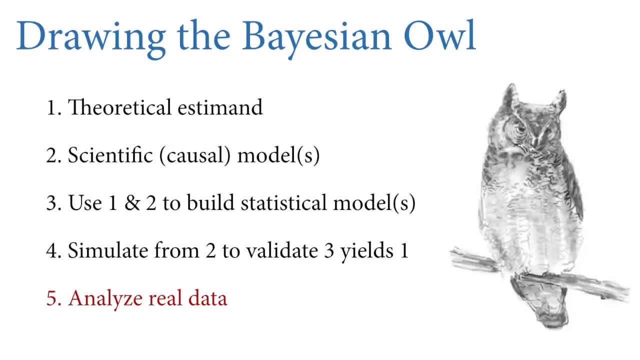 For this lecture. I want to talk about the scientific computing part of drawing the Bayesian Owl, this workflow from the first lecture. It's important to get the theory right in step one, have some clear communicated theoretical estimand predict the 윈ält. 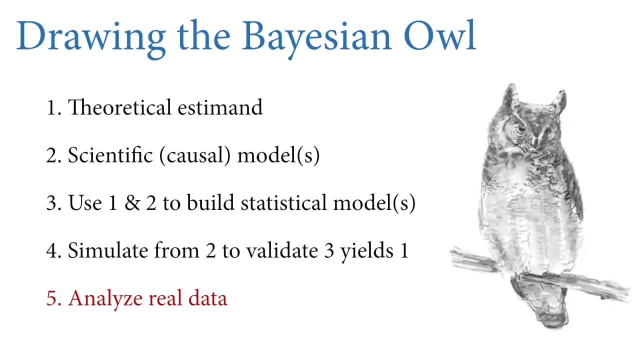 You need to have some way to translate scientific assumptions into structural causal models and then you need to use logic to get that causal logic into statistical modeling. But in step five here I think I've let you down so far in the sense that I haven't really said that much about the scientific computing part of data analysis for realistically complicated problems. So far we've done a lot, but now I am perfectly satisfied with my data analysis work. 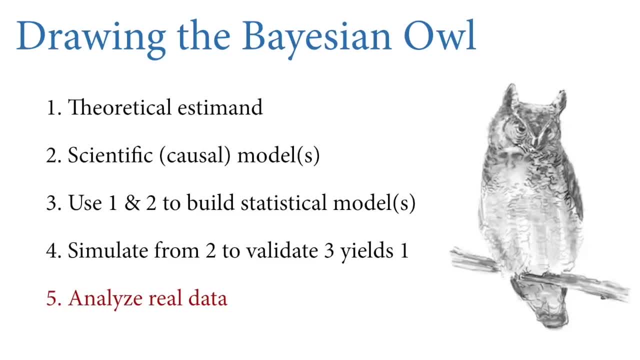 basic linear regression and i've hidden a lot of the computational details from you and to a large extent we can do most of our scientific work with the computational details black boxed away where the experts have safely secured it. but this lecture is for this lecture. i want to open that. 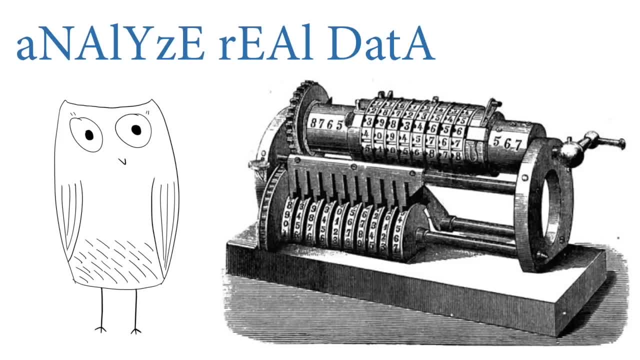 box a bit, because there's a lot about the way that modern computing works, especially bayesian computing, that requires you to know something about what's going on inside the golem, as it were. so we say we're just going to analyze the data, if your response is to be a bit sarcastic, 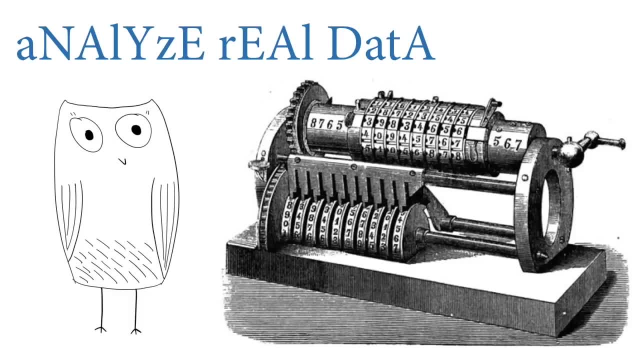 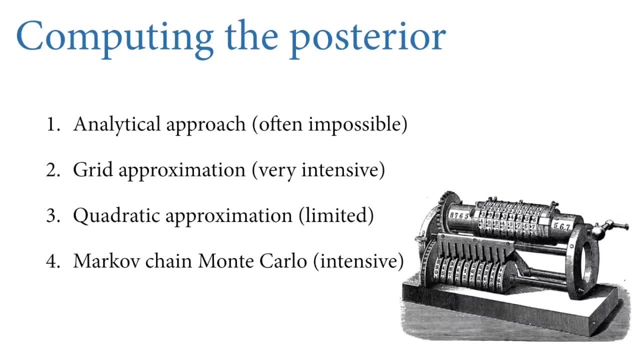 that's fair. there's a lot that goes on in this little step five of analyzing the data. there are lots of different machines you can use to compute the posterior distribution or get some approximation, rather, of the posterior distribution. um the first is this analytical approach, the classical approach, 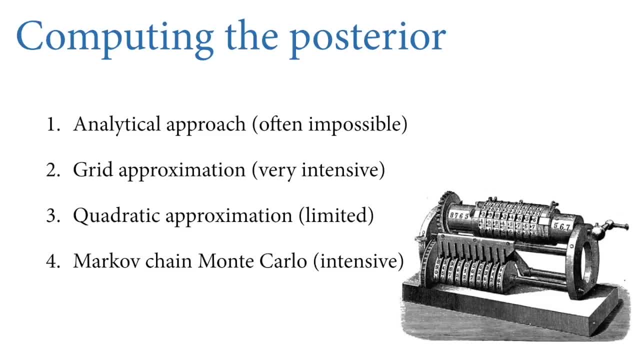 i've shown no examples of it in this course because it is completely unimportant aside from understanding the logic of bayesian analysis, but it's not useful for even simple problems. the second is grid approximation, which i showed you in the second lecture. grid approximation is a great way to understand what bayesian updating is about. 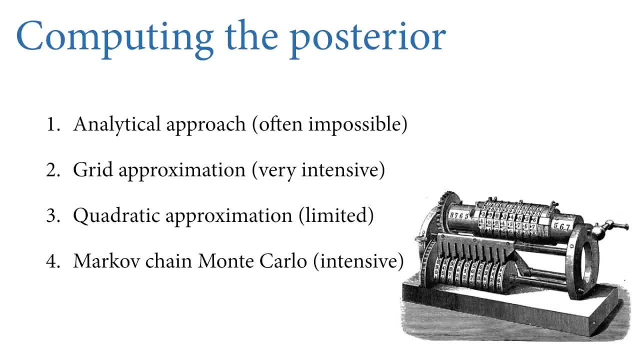 as it reinforces that. it's just counting, counting all the possibilities for every possible explanation of the data and then showing the relative numbers of ways that each explanation is compatible with the data. but grid approximation is just too computationally intensive. as models get more complicated, that is, the dimensionality of the problem grows. 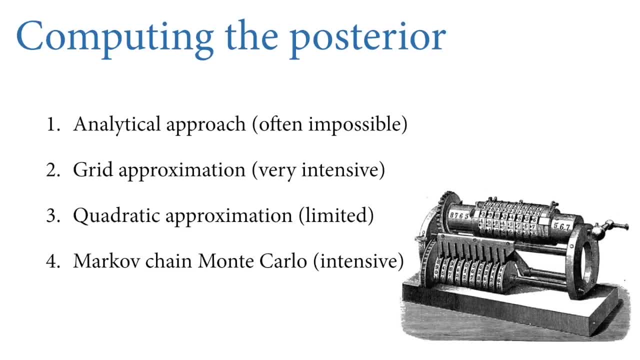 even the fastest computers in the world are not fast enough to solve your problems within your lifetime. and then the third model is the corner grid approximation, which is basically to calculate. And then the third we've been using up to this point is quadratic approximation, or Laplace approximation it's sometimes called. 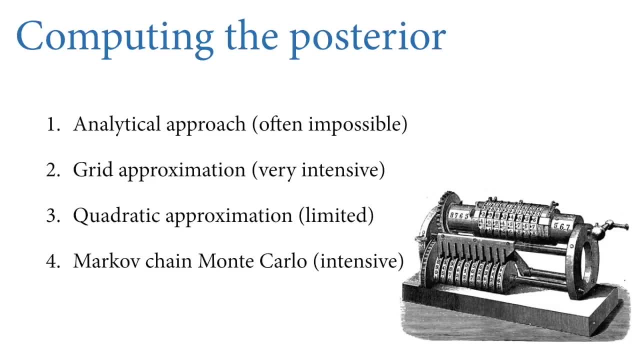 And this is where we approximate the posterior distribution as a multivariate normal distribution. This is a really valuable technique. It'll continue to be valuable for a very long time, But it's limited in the sense that lots of problems are not multivariate Gaussian. 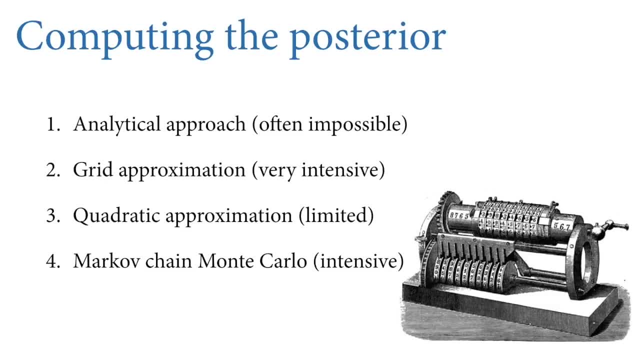 And we're going to start to use problems of that kind or encounter problems of that kind in this course now, And so we need some other option. So this lecture is about number four, Markov chain, Monte Carlo. Markov chain, Monte Carlo, is intensive, but it's not very intensive. 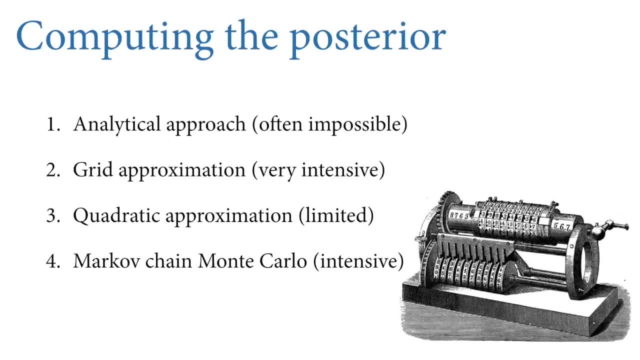 It's intensive in the sense that models that would take a second to fit with quadratic approximation might take a minute, Or half a minute to a minute with Markov chain, Monte Carlo. Maybe that doesn't sound like a bad ratio to you, But when you get into things that take ten minutes with quadratic approximation, 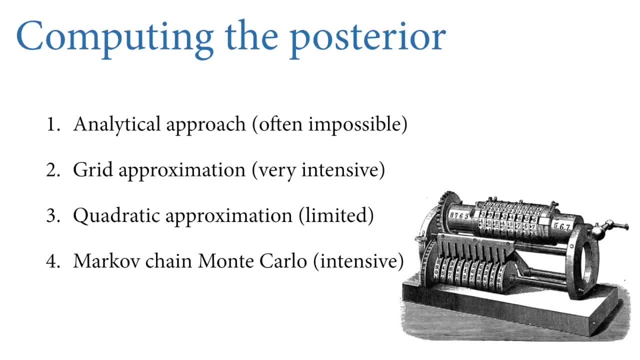 they could take hours or days with Markov chain Monte Carlo. So why would we ever use it? Well, the answer is because it's much more capable, It has many fewer limitations And, in fact, it has become essential in many areas of science. 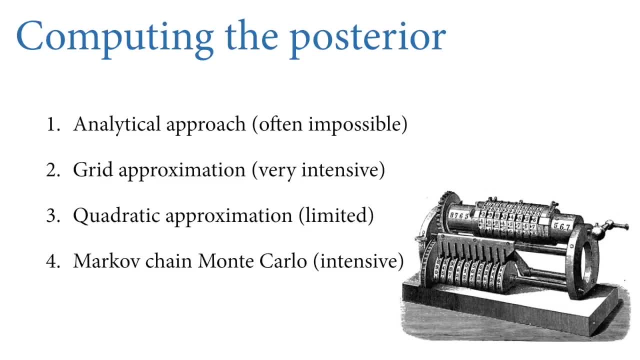 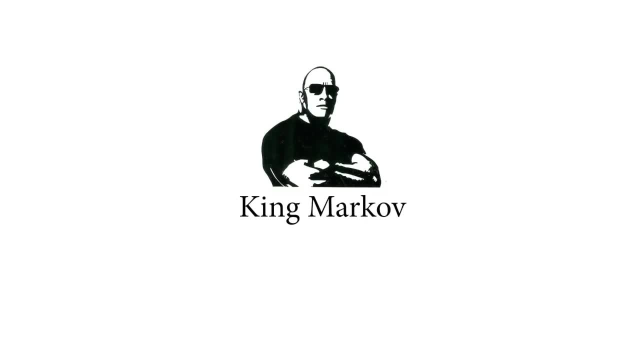 because it makes it possible to fit models to data that essentially nobody could fit to data before. Before we get into the details of it, though, let's think sort of as an allegory, And I'll walk you in a narrative way into what Markov chain Monte Carlo is. 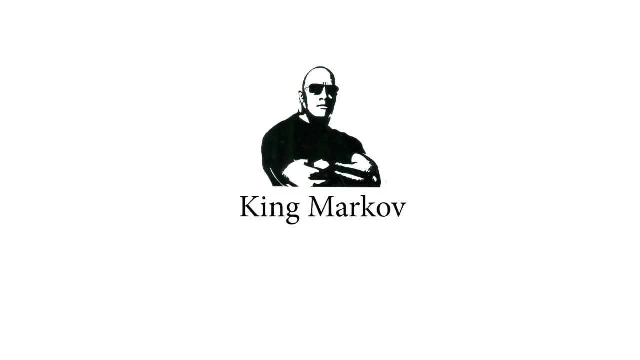 So imagine an oceanic king, a benign monarch named King Markov, pictured here. And King Markov is the benign ruler of an archipelago, the metropolis archipelago, And this archipelago has a number of islands in it. 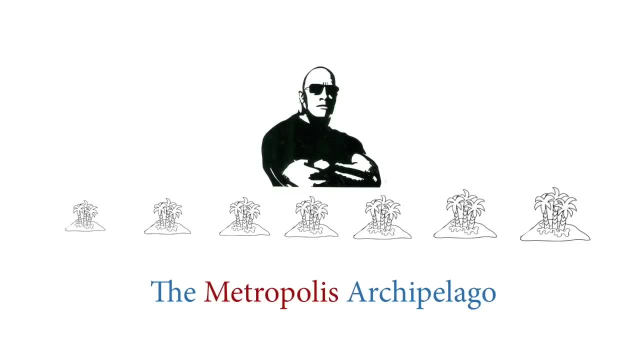 And the islands are different sizes And so they have different populations on them, different sizes of populations on them. And as a benign monarch, King Markov has this contract with his people that he will visit them, that his people love him, So he agrees to visit them. 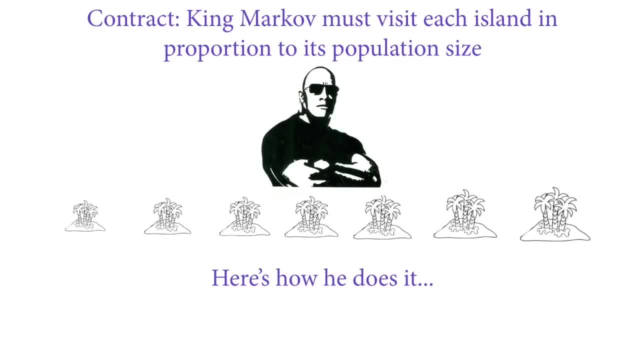 He will visit them in proportion to the population sizes of the islands they're on, And his advisors have gotten together And figured out a way that he can do this without any kind of calendar or schedule, because King Markov likes to live free. He's a bit of a bohemian. 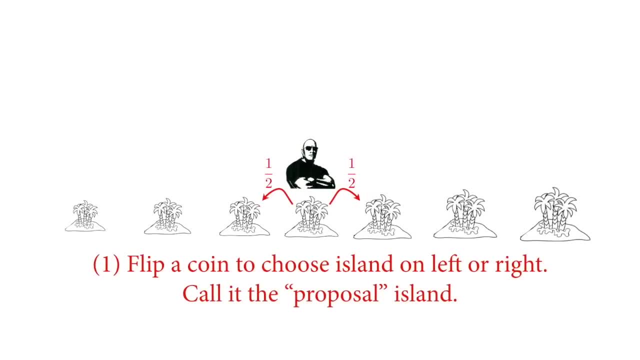 So here's how he does it. So he does a visit on an island And then at the end of that week of his visit he flips a coin to choose the island to the left or the right of the current island he's on. 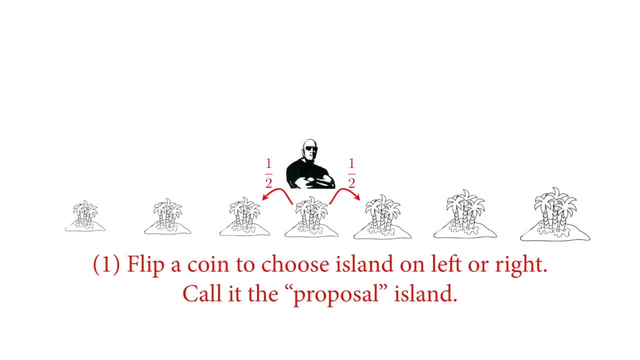 And he calls that island. whichever the coin chooses, he calls that the proposal island, And there's a half chance of proposing the left or the right. So suppose the proposal ends up being the right in this case, Then he will ask someone. 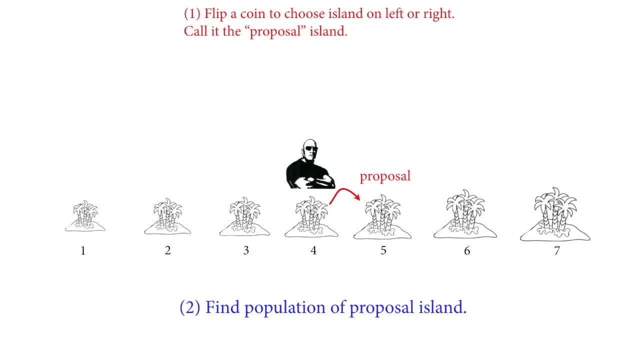 hey, that island over there, what's its population size? So he gets an estimate of the population size of the proposal island. Let's call that P sub 5. And he compares that. And he compares that to the population of the current island. 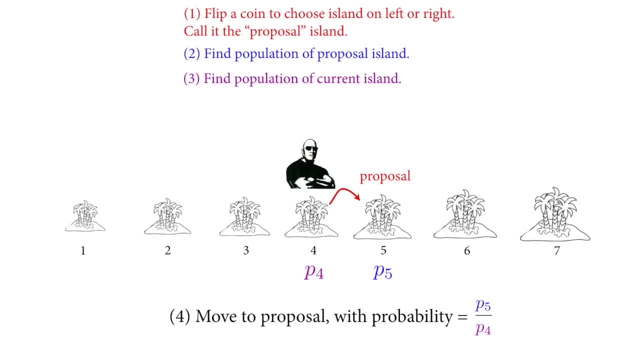 which we'll call P sub 4.. And then he moves to the proposal island with a probability equal to P5 over P4. Now this number can be greater than 1. In that case he always moves, But if it's less than 1,. 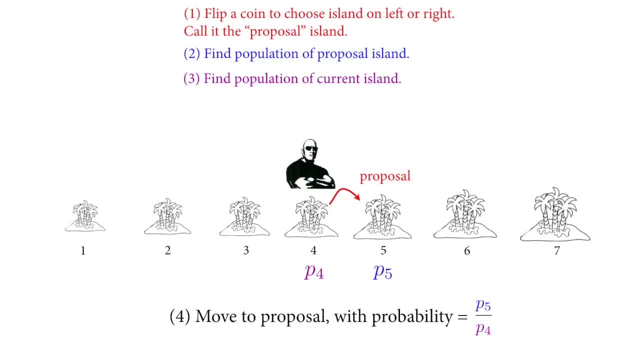 then he uses a bag of seashells or some dice as a randomization method to obey the probability, or a spinner wheel or a mechanism of that sort, And then he repeats from step 1.. He spends a week on. either he moves or he doesn't. 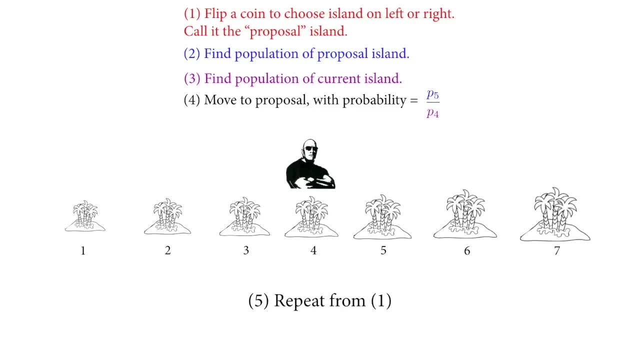 If he stays, he spends another week on island 4.. The people of island 4 rejoice. Or he moves to island 5, in this example, And the people of island 5 rejoice. He spends a week there. Either way, at the end of the next week 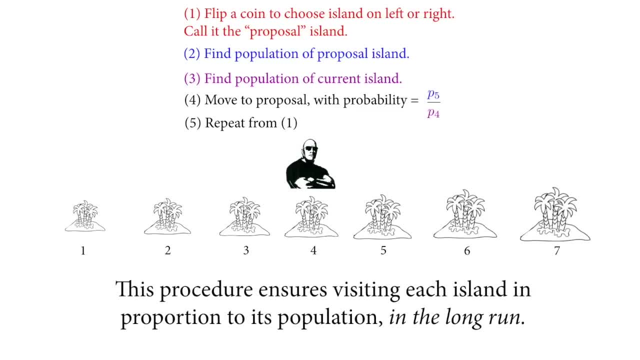 he repeats it all over again and starts over at step 1 and flips a coin. It turns out as weird as this procedure sounds, it ensures that, in the long run, King Markov will visit each of the islands in proportion to its population size. 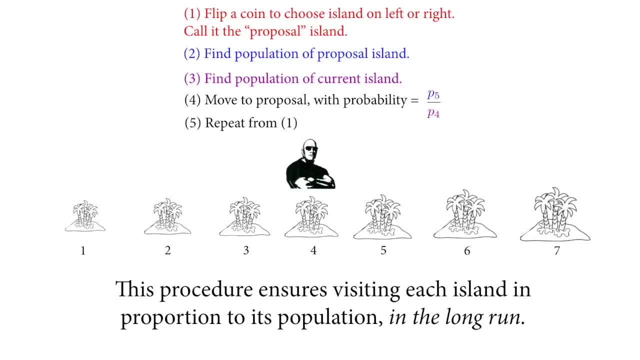 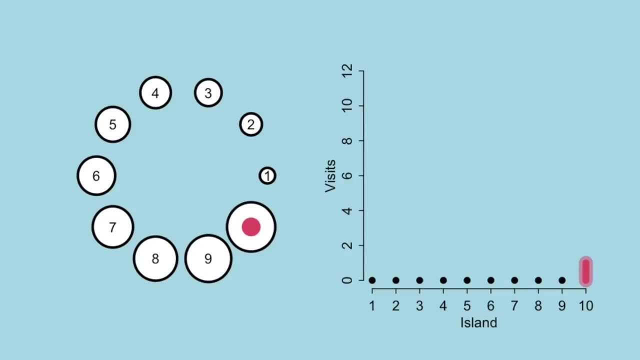 But only in the long run. In the short run, of course, he could stay on island 4 for 10 weeks in a row. It's not likely, but it could happen. Let's take that algorithm and animate it so you can get a sense about how it functions. 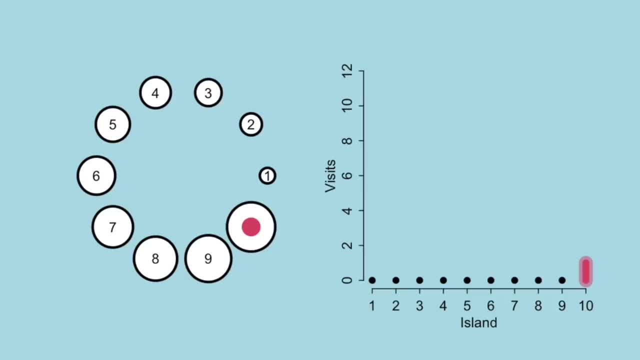 So what I've drawn on this slide on the left is the archipelago represented as a ring, so that you can loop from the smallest island, which is labeled with the number 4, to the number 1.. These numbers are relative to the population sizes. 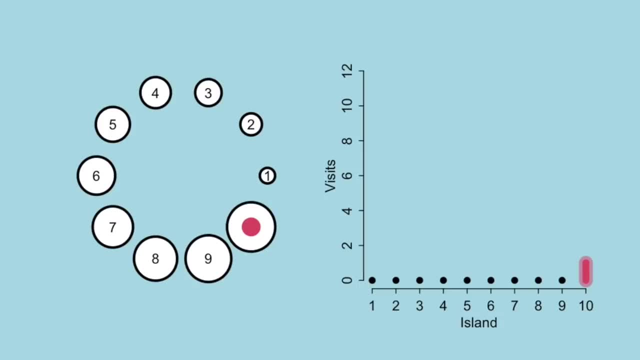 of the islands and they're drawn, so their areas are proportional to the numbers on them, And the largest one with the red dot on it, that's where King Markov is going to start in the simulation. That's the 10th island. 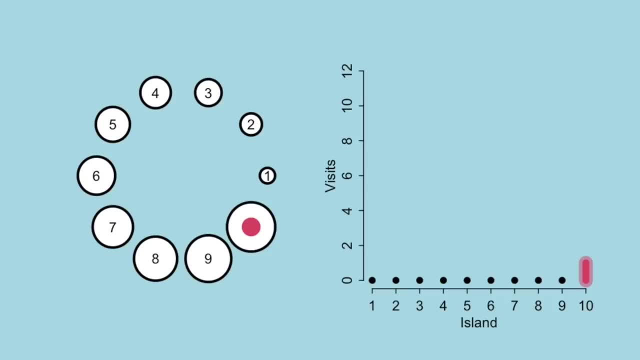 And on the right we have a histogram that is going to count up the numbers of visits he has made to each of these islands starting from now, And you'll see that he makes proposals and he leaps across on his little royal boat or he stays. 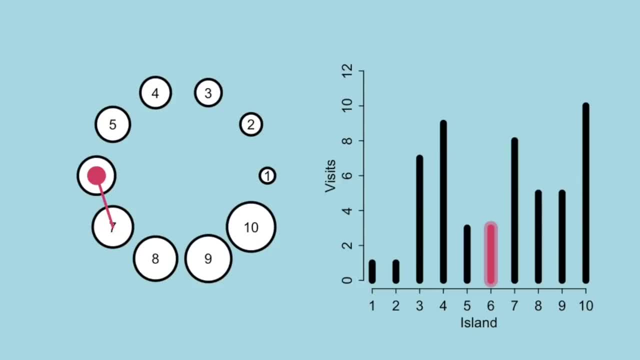 and then we count up weeks of visits on the right And you'll see that the bars grow And at first it's just a jagged mess. There's no real pattern, because it's incredibly random. There's no long-range plan here, remember. 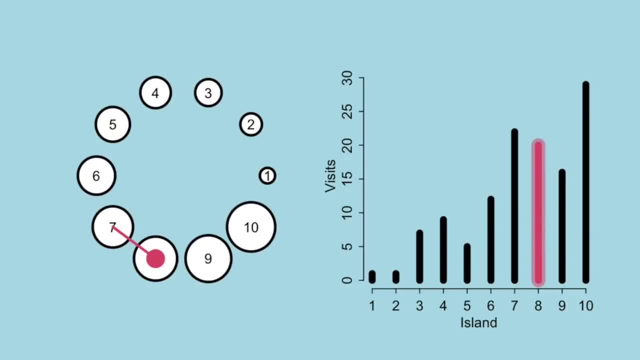 King Markov is not planning for the future. He's just deciding every week whether he stays or moves, and he does so with a random device. But quickly you start to see that he spends more time on big islands because jumps to bigger islands are more likely. 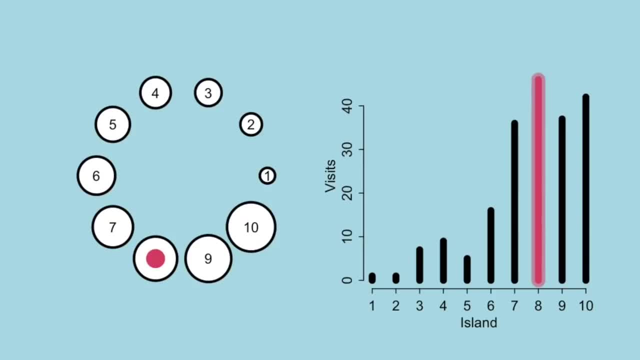 than jumps to smaller islands. But jumps to smaller islands are possible. So in the very long run, after several hundred visits, you'll see that the pattern is well established and he tends to visit each of the islands in direct proportion to its relative population size. 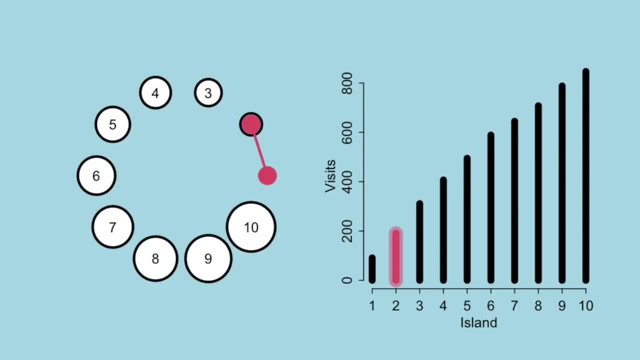 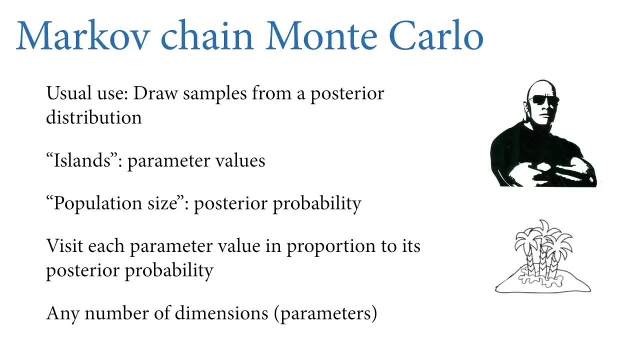 relative to the other islands in the archipelago. This algorithm. of course, it doesn't really have anything to do with oceanic monarchs. This is an example of Markov Chain, Monte Carlo. Our usual use of it in scientific computing is to draw samples from a posterior distribution. 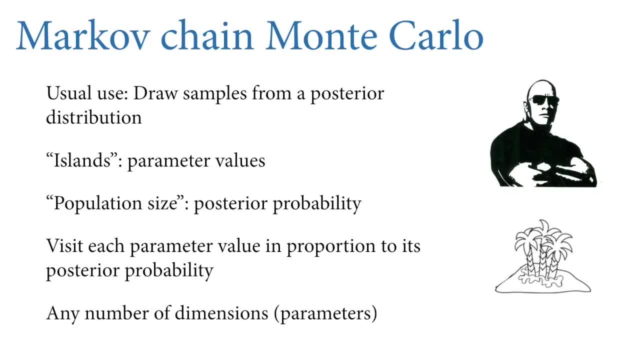 or really any distribution, but we're going to use it in this class for posterior distributions. The islands in the example are the parameter values, the explanations of the data that we've been interested in up to this point in the course, And the population sizes. 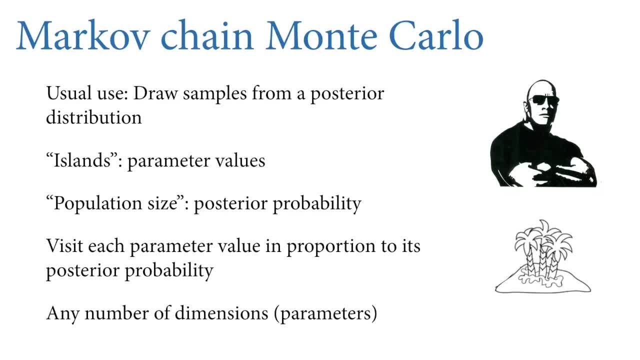 are the posterior probabilities of each of those parameter values, each of those explanations, The relative numbers of ways that that parameter value or island could explain the data And what the algorithm that I just showed you does is. it guarantees that, in the long run, that the computer will visit. 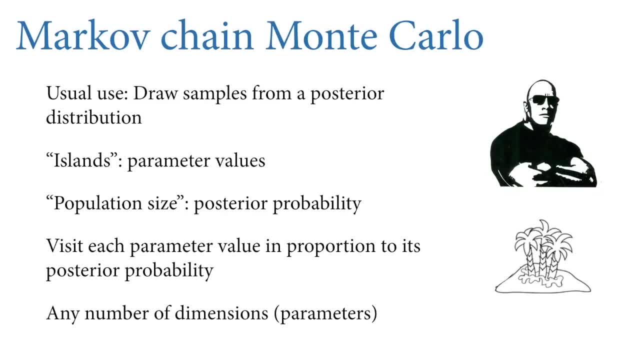 each parameter value in proportion to its posterior probability. And all you need to be able to do computationally is compute the posterior probability for any specific combination of the parameter values, one at a time, So you don't have to evaluate like in grid approximation. 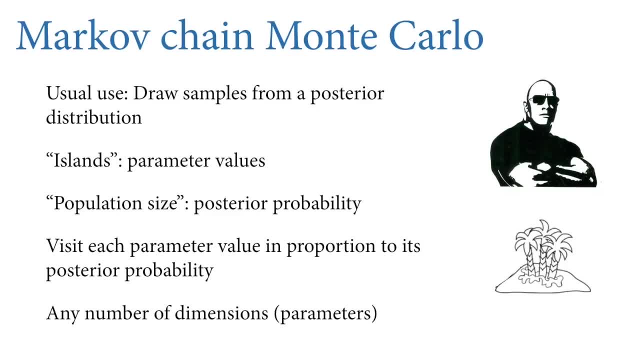 the entire grid. You just do the proposal and your current location. so it's just two posterior probabilities, two little spots in the grid, and that's what you need to know if you move And at every step, every proposal, step again. there's just two numbers to compute. 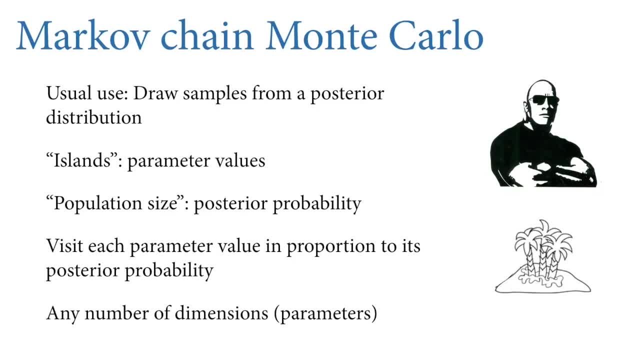 This algorithm scales up to more dimensions. In the islands example, there's just one dimension, That is, there's just the location, the island that King Markov is on. But of course we often have many parameters in our models And this algorithm. 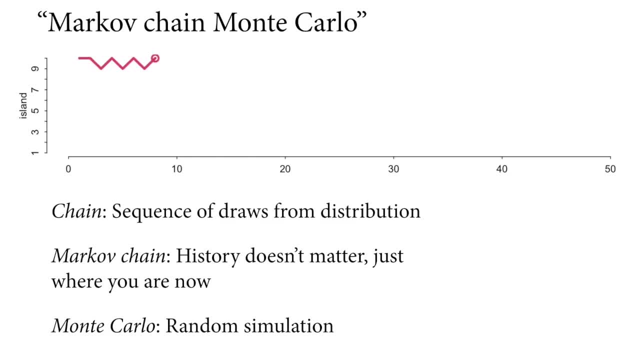 can handle that as well. It's called a Markov chain because it's a temporal sequence, That is, the values are sampled in sequence and the next sample or the next proposal only depends upon the most recent one. So, as I'm showing here on this slide, 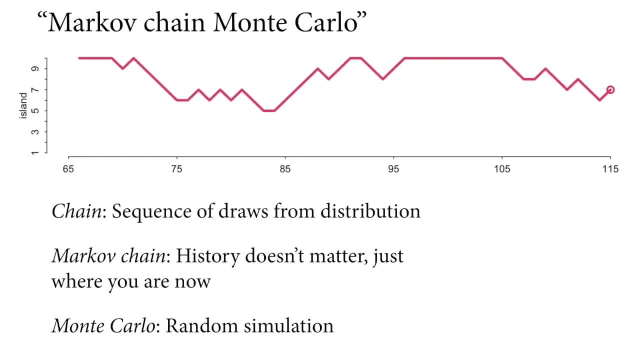 you can represent it as a migration through time from the left to the right, with increasing samples. This is King Markov on the far right there, wandering around, and the path behind him is the Markov chain, so to speak, the chain of visits that he's been at. 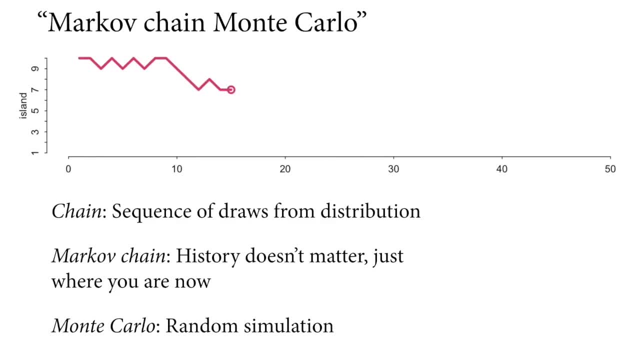 You can see he tends to spend more time near the top of this plot because those are the populous islands, but he does wander to the islands with smaller populations, and he does so in the long run, In proportion to their population size. So this is a key feature. 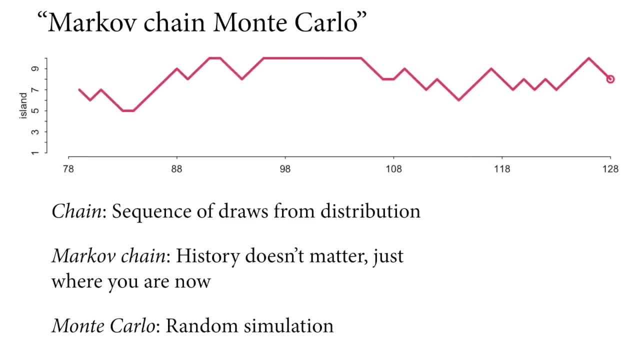 of the Markov chain is that? what makes something a Markov chain is that history doesn't matter. Where you're going to go next only depends upon where you are now, And that's why King Markov doesn't need records or any planning or any calendar. 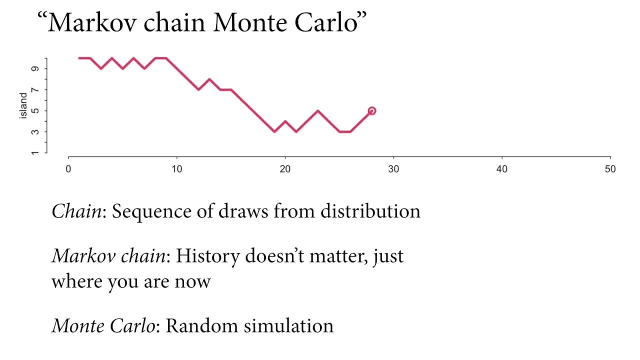 And that's what he likes about it. The Monte Carlo part of Markov chain. Monte Carlo just means some numerical algorithm that uses randomization, Randomization, to perform a calculation, And there are lots of Monte Carlo techniques in the sciences. Markov chain, Monte Carlo. 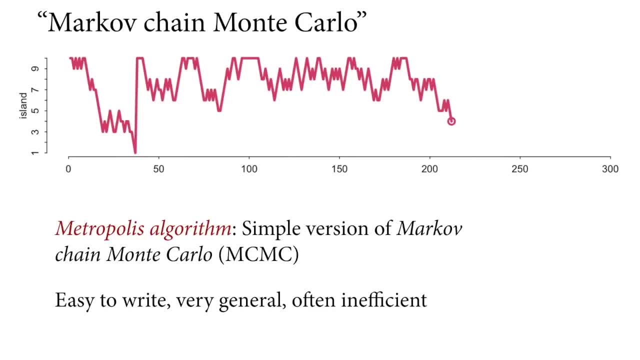 is only one of them. So here I've zoomed out on that same chain. You can get a sense now of how the visits aggregate in the more populous islands. You can see it a little better. This particular algorithm that's animating at the top here. 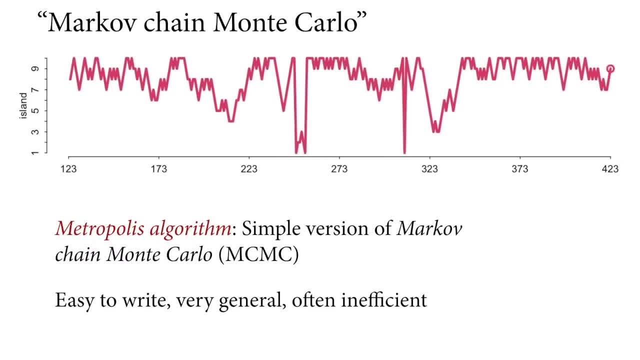 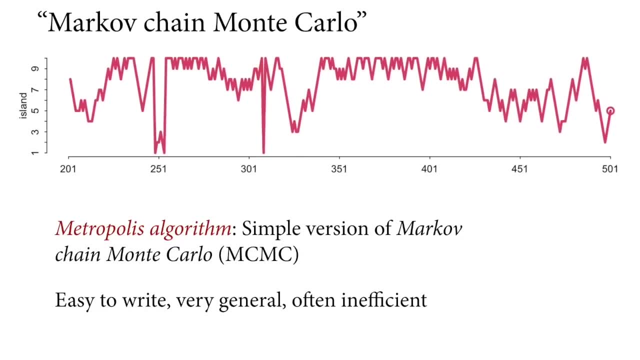 is known as the Metropolis algorithm, And it's a very simple version Of Markov chain Monte Carlo, Or MCMC as it's usually abbreviated. In fact, it's the original one, And I'll talk more about that in a moment. 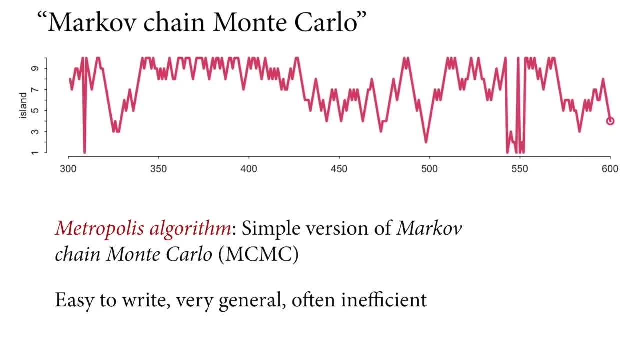 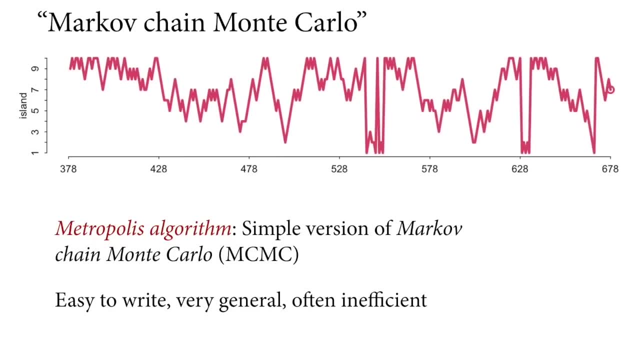 It's very easy to write it. So in the book I have a small example. You can do it in half a dozen lines of R code or any other scripting language, And it's very general. You can apply lots of problems to it. 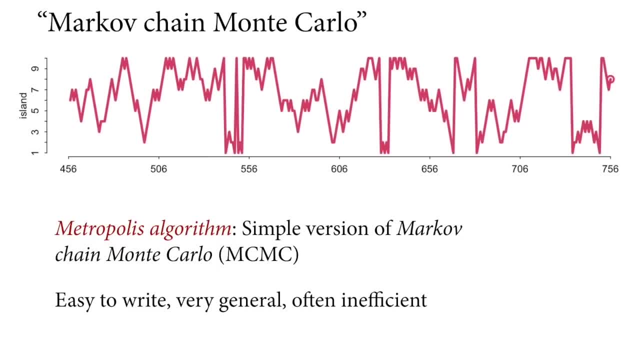 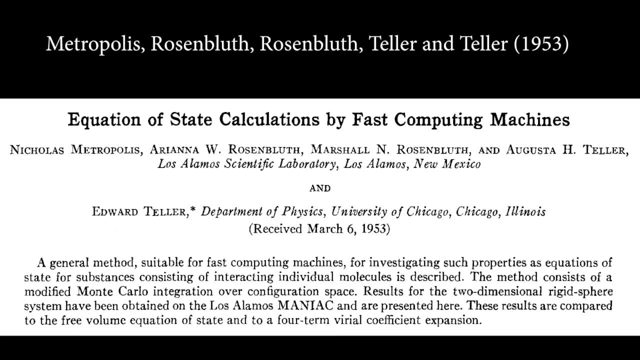 However, it's often inefficient, Especially as the domain name and dimensionality of the problem grows. It can be quite hard to tune it and make it work. This Metropolis algorithm comes from this paper shown here. It's a very famous paper in the computational sciences. 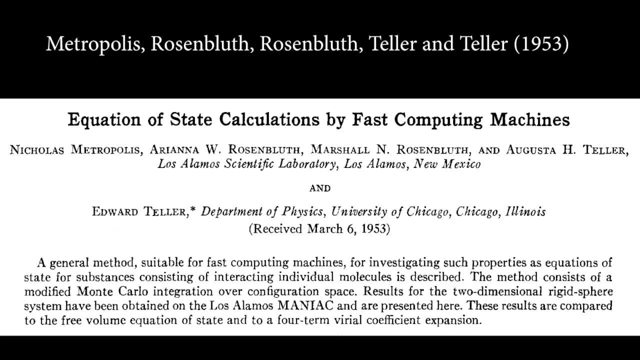 The Metropolis Rosenbluth, Rosenbluth, Teller and Teller in 1953. With a very exciting title: Equation of states: calculations by fast computing machines. This is one of those papers that started a whole new field, Not just a field. 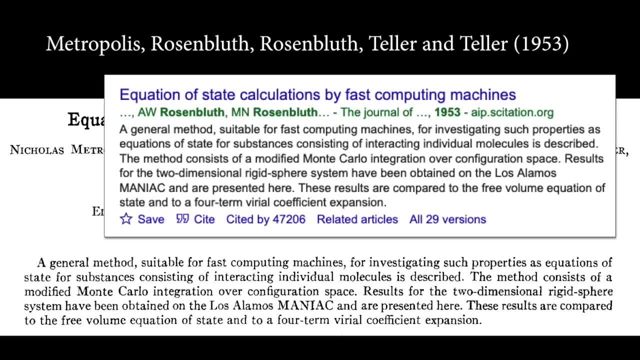 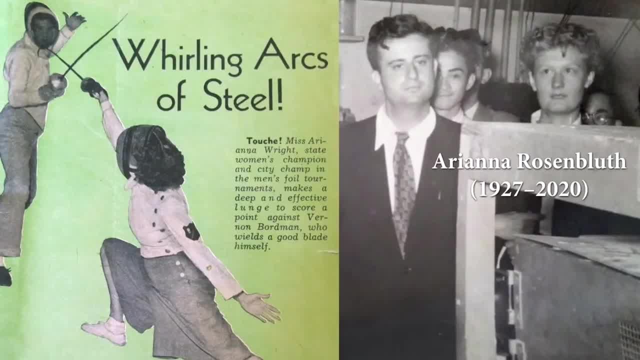 But a bunch of solutions that span individual scientific fields. It's been cited over 47,000 times by the latest count. This is an incredible piece of work And the bulk of the computational work, I think nearly all of it- was done by one person. 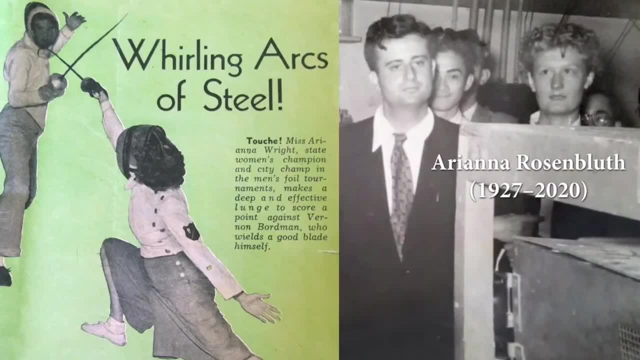 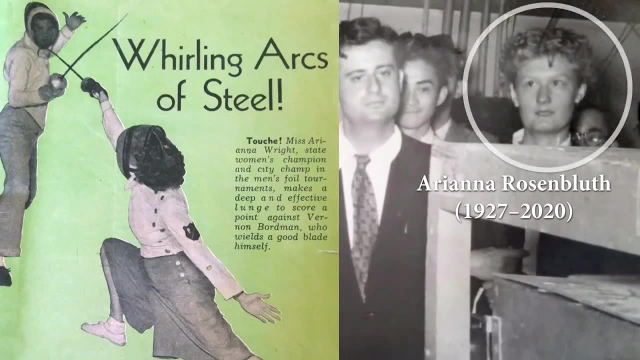 One of the authors, Ariana Rosenbluth, Who's pictured in the upper right of this slide. She's also the person lunging there in the foreground on the left The fencer. Ariana Rosenbluth was an Olympic fencer. 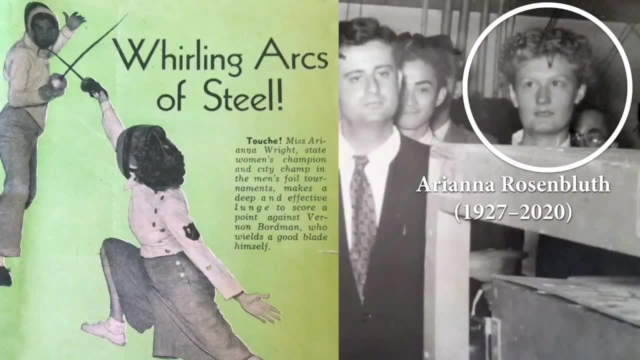 Qualified for the Olympics, But World War II prevented her from competing. And then she went on to get a PhD in physics from Harvard And then to work on the Manhattan project in Los Alamos, where she programmed machines to do all manner of simulations. 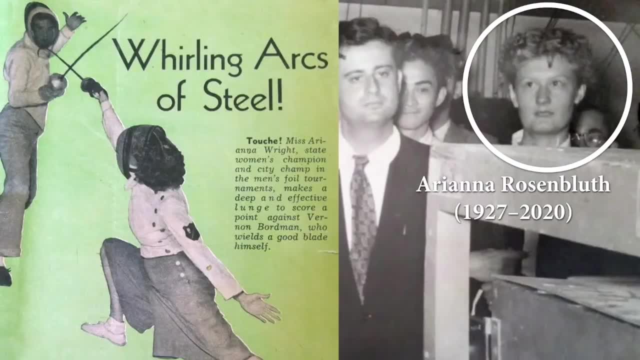 Including the first Metropolis algorithm simulation, The first scientific application of Markov chain, Monte Carlo, And a lot goes into this. Now lots of scientific computing students learn how to write these algorithms, But to invent one is a whole different business, And to make it work with the computer. 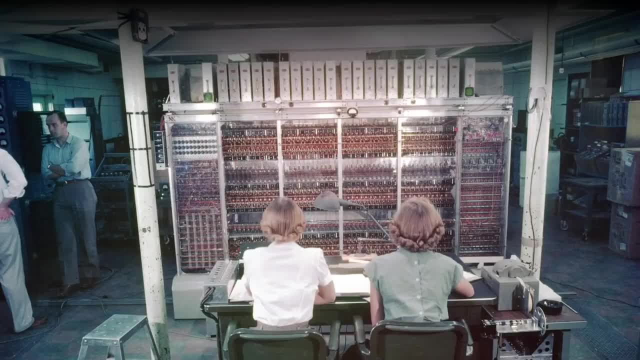 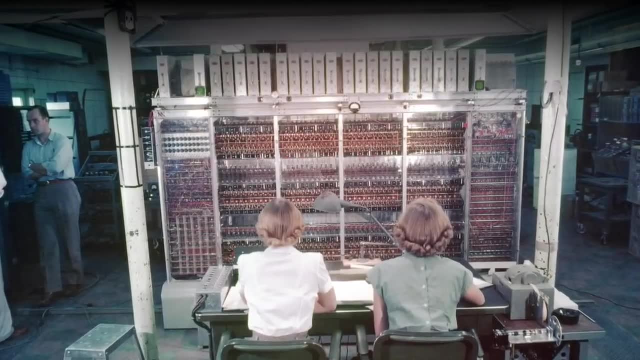 hardware at the time is indeed quite an achievement. So this is the computer that Ariana Rosenbluth had to work with. This thing was called Maniac. I'll tell you why it's called that in a moment. Maniac is a huge number. 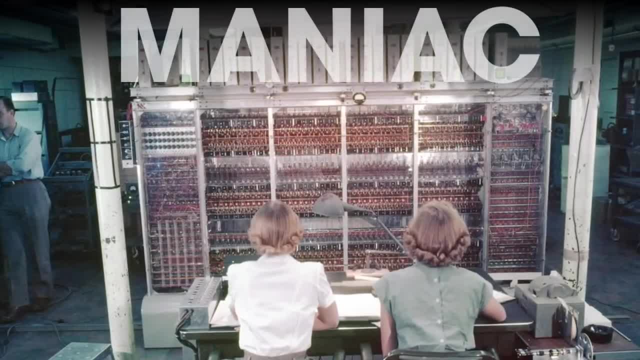 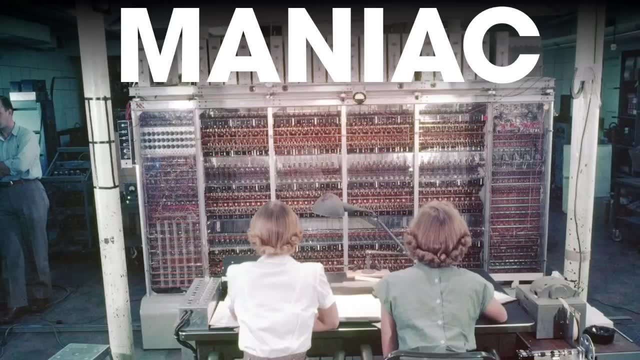 of transistors and vacuum tubes and other things And by modern standards, a very feeble computer. But at the time it was one of the most capable ones And at Los Alamos they were putting it to use for lots of different purposes. 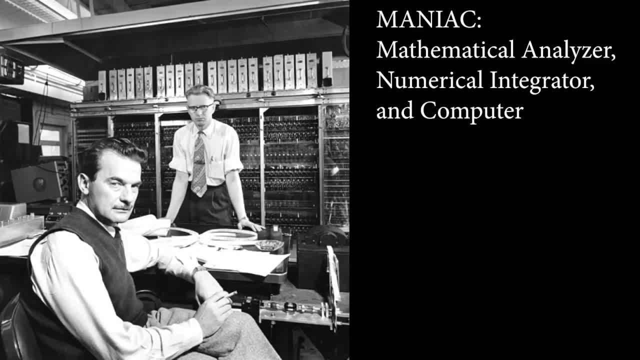 Nick Metropolis, who gave his name to the Metropolis algorithm, is pictured here in the foreground on the left smoking the cigarette, And I'm not sure if he called the computer Maniac or someone else did, But it's a bit of an inside joke. 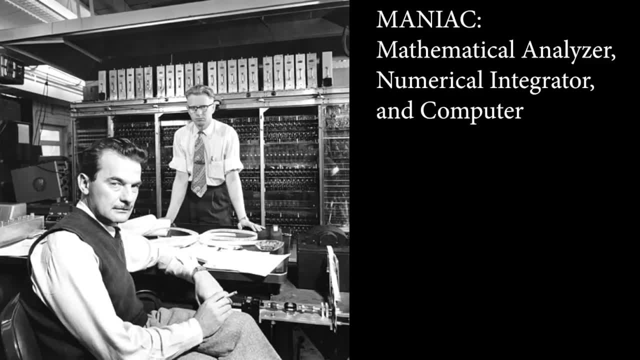 Obviously it stands for Mathematical Analyzer, Numerical Integrator and Computer, And the idea was that scientific acronyms had already become absurd at the time, And so they were playing with the game as a bit of a pun Maniac weighed a thousand pounds. 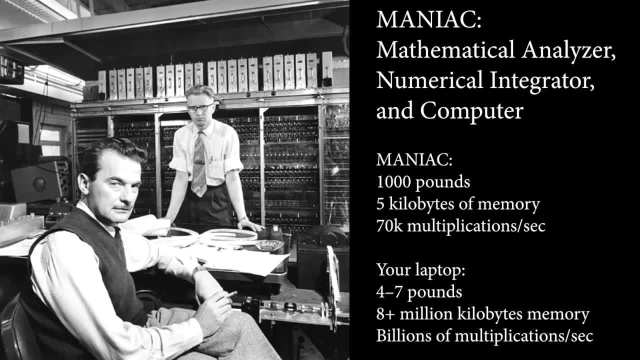 Had only five kilobytes of memory And could do seventy thousand multiplications per second. Now, five kilobytes of memory and seventy thousand multiplications per second may sound like a lot if you're a person, Because you may not have direct short term access. 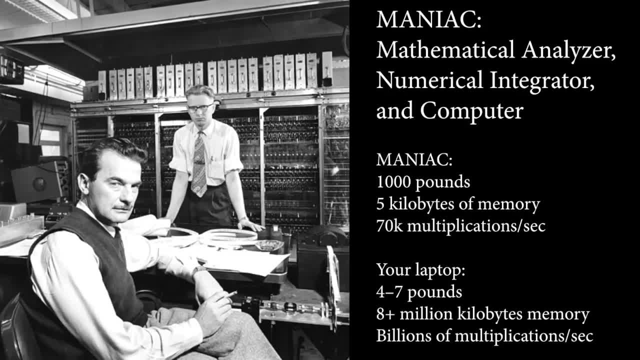 to five kilobytes of memory and seventy thousand multiplications per second is not something you could consciously do- Unconsciously perhaps, but not consciously- But in contrast, your laptop, even a cheap laptop that's five to seven years old, will only weigh four to seven pounds. 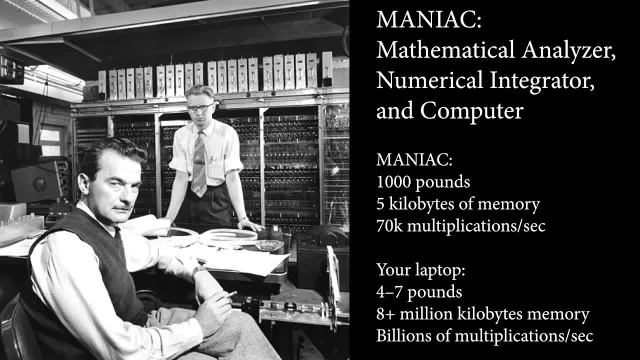 have more than eight million kilobytes of memory and be capable of billions of multiplications per second. Maniac was capable at the time, but it was very difficult. hardware to program in Memory was cramped, The operations were limited And most of the programming tools 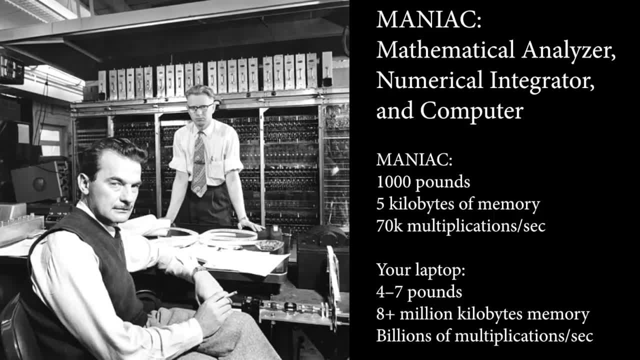 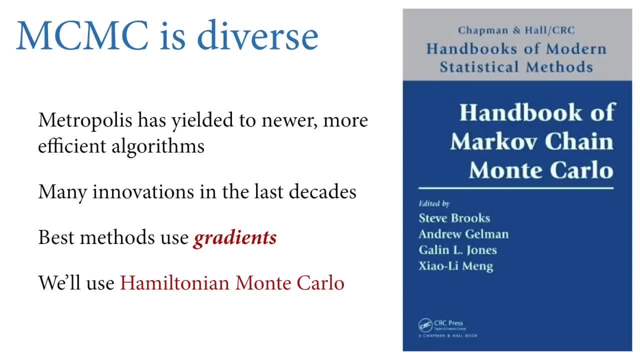 we take for granted now high level languages compilers, debuggers- simply didn't exist, So Arianna Rosenbluth had a really incredible task here. Before I talk about the details of these algorithms, or rather show you heuristically how they function, I want to give you an idea about 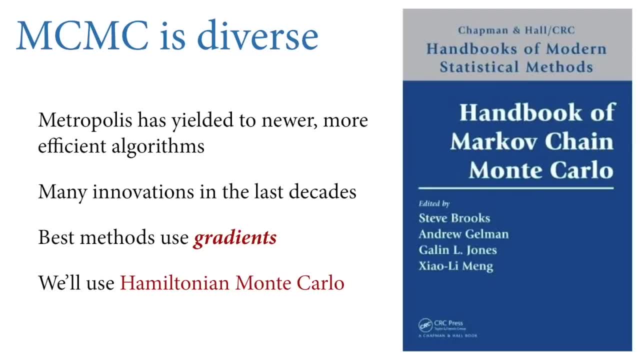 how big this topic is now. Mark of Chain, Monte Carlo is a huge field and there are people that spend their whole careers just working on these algorithms: inventing new ones, inventing diagnostics for them, finding new ways to make them efficient, And so the sort of plain Metropolis algorithm. 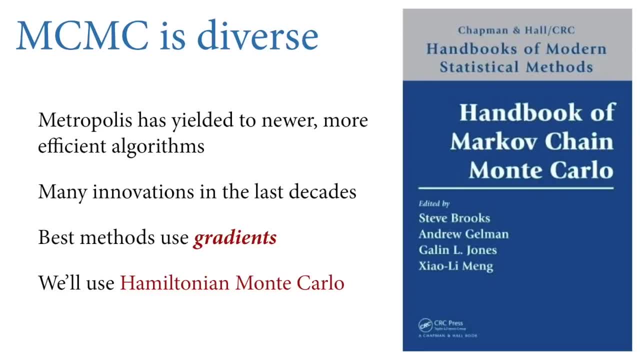 that Rosenbluth invented, or rather found a computerized algorithm for mathematicians came up with the basic strategy, isn't of much use anymore because we have much more efficient algorithms to use. But that's not to disrespect it at all, because without the Metropolis algorithm 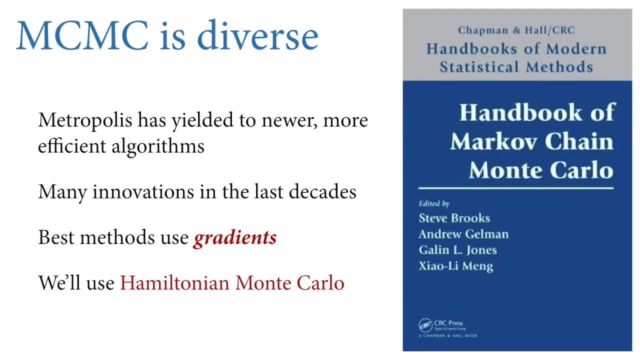 or maybe we should call it the Rosenbluth algorithm. we wouldn't have the new ones either. There have been a lot of innovations, especially in the last two decades, and all of the new best methods for Mark of Chain, Monte Carlo, use gradients, Gradients. I'll say more about this later. 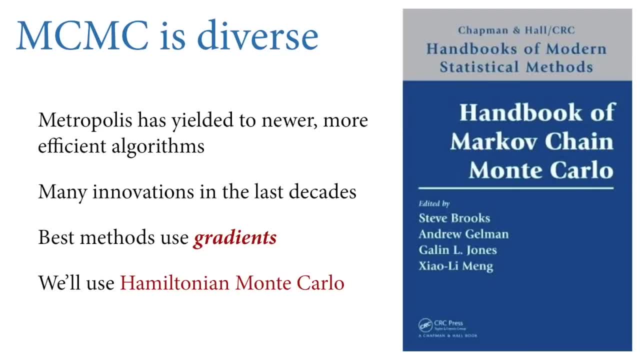 but the gradient has to do with the curvature of the distribution you're sampling from the local curvature at each point. I'll say why that helps as we go forward. The gradient method we're going to talk about and use in this course is called Hamiltonian Monte Carlo. 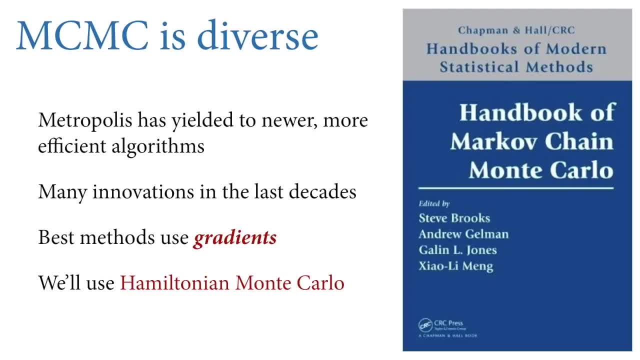 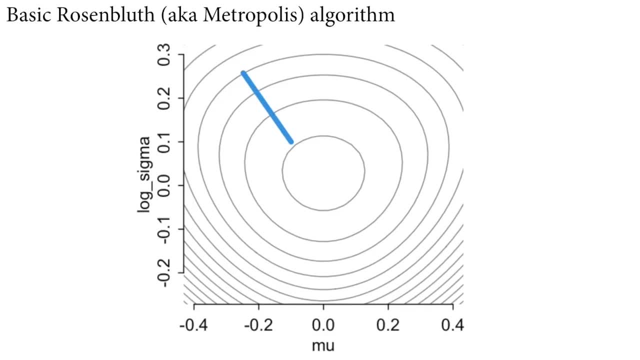 And the Hamiltonian is a term from physics that has to do with the energy in a system, And it has to do. I'll say why in a bit, but let's still talk about the Rosenbluth algorithm, usually known as the Metropolis algorithm. 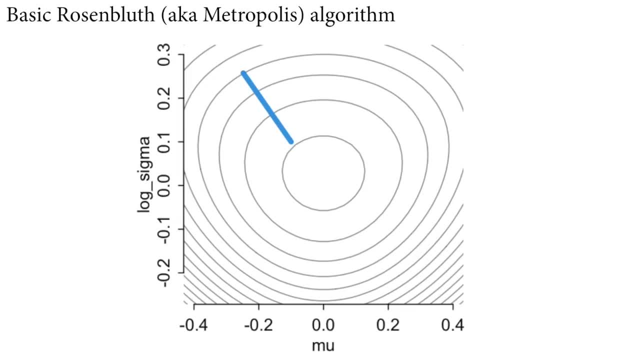 The way it works, as you saw with King Markov, was to make propositions and then consider that proposal in relation to your current position, So in continuous space. how does that work? And I'm showing you on this slide is a typical normal distribution estimation problem. 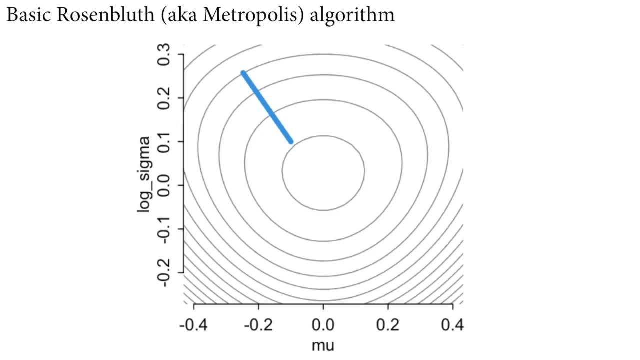 where we've got the mean of a normal distribution on the horizontal axis and the standard deviation sigma on the vertical. But we're showing the logarithm of the standard deviation so that it's continuous. So there's no boundary at zero, So the negative numbers are below one. 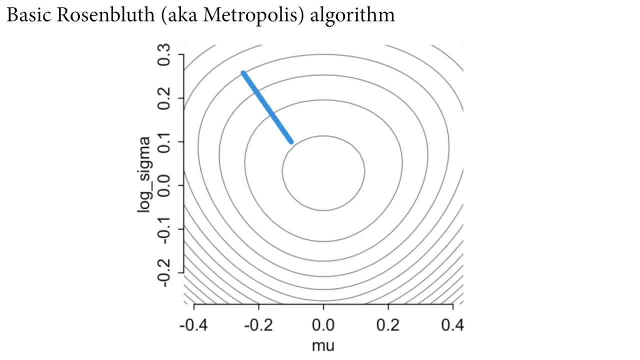 If you exponentiated them, they'd be above zero. So what you're seeing with the blue, I should say the rings on this slide represent the shape of the posterior distribution that we want to draw samples from. If we knew it, it would have this shape. 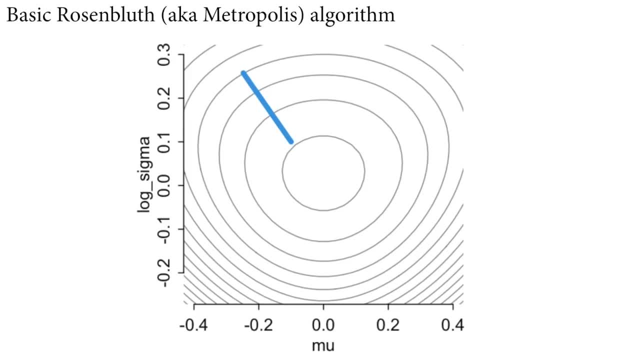 it would look like a hill, or rather, I want you to think of this thing as a bowl, where in the center of this slide is the region of highest posterior probability, and that's down in a valley. Things tend to sink into it And then, as you move towards the edge, 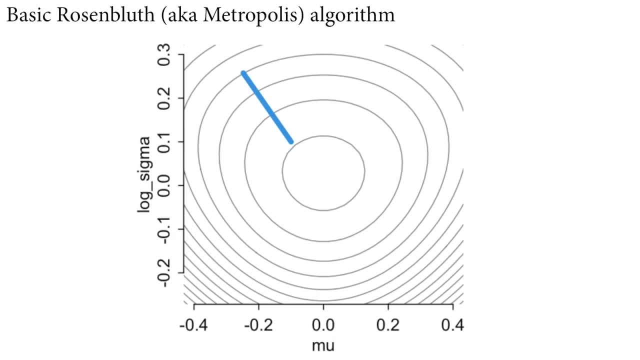 and the contour lines get closer together. those are ridges that are rising up and those are regions of very low posterior probability And we don't want to visit those places very often because they're like islands with small population sizes And the blue line you see there. 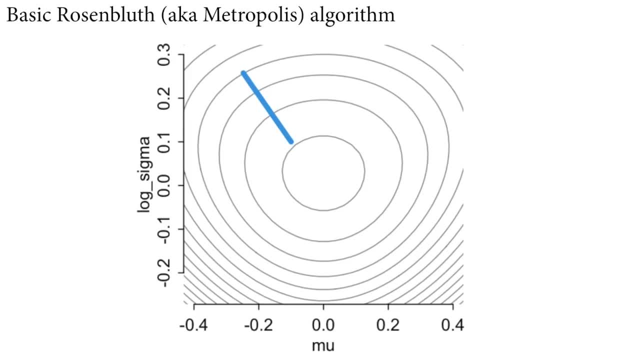 is the first proposal And this chain is going to animate and what you'll see is that if there's a red dot, that's a rejected move through the randomization device and otherwise it will move and there'll be a new black dot, And then those points are the samples that we collect. 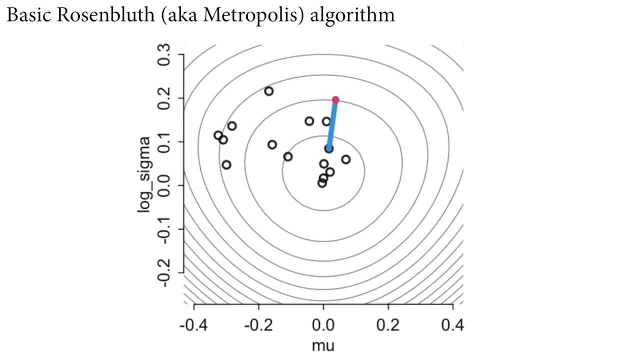 And if we pile up all those samples, we get the posterior distribution. If we get enough of them, we get an approximation of the posterior distribution. So you can see, this thing about these algorithms is that they only act locally. They don't know the posterior distribution. 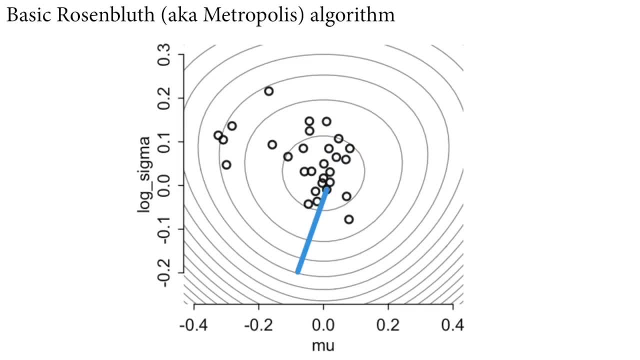 That's why we need these methods, because we don't know the posterior distribution. We can't sample from it directly, But we can blindly stumble around it miraculously and draw proper samples from it. And that's what these Markov Chain- Monte Carlo algorithms allow us to do. 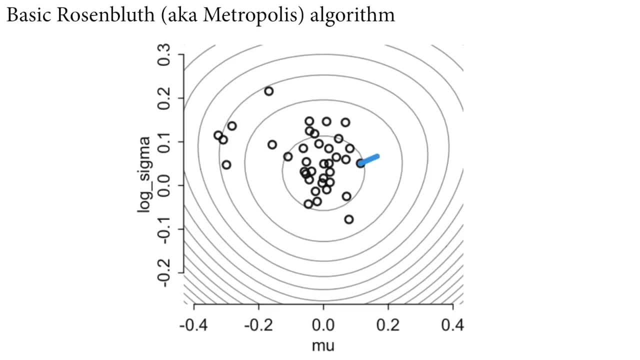 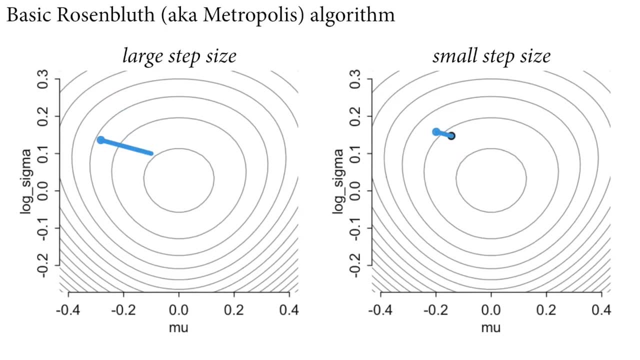 And they're often a most efficient solution for directly sampling from arbitrary probability densities. One of the things about the Rosenbluth algorithm that is frustrating is that it has to be tuned So the size of the proposal. that is, how far from your current location? 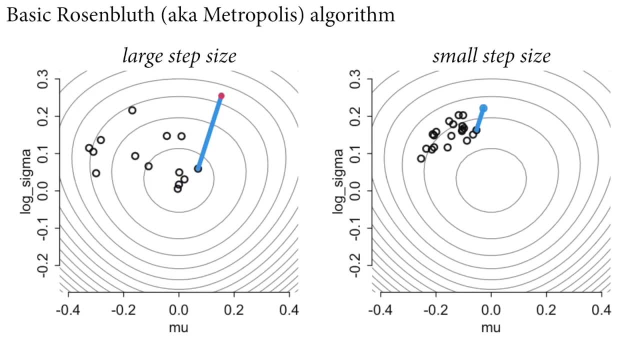 you consider, moving has a big effect on how efficient the algorithm is And basically you lose at one extreme or the other. So you have to tune these things in general applications. So on the left I'm showing you the animation from the previous slide, what I'm calling the large step size. 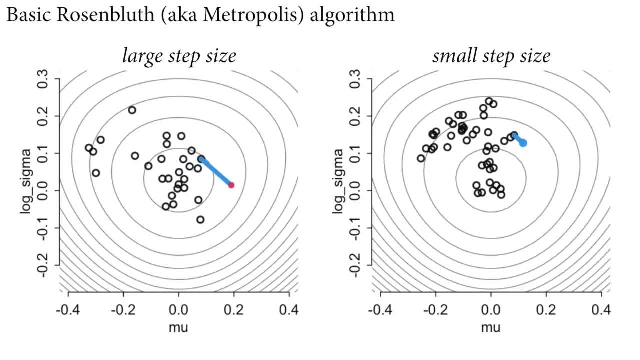 version of the simulation, You'll see that the blue bar is often quite large. This simulation is willing to consider points very far from the current location. As a consequence, lots of them are red, meaning that they're rejected, And then the changes stay still. 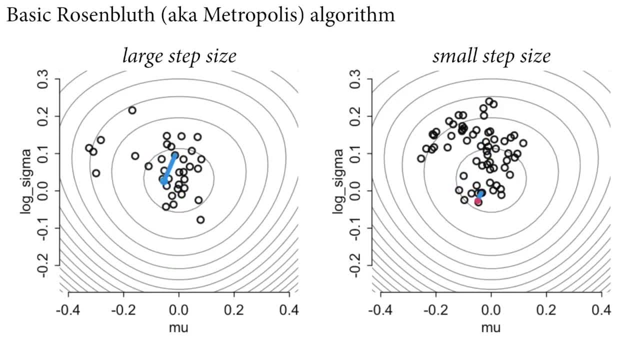 for many steps at a time, as it is right there, And that wastes a lot of computation. What you'd really like is for every proposal to be accepted, to always propose points that are valid in the posterior distribution and to always move there, But that's not possible with this algorithm. 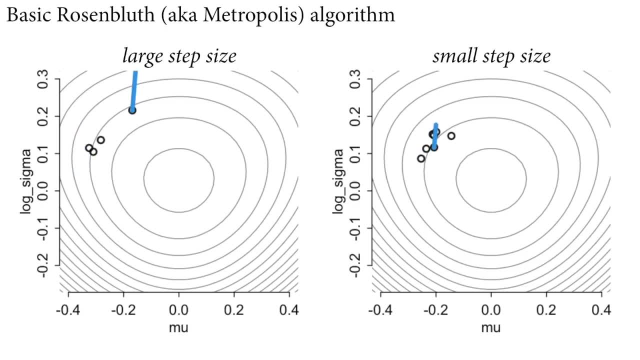 On the right you've got the other extreme, small step sizes, only considering very local proposals. This is like King Markov's algorithm where he only considered neighboring islands. When you do it this way, you only very rarely reject, or much more rarely reject moving. It still happens. 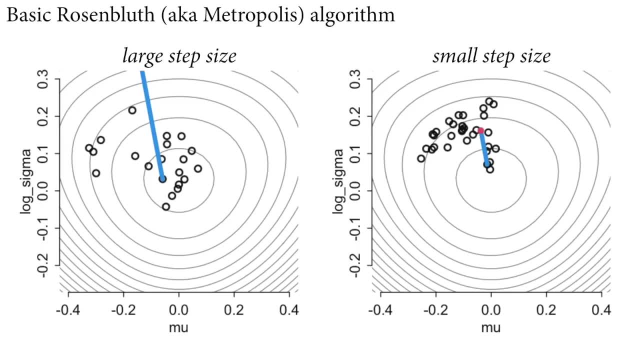 So you take more samples, but the samples are really close to one another and, as a consequence, each additional sample doesn't add a lot of information about the shape of the distribution. In contrast, on the left, when you do manage to move, you learn a lot more. 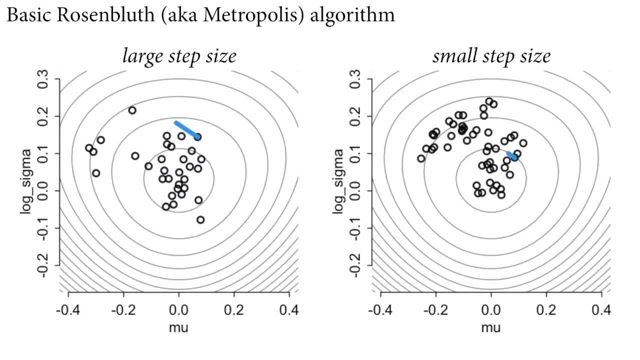 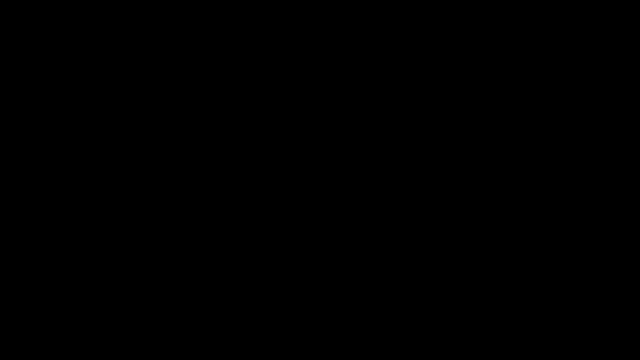 because the points are less similar to one another after a move. So all computational methods have trade-offs like that, So there's nothing special about that. But it turns out we can do a lot better, And that's what these modern gradient methods do. 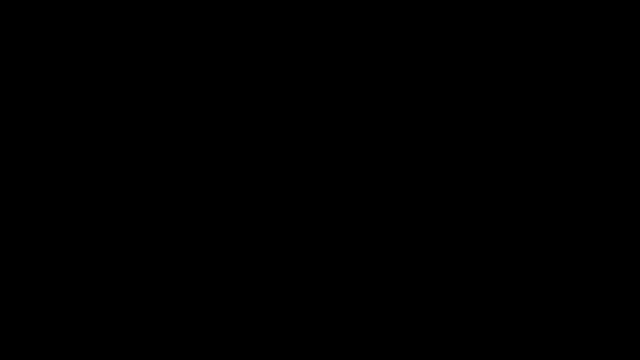 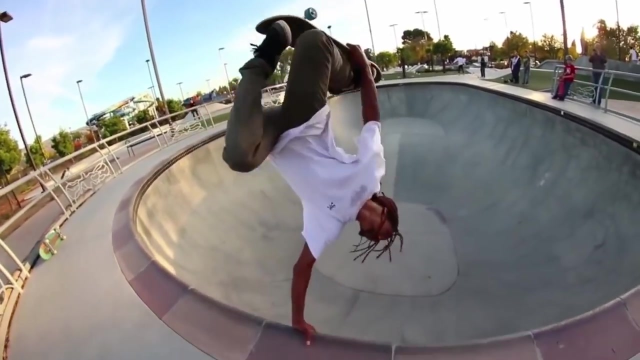 So let's consider an analogy. before I show you what Hamiltonian Monte Carlo looks like, I want you to think about skateboarding and skate parks. So here, like this bowl, is what I would call this a big bowl, And the very talented young man. 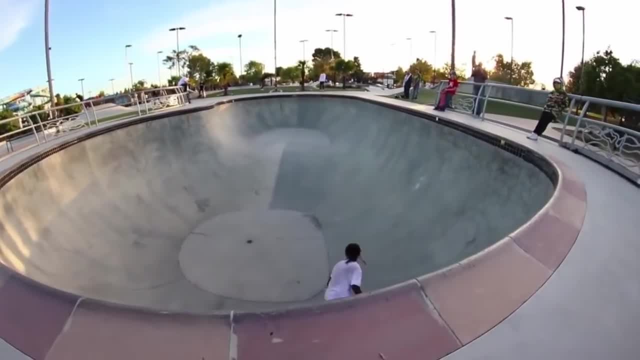 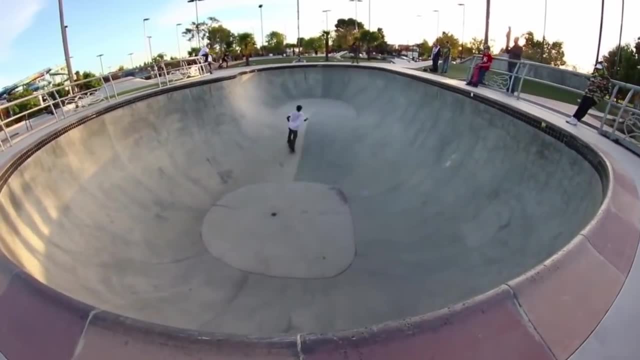 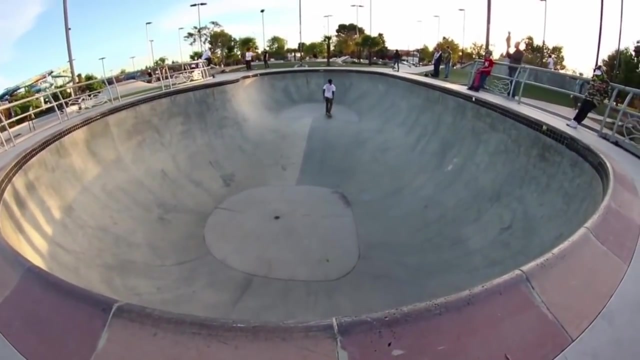 there who is skating. there's a sense in which, of course, his skateboard doesn't know anything about the shape of that bowl And yet it rolls effortlessly around it. And because the potential energy as he rolls around this thing is highest on the edges, it will naturally turn him around. 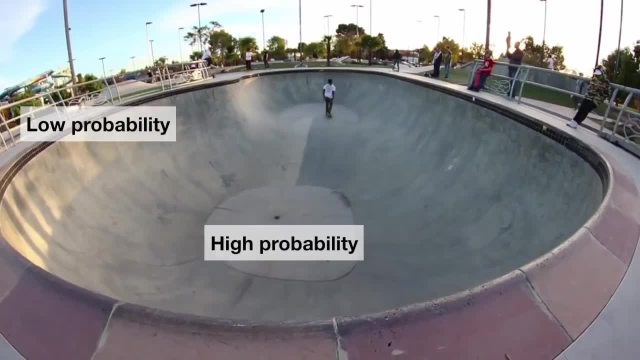 under the force of gravity, and he will tend to spend more time near the bottom, And so this is like the high probability region of a posterior distribution, Whereas the edge is the low probability region because he can't stay there as a moving skateboardist, as it were. 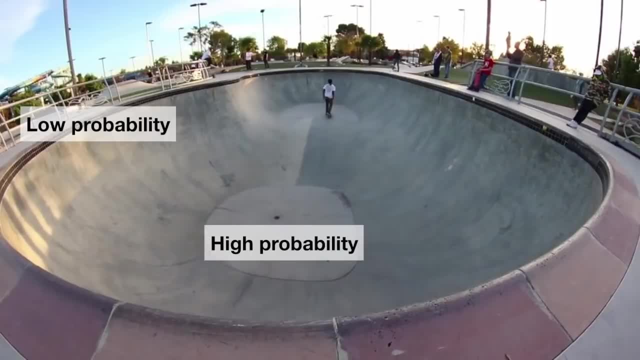 So what if we could use a strategy like this to sample from arbitrary distributions. represent them like bowls. they don't have to be perfectly Gaussian bowls, they can have odd shapes, like the one you see on your slide. And then we put virtual skateboarders to thrash around in there. 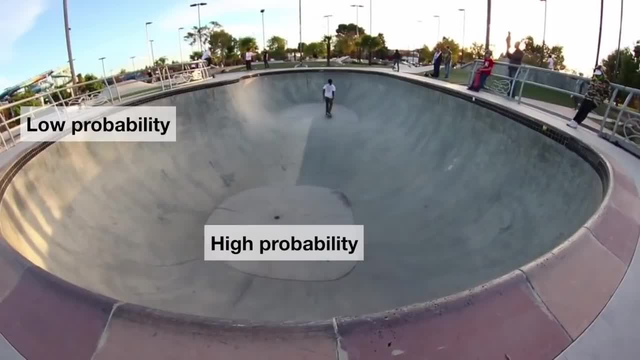 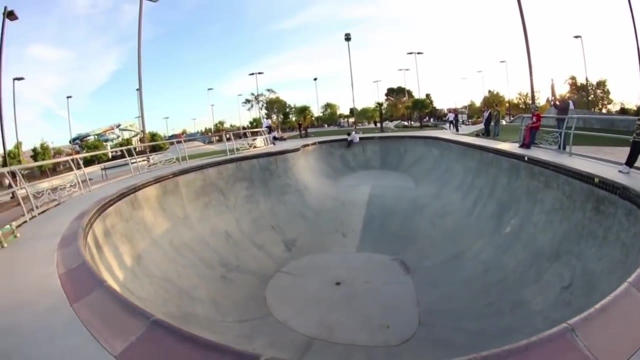 We flick them through the bowl and let them do a couple tricks and as we track their positions, their positions over time will tend to take samples from the shape of this bowl, because they spend more time near the bottom than near the top, And it turns out you can do this. 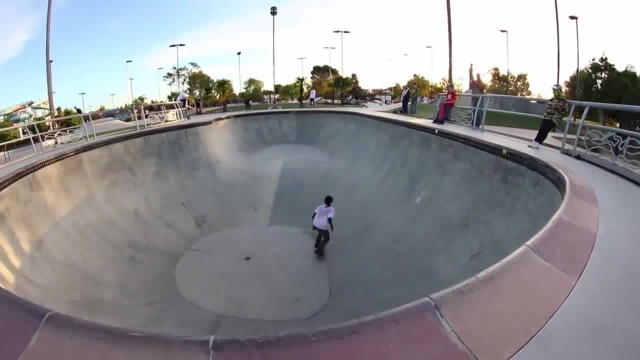 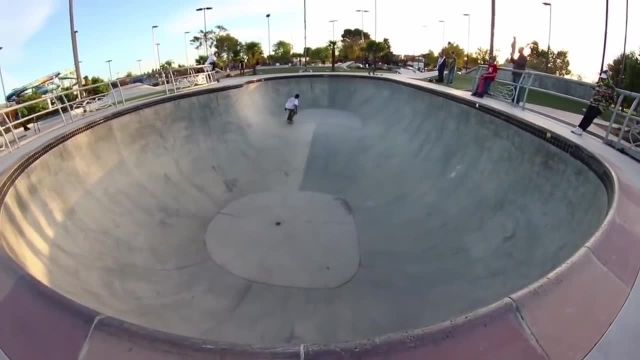 and this is what the algorithms I'm going to show you next actually do. And it seems weird that we can do this, but we really are. We're going to run skateboard simulations, or frictionless skateboarder simulations, inside the computer so we can take samples. 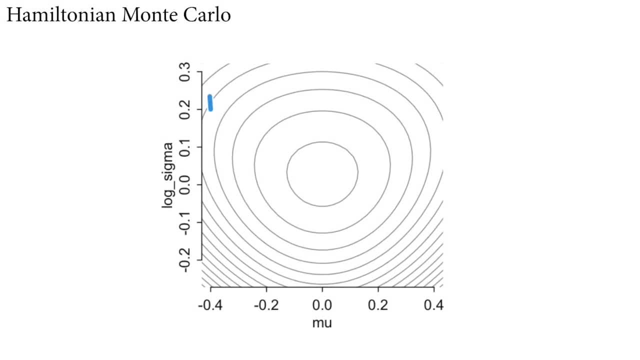 Okay, how does this actually end up looking? Now I've got my virtual skateboardist lined up on the edge of the bowl. there there's that little blue tick, he's about to start rolling, and it's the same Gaussian posterior problem as I had before. 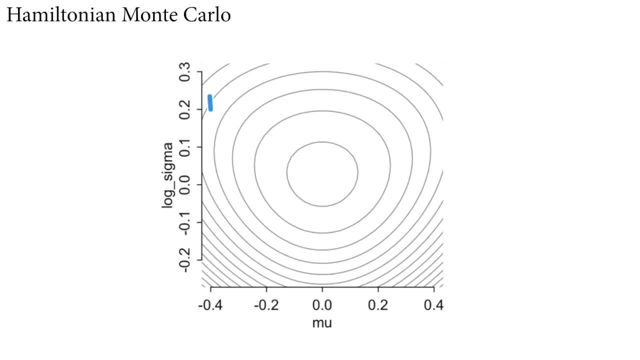 with the mean of a normal distribution that's estimated on the horizontal and it's log standard deviation on the vertical. Now what's going to happen here, remember, is the middle of this contour, is the center of the bowl, it's the bottom and then out on the edges. 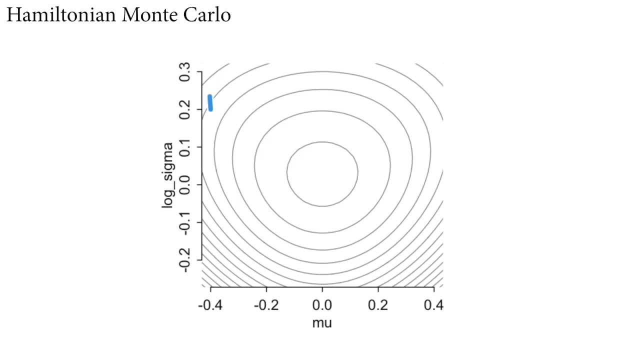 we've got the ridges, the edge of this thing, and so we're just going to start a physics simulation, literally, and it's going to be a frictionless skateboard and it's going to roll. we're going to flick it with momentum in a particular direction, a random direction, in fact. 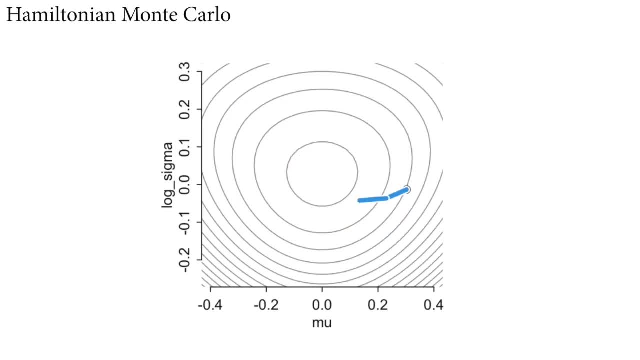 and we're going to let it run for a little while, as you see here, and it follows the contour and rolls back down, and then we stop it after some particular length of path and we record the position and that's what those black dots are, and then we flick the skateboarder again. 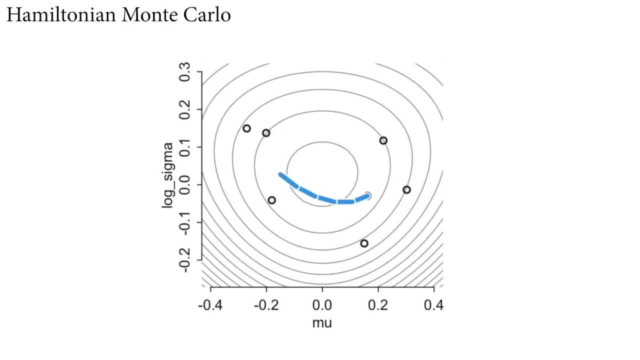 in a random direction and we let the physics simulation go, turns around, record the position, and every one of these trajectories- they're called- results in a sample from the posterior distribution. now you have to be careful exactly how you do these calculations so that it's a proper Markov chain. 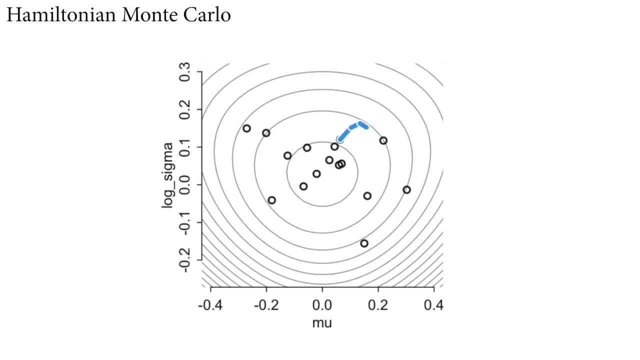 but it's not that complicated to do it and the mathematicians have figured out the details for us to make it work. this is a fantastically very useful sort of thing, but it requires the gradients, as I said. the additional thing you need to know here is the local curvature. 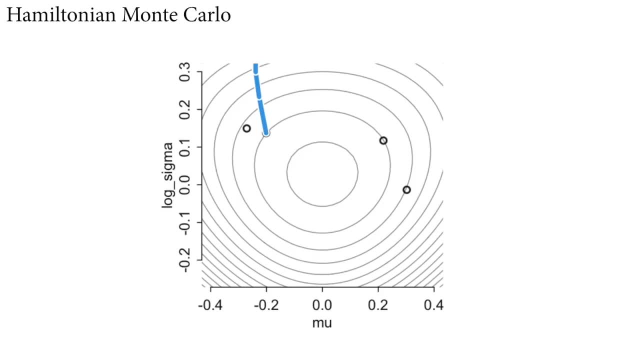 that is, you need to know what the skateboard knows, you need to know whether you're going uphill or downhill in any particular local position so that you can run the simulation, because this is not a metaphor, that I'm running a physics simulation here. this really is a physics simulation. 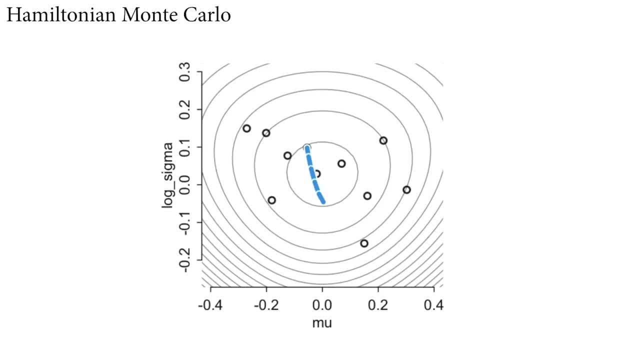 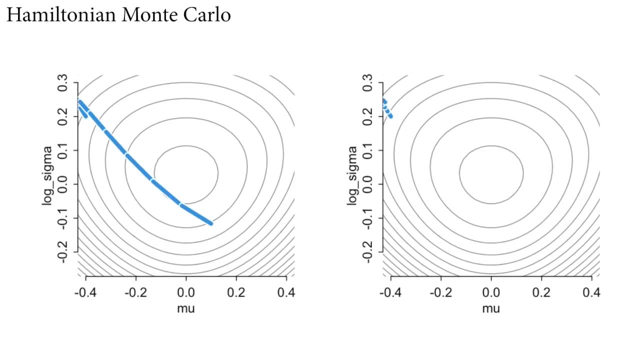 a little frictionless particle rolling around on the posterior distribution and the samples just come from its position at fixed points in time. so these methods also require some tuning and you can have really long trajectories, like on the left, and let the skateboard roll for a long time. 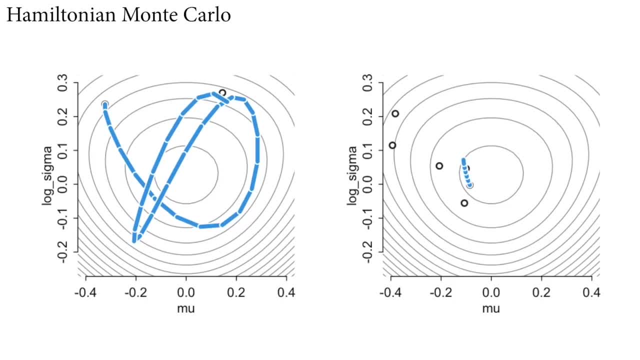 and since it's frictionless, it'll roll forever. actually, they'll never stop. this is not always the most efficient thing to do, because often it'll loop back and you get this phenomenon I talk about more in the book called the U-turn phenomenon, where the trajectory turns around. 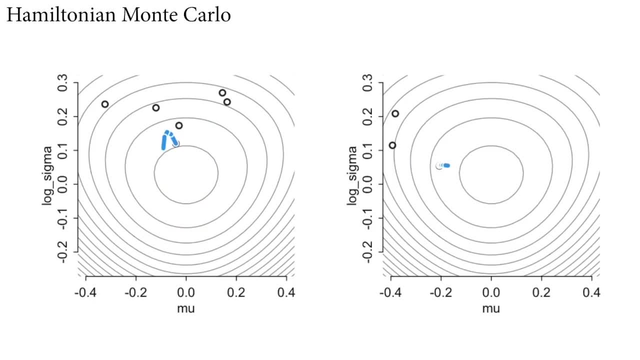 and so you end up with samples that are really similar to one another, because they end up next to one another, as you see on the left, and that's not optimal now. in the long run it'll be fine and you will take valid samples from the posterior distribution. 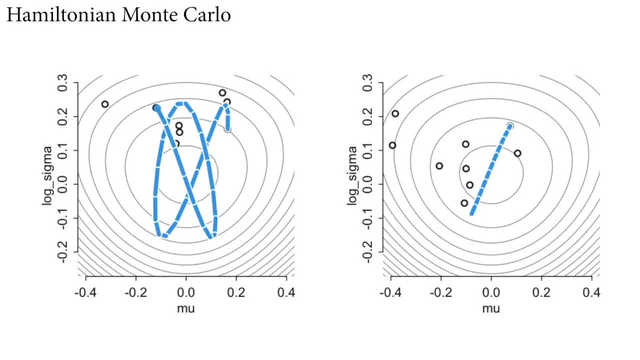 and explore it. it's just less efficient. on the other extreme, we have really short steps. you see the little increments in the blue worm there. that's called step size. and when the trajectories are short and have small steps, exploration is slower but in a few jumps. 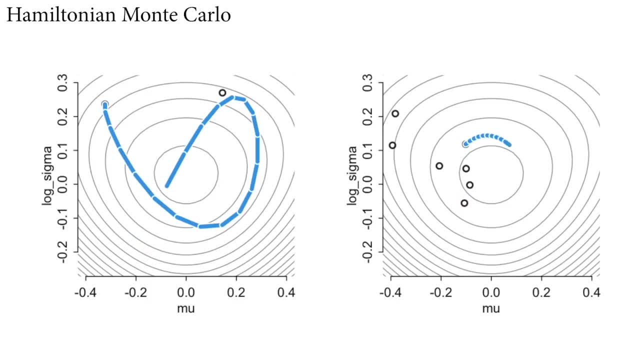 you can still traverse the whole shape of the thing and get valid samples. it just may take longer to explore the whole shape of the distribution. modern engines, as I'll talk about in a little bit, figure out these parameters for you. they have an adaptation algorithm in them. 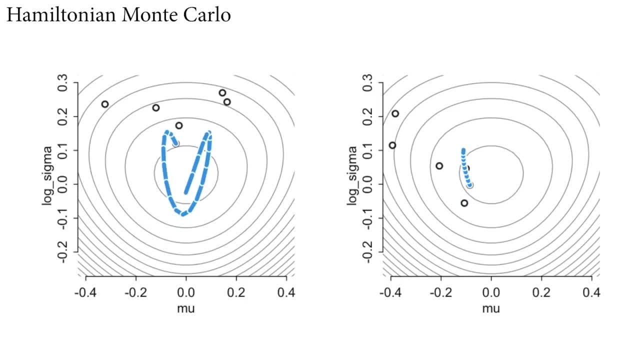 to try and figure out the right step size and length of trajectory, that is, how fast and how long the skateboarder should go, so that you can efficiently explore the posterior distribution. now, of course, the distribution on this slide is not hard to sample from and the basic Rosenbluth 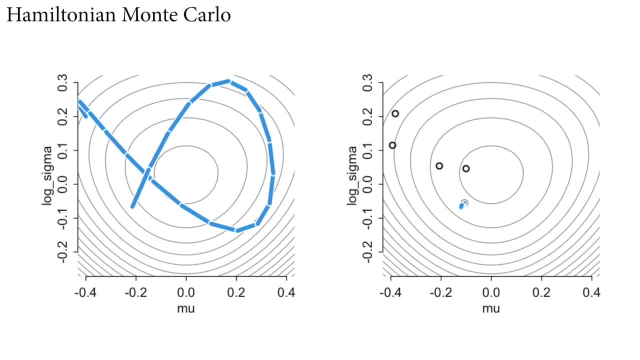 or Metropolis algorithm will have no problem sampling from it either. it's a bit of overkill, although it's fun to watch. where Hamiltonian Monte Carlo really shines and becomes essential is in more complicated posterior distributions with many dimensions. and the thing about more complicated posterior distributions: 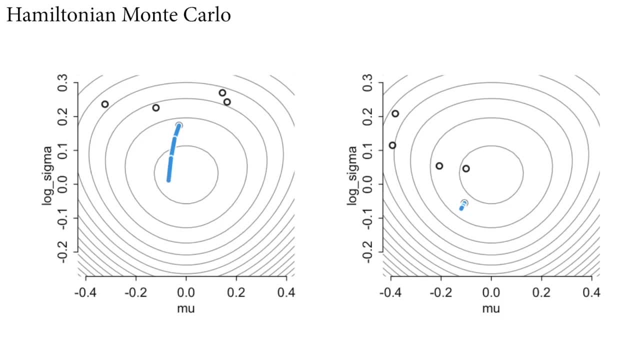 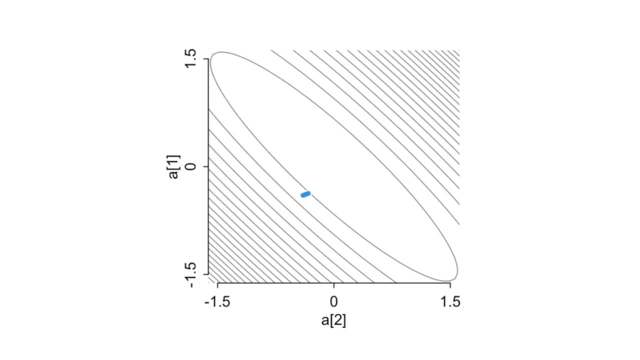 which arise even in modestly more complicated models than the ones we've used so far in the course is that they often have very high correlations in them between the parameters. so let me show you an example of that. this is still only a two-dimensional example, because who can see 3D or 4D on a slide? 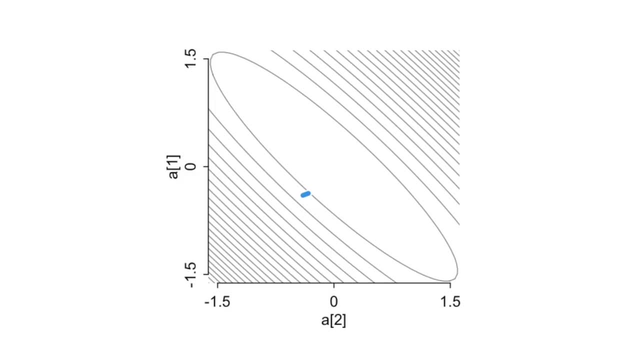 so we'll stare at this and even though it's only two-dimensionals, imagine it's very high-dimensional and these correlations exist between a bunch of parameters simultaneously. what your Markov chain sampler has to do is move along some hyper-dimensional thin ridge like the oval on this. 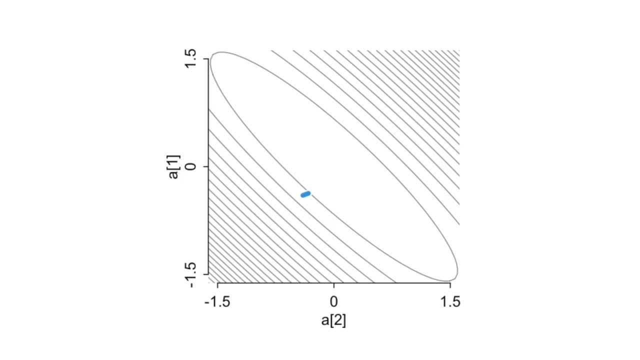 on your screen here. this shows again the contours of the posterior distribution, and the oval in the center is the high probability region. that's where we want to spend our time, that's where the skateboarder will spend his time, and the more closely packed ridges are the low probability regions. 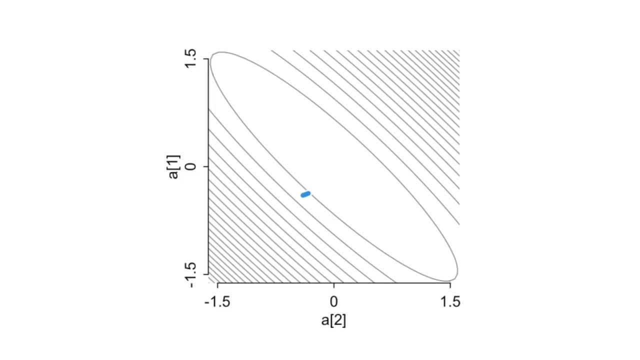 where gravity forces you back towards the middle and we can. Metropolis has a really hard time with distributions like this, because it tends to. since this is such a narrow shape in the middle, Metropolis will tend to make proposals in the bad part, outside the ridges. 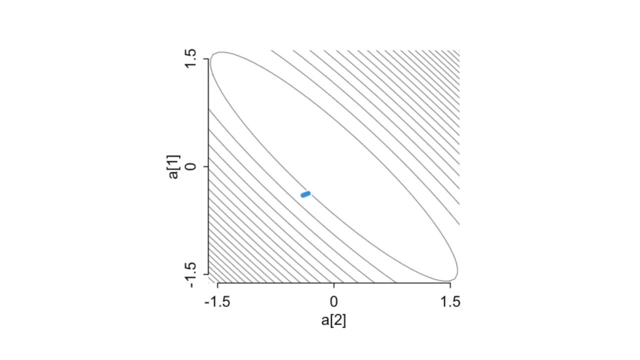 and almost all of them will be rejected, and so it's hard for Metropolis to move around a space like this because it doesn't know anything about the global shape. the thing about the skateboard that is really cool is that, even though the skateboard doesn't know anything, 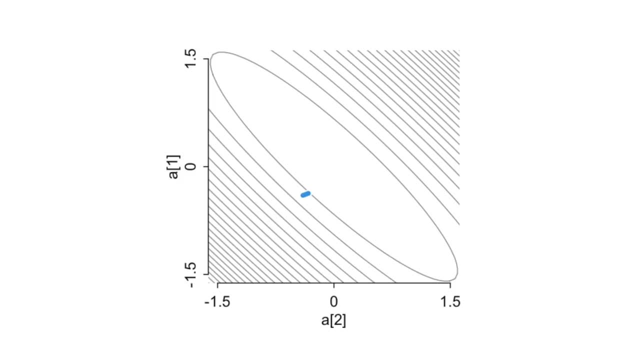 about the global shape either. the fact that it senses the curvature where it is, it knows which direction to roll, means it effectively explores the global shape quite efficiently, that is, it won't roll uphill. so let me show you what that looks like in animation. here's our skateboarder. 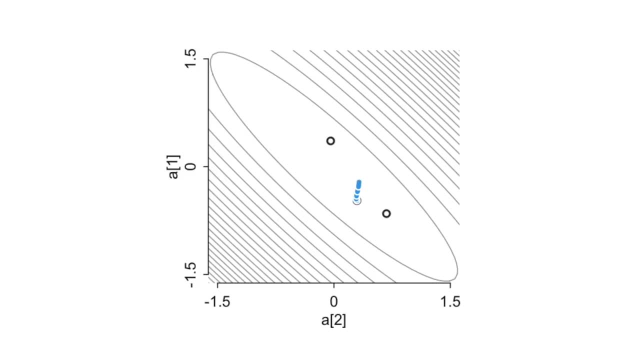 we started him on the edge. now he rolls around in the middle and takes some samples and you'll see that, even though at any point in time the simulation only knows the local curvature, it's not calculating the whole posterior distribution. it doesn't know it. it has to get that from the samples. 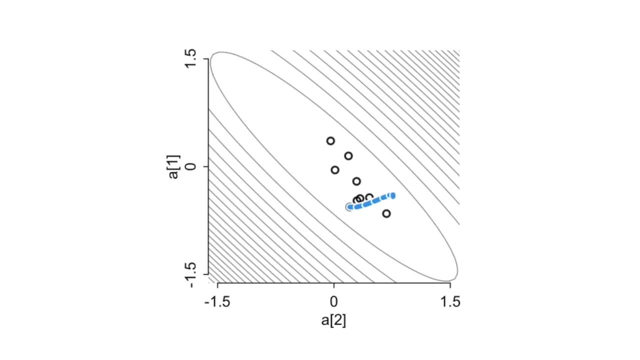 it still manages to find the shape of the oval in the middle of the slide and take samples from it and make these zig-zaggy snake patterns and all the algorithms. there are other algorithms that also use gradients and they can be as efficient as Hamiltonian Monte Carlo. 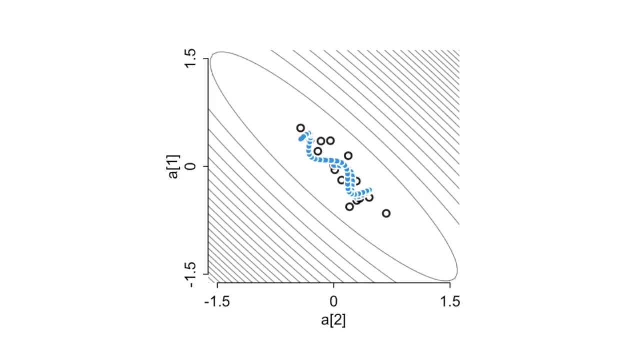 and that's because what they all share is this ability to sort of find the global curvature by considering local curvature is eventually find global curvature by considering local curvature. they're not magic and so, yes, with enough samples, as you see here, you can get the whole shape pretty rapidly. 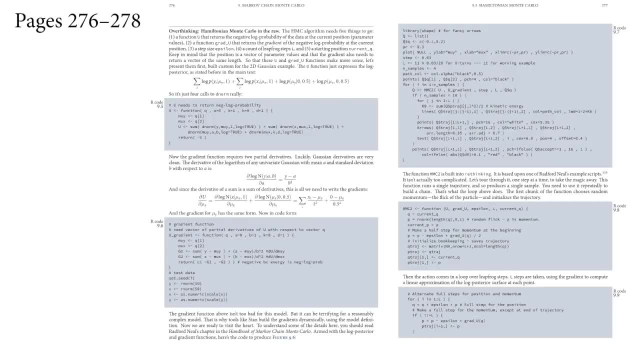 okay, that's Hamiltonian Monte Carlo. if you're interested in the actual details of the algorithm, you want to see what it looks like in code. on pages 276 to 278 of my book I show you how to do this. with basic R scripting you can write the simulations. 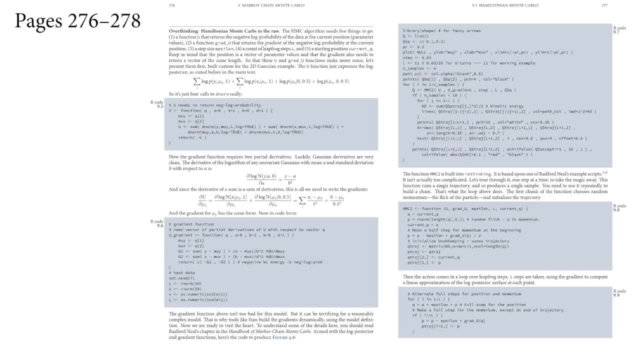 I just showed you with basic R scripting it's not that complicated and I take you through all the justifications for the different parts. and the key thing about this, the- the physics simulation part is actually pretty easy. it's just a loop that calculates velocities and updates the position of a particle. 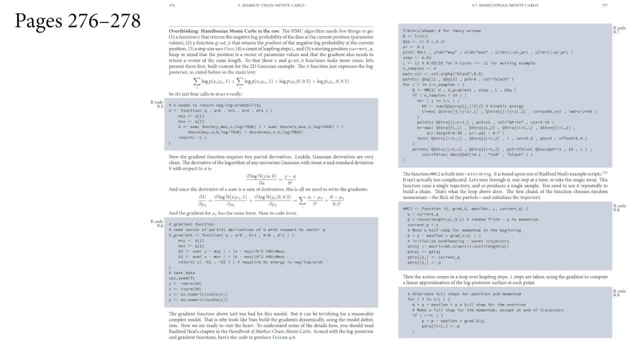 it's not. maybe off the top of your head, you wouldn't know how to write that, but once you've seen it you'll agree. it's just a little loop with some updates of positions. the tricky part is that for every model you write and want to analyze this way, 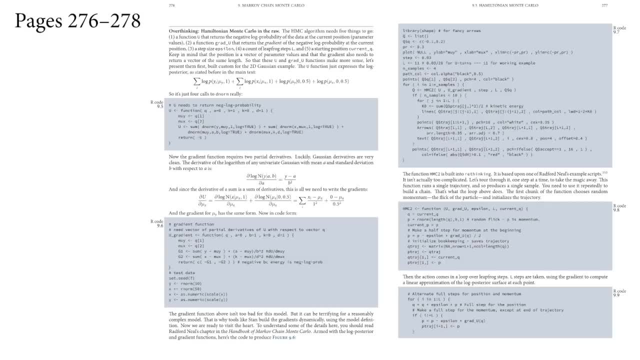 you have to calculate the gradient somehow. you need the derivative for every parameter of the log, and for big models that means a lot of derivatives and it means a lot of calculations and a lot of custom programming for every problem. we're not going to have to do that. 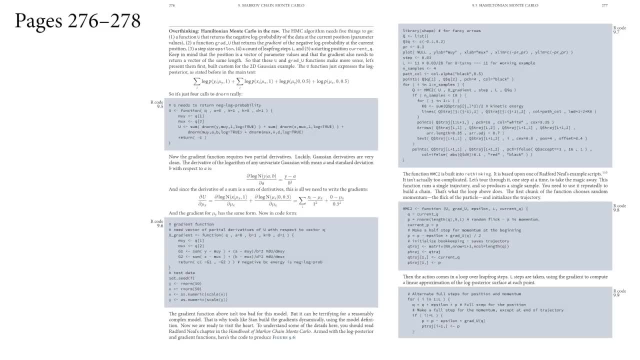 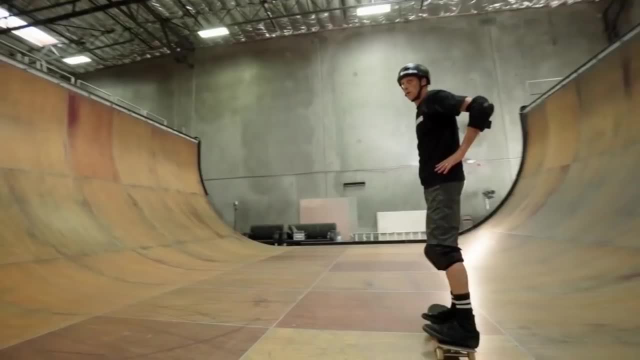 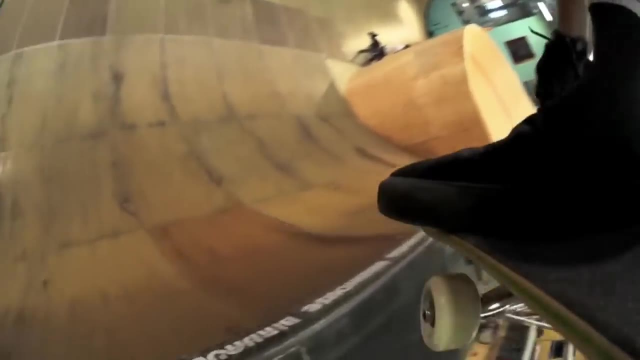 but if you're interested in that, I explain more on these three pages in the book. okay. so gradients: yes, we keep talking about gradients and we need them. here's another video to give an impression to you about how the gradient governs the motion. here's the skateboard's view. 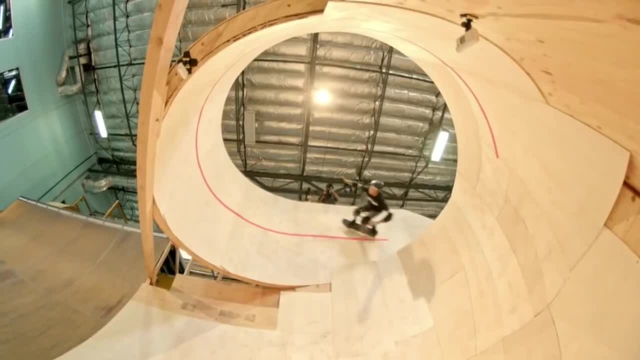 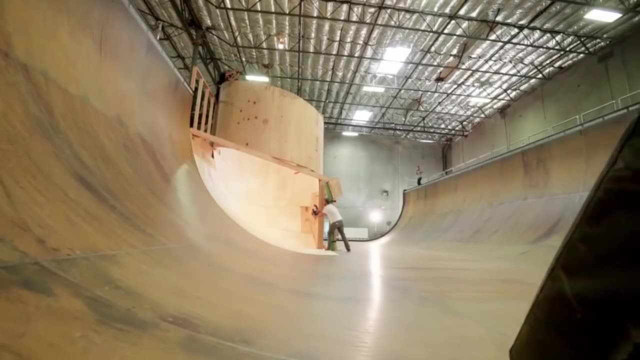 of moving along a half-pipe, a particularly deadly half-pipe, with this bizarre trap in it. the skateboard doesn't know anything about the global shape, but it can find it. all it needs at any particular point is its curvature, and so that's what we need to calculate. 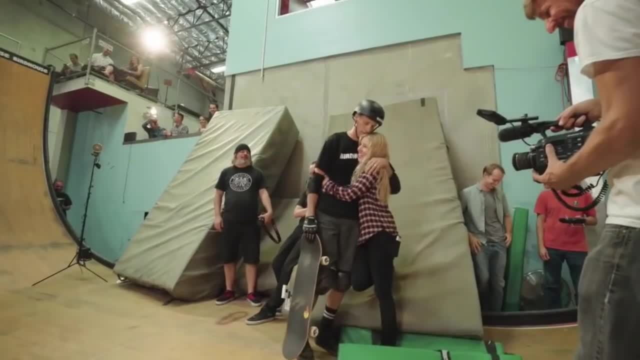 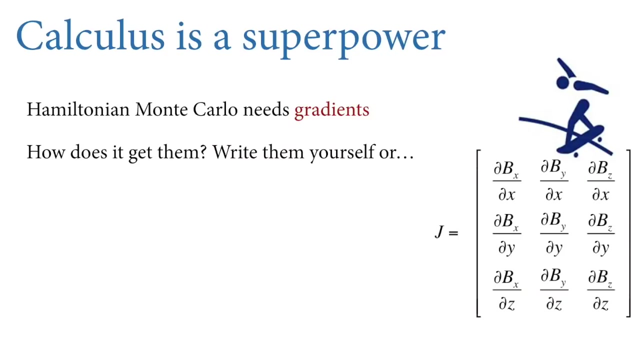 for any arbitrary half-pipe structure. so how do we do that? how do we maintain our convenience of writing general statistical models and calculate the curvature of Tony Hawk half-pipe? so we need gradients and, as I said, you can write them yourself. you could go and measure any particular half-pipe. 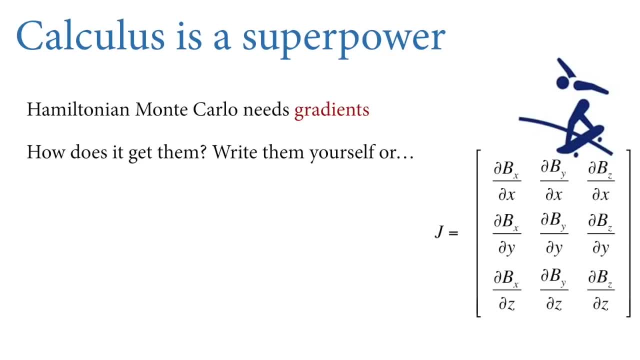 and get the curvature at every point and you could represent that knowledge with giant tables that you could look up as you do the simulation, but that's not very efficient. or you could have equations, if you can describe the shape of the posterior distribution with general equations, but that means we have to recode. 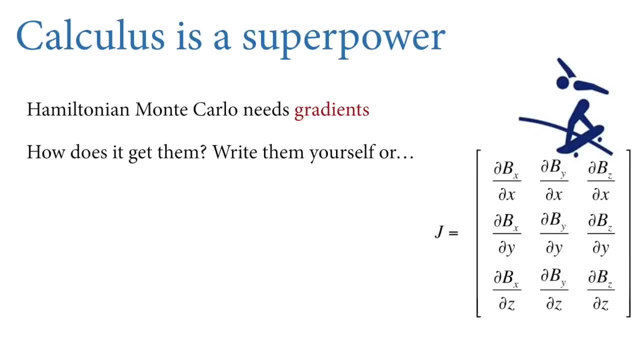 the Markov chain for every model. so you don't want to do that, you don't want to write them yourself. instead, there's this fantastic scientific computing technique called AutoDiff, which stands for automatic differentiation. and what AutoDiff does is it takes your computer code and it computes symbolic derivatives. 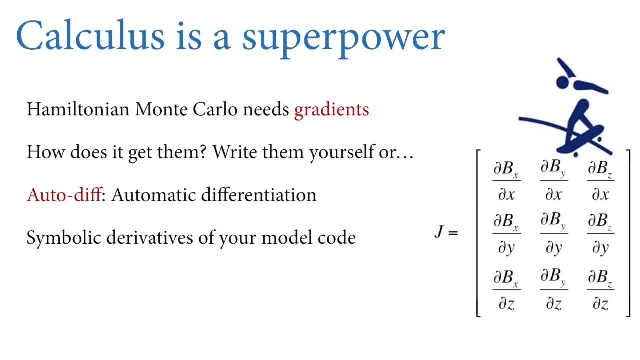 that is, the gradients from your model code. that is to say, when you write a statistical model just like the ones we've been writing in this course, at this point what you're writing is an expression, an analytical expression for the posterior probability, and that defines the distribution. 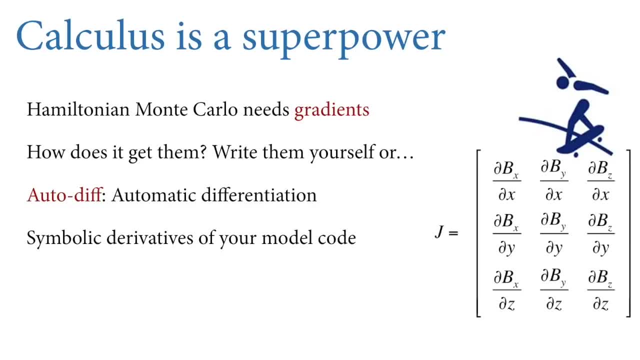 we want to sample from. that is, you can plug in fixed values for all the parameters and you can get the number, relative numbers of ways that the data could arise from that combination of parameter values. that's the posterior probability. of course we want to evaluate it, evaluate the posterior distribution. 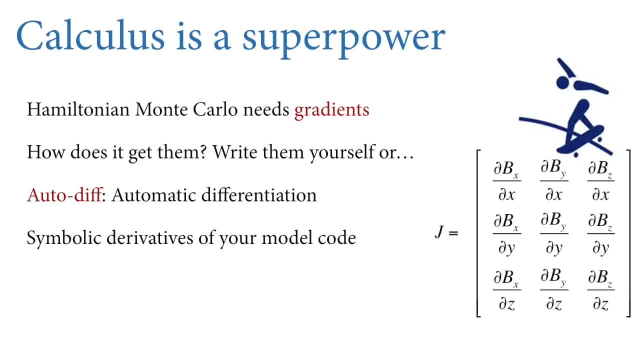 of parameter values and that's a tall order. if you had the derivatives of that expression for the posterior probability, you'd know which way was uphill and downhill from any particular combination of parameter values you had. and in mathematics when we take a set of derivatives like that from a function, 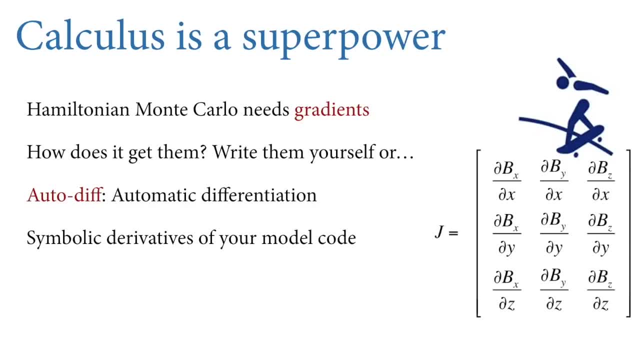 you get a matrix that's called a Jacobian, as shown on the right hand side here, and it's just a matrix of derivatives with respect to that set of variables. in our example, these would be parameters. you take the derivative with respect to that parameter and this gives you 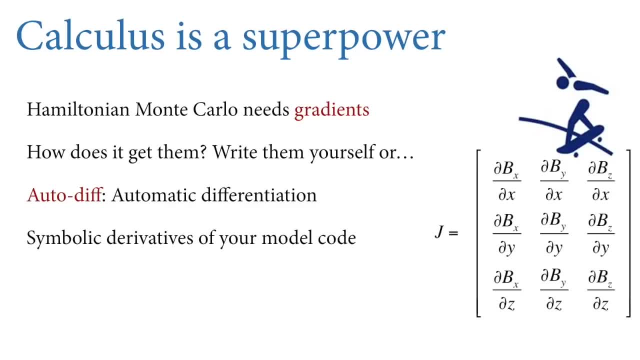 information about whether it's uphill or downhill for any particular parameter. if you increase that parameter, would the probability go up. if you decrease it, would it go down, and AutoDiff does this for you. that's why it's called automatic differentiation. it can do this because taking derivatives is. 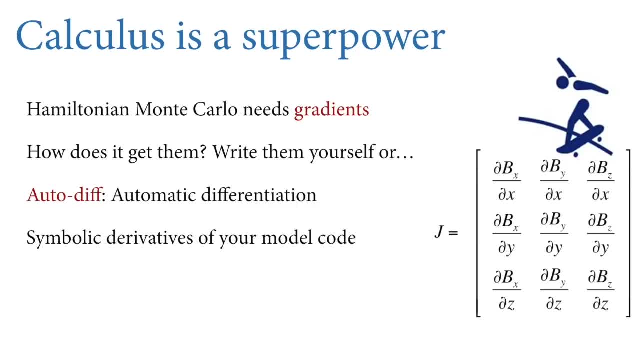 easy, there are rules for it and your computer is very good at following them. still, the computer science that goes into these algorithms is really amazing, and we're lucky that people have written them for us and we can just use the libraries that make it work. automatic differentiation is not unique. 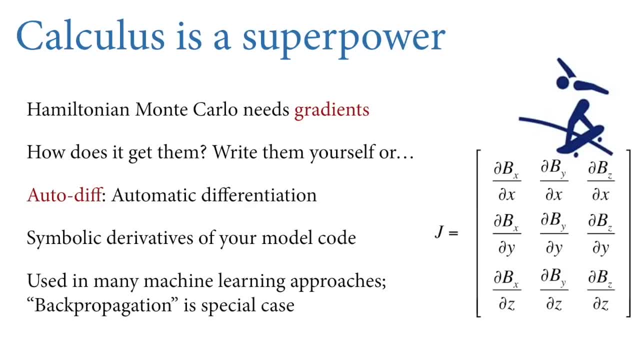 to Hamiltonian Monte Carlo or even Markov chain Monte Carlo. it's used in a lot of machine learning approaches for any kind of high dimensional machine learning that goes on these days. most of it, let's be honest, you need gradients to search the space because there's too many parameters. 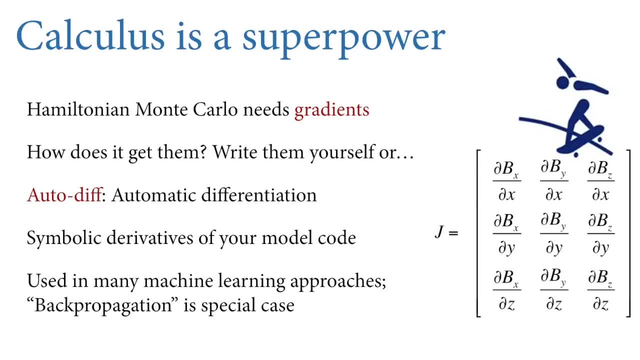 and the parameter space is just too big to do any kind of brute force thing. and so, for example, some of you will have heard of backpropagation, which is used a lot in neural networks. backpropagation is a special case of automatic differentiation. okay, as I said, 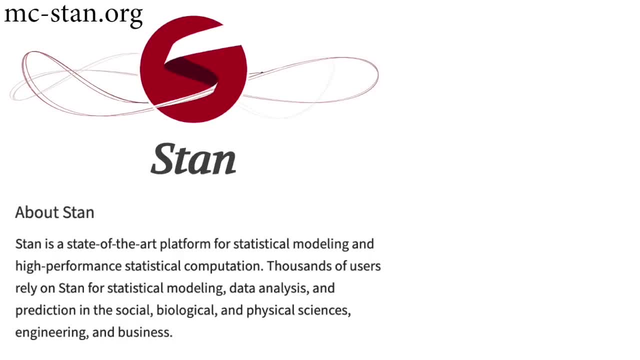 you're not going to have to do any of that yourself. that's the good news. instead, we're going to use the Stan math library to do the automatic differentiation for us. you'll be able to continue writing the model definitions as you have been so far, and Stan will compute the gradients for you. 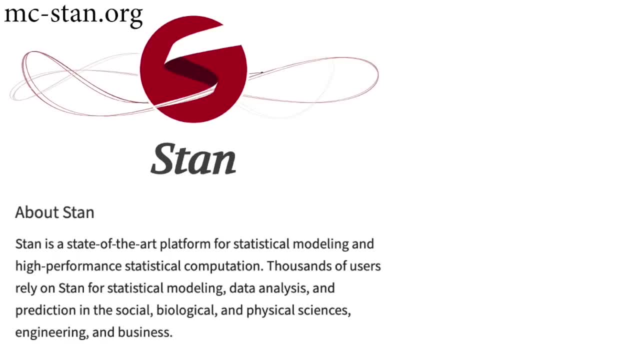 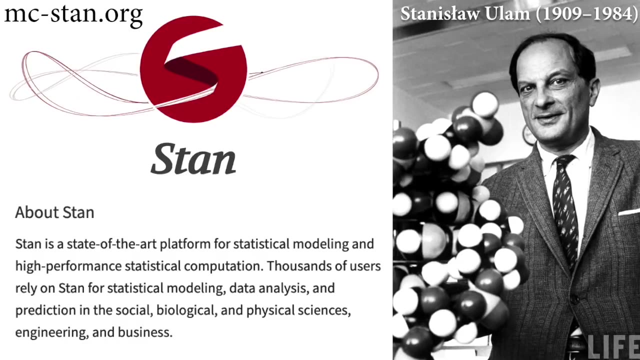 and this makes things really nice. Stan is a very professional open source scientific computing project that is used both in the sciences and in industry quite a lot now. and Stan is not an acronym, it doesn't stand for anything. Stan is a man, or was a man he was named after. 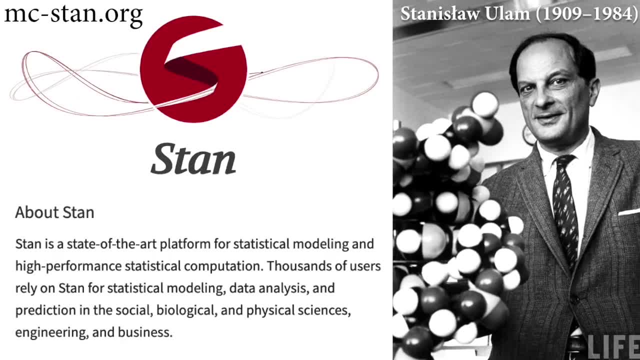 Stanisław, I think that's pronounced. it's a Polish name, Stanisław Ulam, who lived between 1909 and 1984, and Stan is credited as the father of Monte Carlo methods. he's a brilliant mathematician, fled Europe during the second world war. 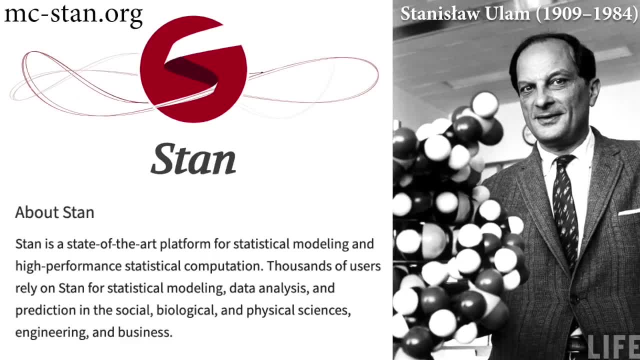 like many brilliant European mathematicians, and went on to make very important contributions in many areas of mathematics, physics and biology. really an extraordinary career. Stan math library is named after him because of Stanisław's contributions that paved the way for later innovations in Monte Carlo methods. 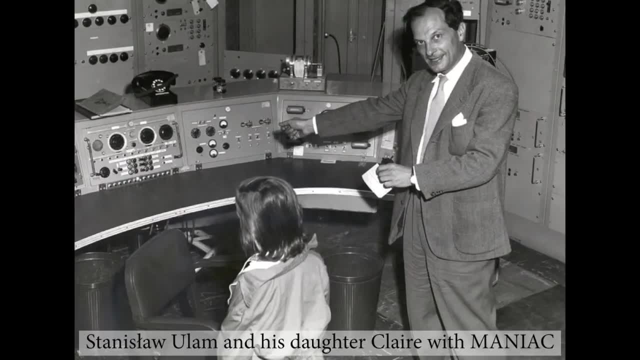 oh yeah, here's Stanisław with his daughter Claire, when she was quite young at Maniac, because they all worked at Los Alamos and Stanisław did analytical mathematics to design the calculations and then Arianna Rosenbluth and others programmed the computers to actually execute them. 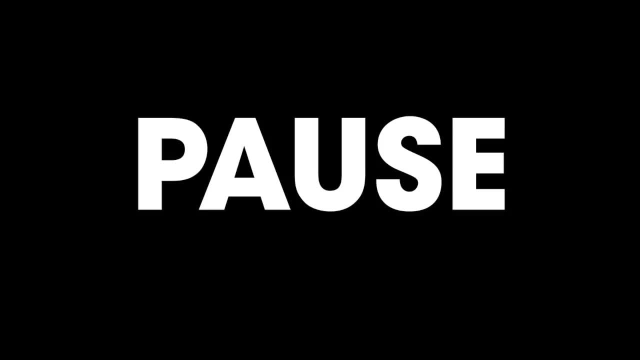 okay, that's a lot and it's mostly conceptual work so far, but nevertheless I think we should pause and, as always, it'd be a good idea to take a look back through the slides so far, see if there's anything that remains confusing. take a couple notes. 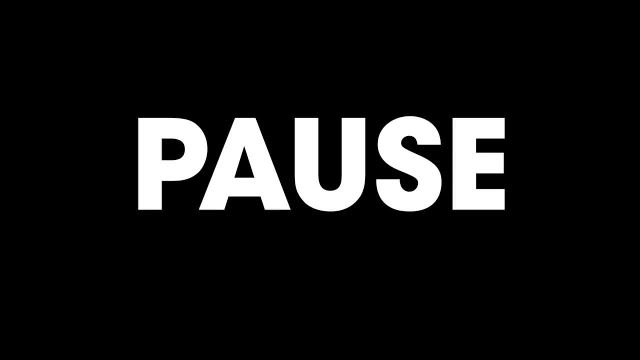 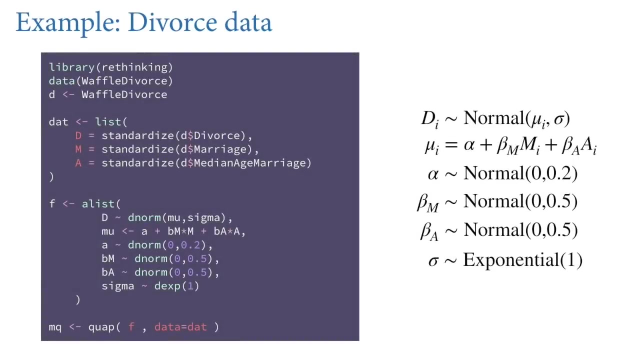 then go for a walk, have a cup of tea or coffee, and when you come back I'll be here. welcome back. let's pick up by actually doing some work now. so what I've tried to do so far in this lecture is give you a conceptual heuristic. 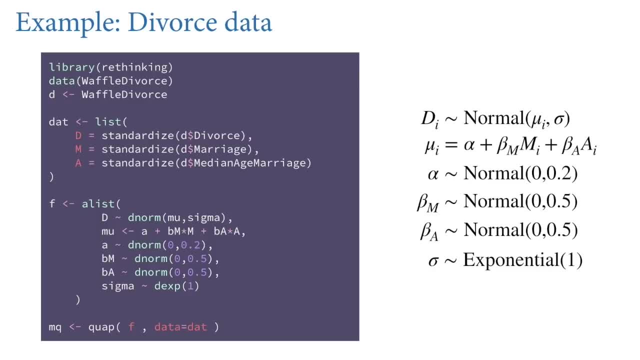 and a little bit of a historical introduction to both Markov chain and Monte Carlo, and especially Hamiltonian Monte Carlo. now I want to show you more of the workflow that we do with this in a typical applied Bayesian data analysis scenario. so let's go. let's revisit an example we already know. 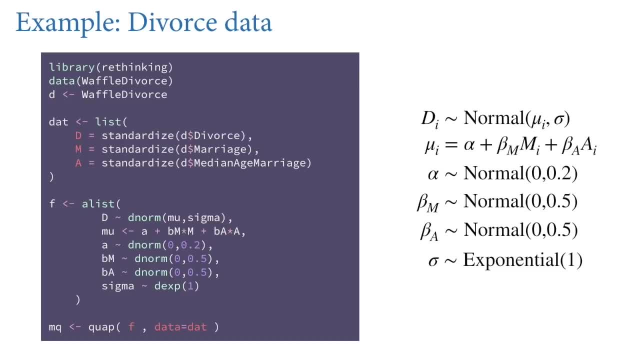 so I don't have to introduce a new data set. let's think of the divorce data again from last week. all I'm doing on this slide is trying to remind you of the model we used to analyze that data set. this is a linear regression. I'll show you the mathematical model notation. 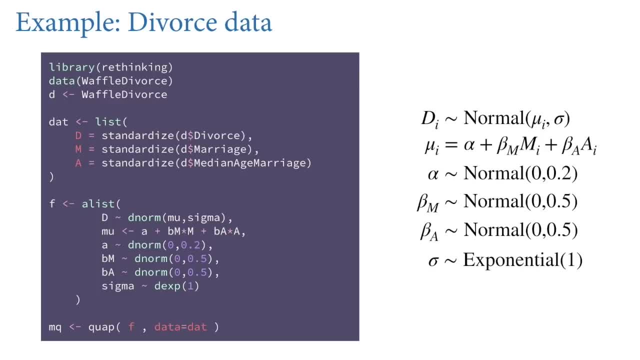 on the right of the slide, the code on the left. it's a linear regression with two predictors, that is, we're stratifying divorce rates simultaneously by marriage rate and age at marriage. that's D for divorce rate, M for marriage rate and A for age at marriage. 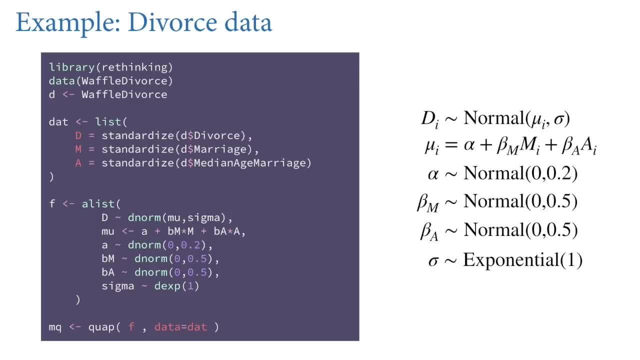 no surprises, I hope, by this point and the code on this slide you would have used before. all that's different about it is I've defined the formula list as a separate object and then passed it into the QAPP call at the bottom of the code block there. 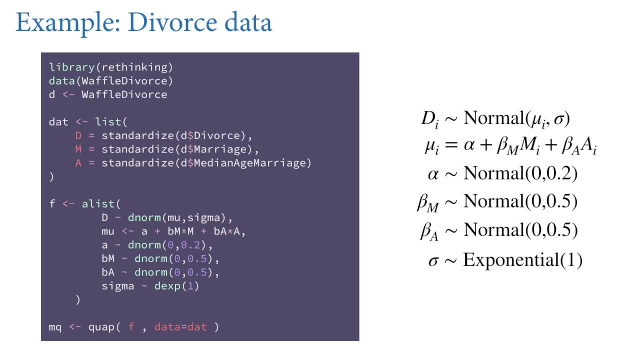 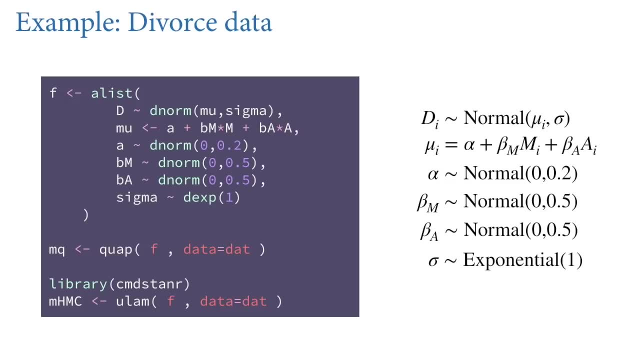 to fit this same model with Hamiltonian Monte Carlo. if you're using my rethinking package, all you need to do is pass the same formula list to the ulam function shown at the bottom, and what ulam will do is it will actually pass the whole job over to the stand math library. 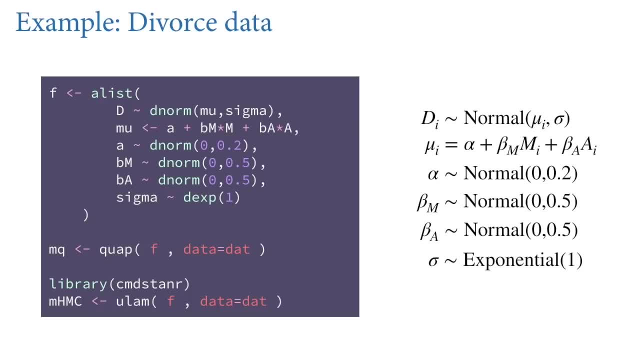 let it compute the gradients, run the physics simulation, collect the samples and then ulam will return those samples to you and you can analyze them, just like the samples from QAPP. that is all the same convenience functions that you've been using so far to analyze QAPP models. 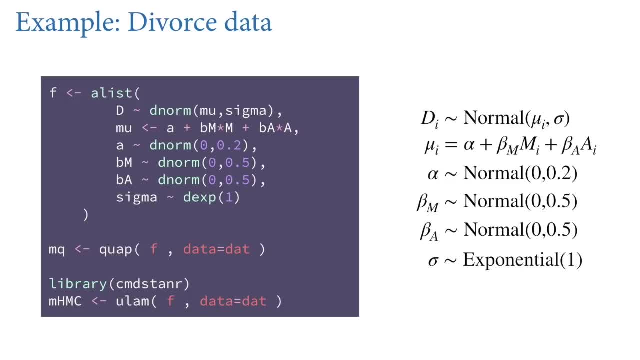 like LINQ and extract samples will also work for models you fit with ulam. all the machinery is different under the hood. everything you've learned so far about how to analyze posterior distributions is still true, and you've already learned how to work with samples. in this case, this is all we get. 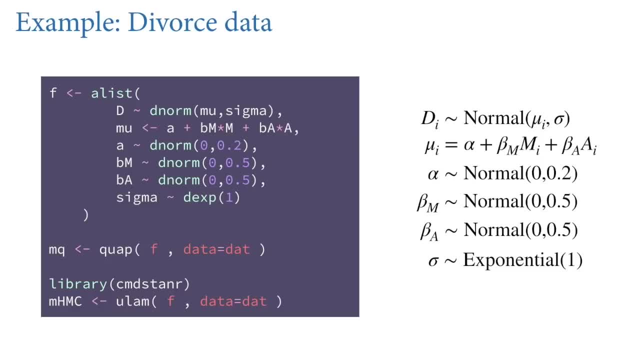 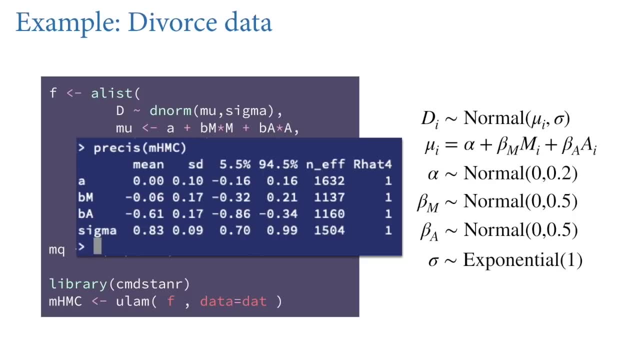 all we get are samples. there is no analytical representation of the posterior distribution when you do Markov chain Monte Carlo. but now you're already a pro at that and you're ready to go, so you run this. I encourage you to run this. make sure you get everything installed right. 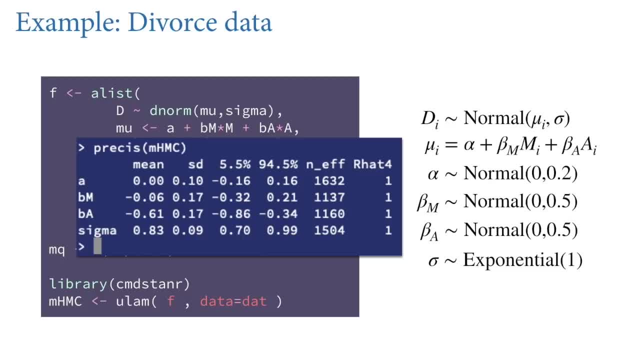 and see if you can reproduce the results of the Preci output for the divorce model fit with Hamiltonian Monte Carlo and the means and standard deviations and compatibility intervals are practically identical. this is a standard linear regression. we don't need Hamiltonian Monte Carlo for a problem like this. 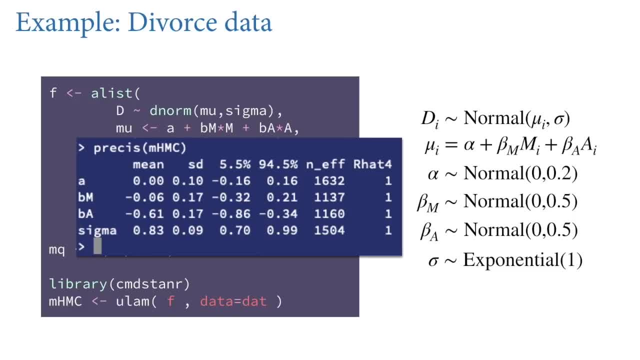 but this is where we start, so that you understand that it's giving the same results in principle and as we scale up to bigger kinds of models. quadratic approximation simply won't work at all and we're going to have to do it with Hamiltonian Monte Carlo. 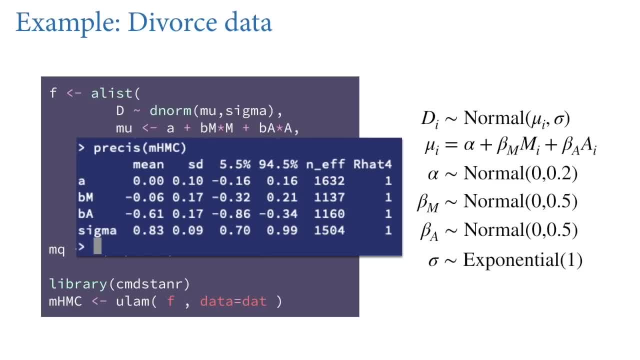 but I'm sure you've already noticed, there are these two new columns on the right, the NF column- you can say that NEF, if you like. I tend to say NF- and RHAT4. I'm going to explain what those are in a bit. just hang on a second. 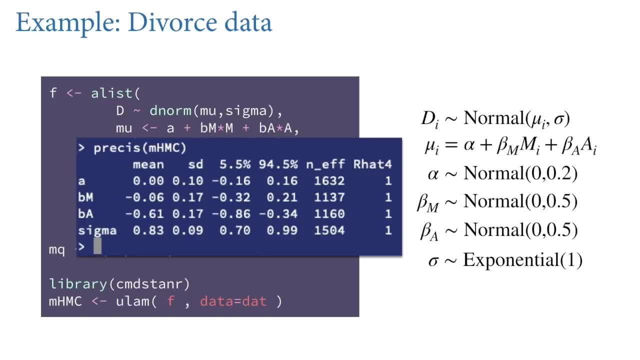 but what they're about is diagnosing how well the simulation has functioned, how well the skater performed, as it were. before I do that, before we talk about the workflow and diagnosing the machine's performance, I want to talk about what this model would look like. 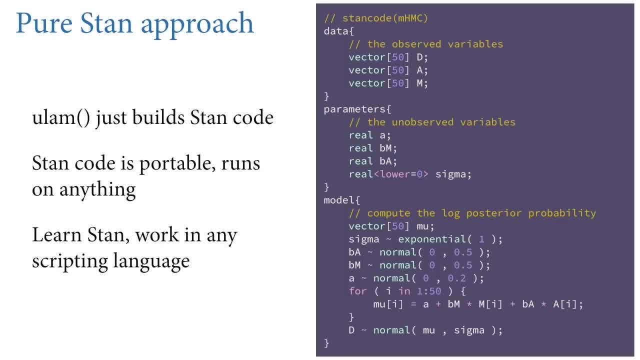 in pure stand code. so ULAM is a convenience function so that you can keep working with those standard kind of mass stats model formulas. but what's really going under the hood in scientific computing requires more input than that, because the mathematics is ambiguous. in those formulas there's a lot of intuitive knowledge that you bring to the context. 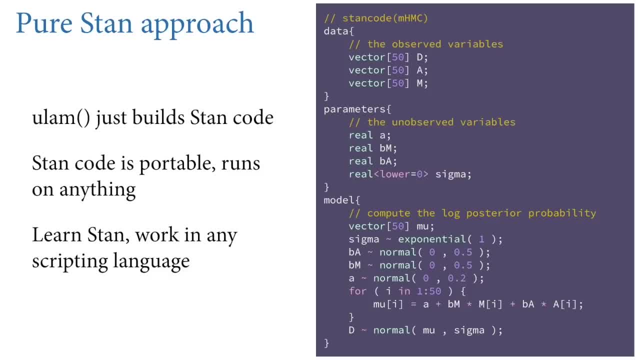 but the computer needs to be told that because it doesn't know it now if you're not interested. so what I'm going to do in the next couple slides is show you what the stand code is like and give you some first meeting with stand, just so you get it. 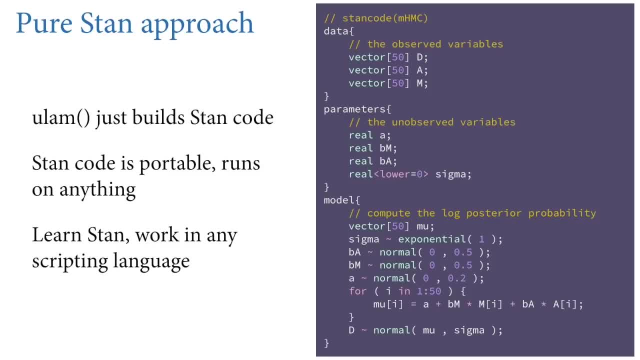 so it's less mysterious. if you're not interested in working with stand right now, feel free to skip this section and keep going. you can check the chapter bookmarks on the YouTube progress bar on the time progress bar at the bottom of the video. so stand code is: 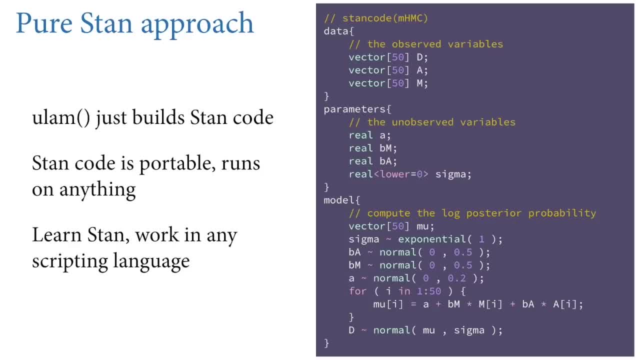 worth learning on its own. eventually, I think about my rethinking package as just a scaffold to get you into using stand or some other similar programming language like Turing in the Julia environment, and the reason is because these probabilistic programming languages like stand or Turing are incredibly expressive. 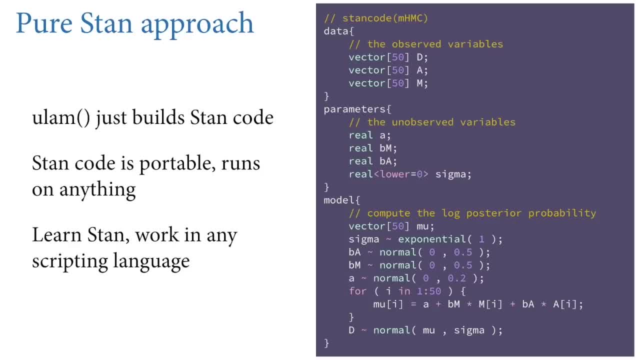 and you can do a lot more with them if you're comfortable with programming in them directly. they're also very portable in a way that R code is not. of course, R is portable on lots of devices. you can probably run it on your watch now, but the same stand model. 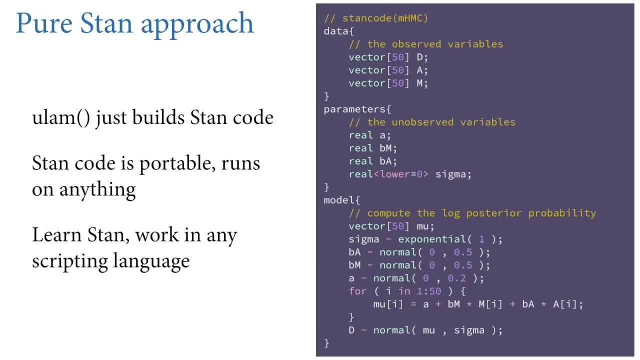 can be compiled in any scripting language, because stand doesn't depend upon any particular scripting languages, and that means that you can share it with lots of colleagues in high performance computing. on the right, I'm showing you the stand code for the device and the force model, and you can always get Ulam. 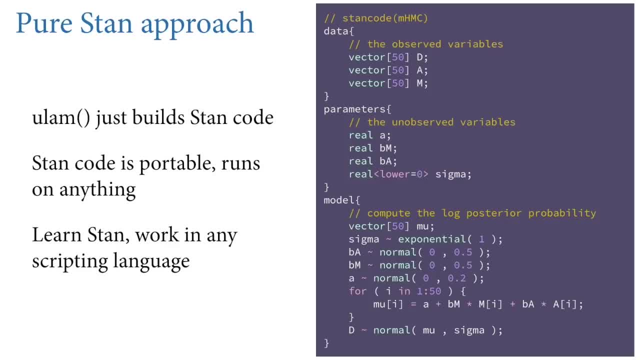 to spit out the equivalent stand code by typing the command at the top here that I've commented out- the stand code function, and then the name of the fit model object, and then it will display the stand code that was actually run. let me explain each of the parts of this. 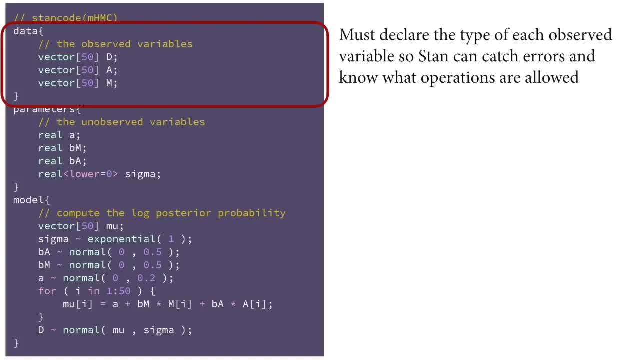 for you, and I'm not going to go into intricate detail here. I just want to give you an idea of the general personality of each of these blocks. the top part of every stand model is a data block, and this is where we declare observed variables. it's things usually that we call data. 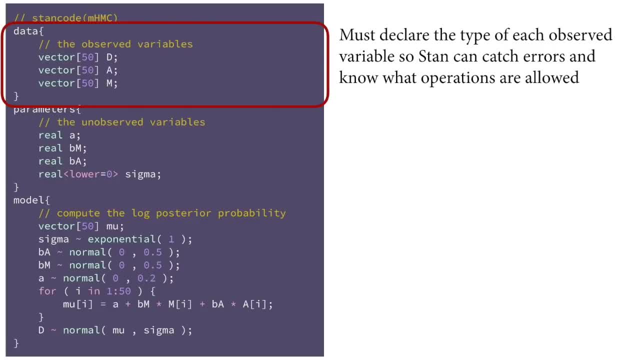 but they're observed variables in Bayesian data analysis. so these are the divorce rates, the ages at marriage and the marriage rates, and you'll notice that the names are the same here- D, A and M- but they're all prepended by this word vector and then in brackets, 50. 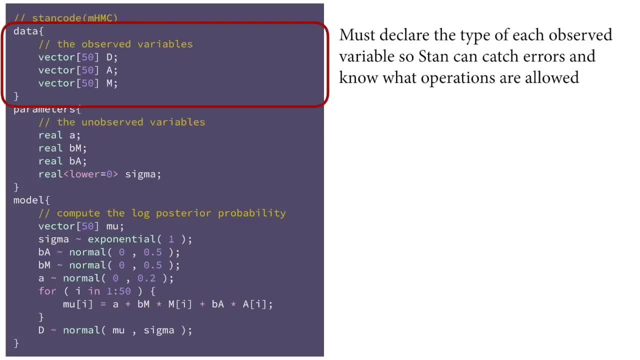 50 is the length, there are 50 observations, and vector is the kind of data. it tells Stan how the variable is represented in memory. and this is if you haven't programmed in languages like C that require this. this seems really strange because R and Python don't normally require you. 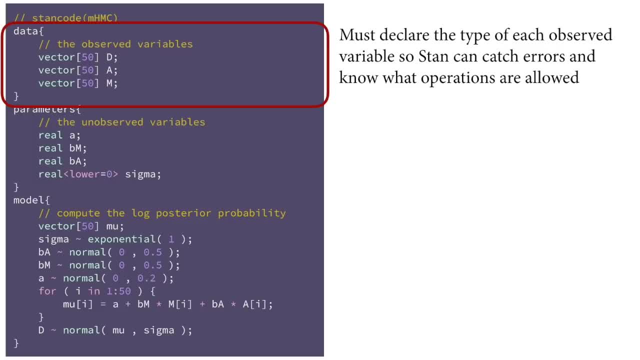 to say anything about the representation of the variable in memory. maybe, once in a while, you've coerced something to be an integer, and so you've gotten a slight whiff of this and what it's about. this is essential, though, in high performance computing for code that's going to be compiled down. 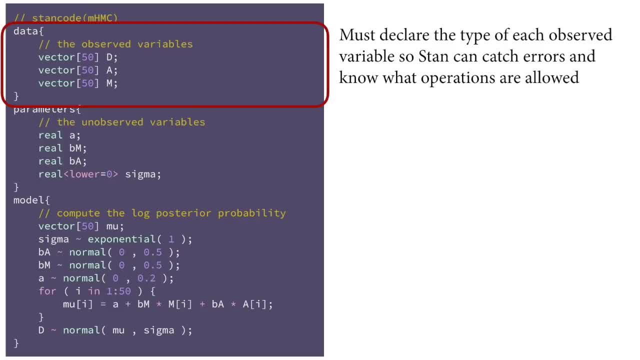 in machine code. you have to tell the computer unambiguously what the memory representation is going to be, and the reason is because this allows Stan to catch errors in your coding. that is, you try to do something that's not allowed with a particular type and 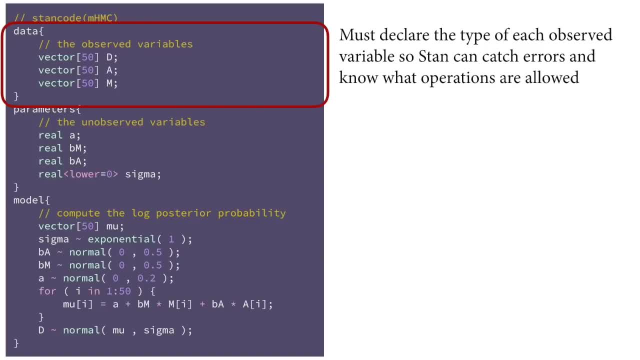 that's really indispensable because it reduces the amount of debugging you need to do. basically, it creates internal consistency, changes and checks of the code. it's a way of proofing the code as you write it, as it were. and the second block are the parameters. these are the unobserved variables in the model. 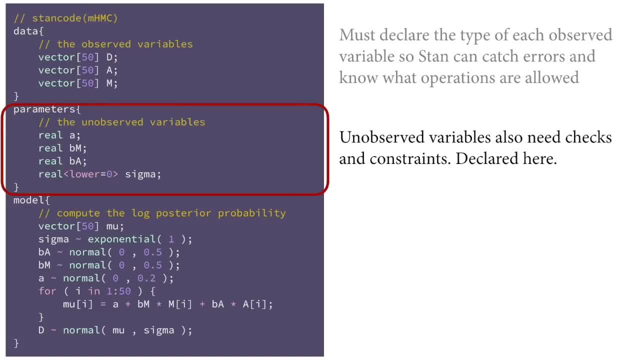 remember, in a fundamental sense, in Bayes, parameters are just unobserved variables, unobserved data. we'll push that metaphor to its limits in a later week, and the same thing holds here. Stan needs to know the types of each of these so it knows which checks to run. 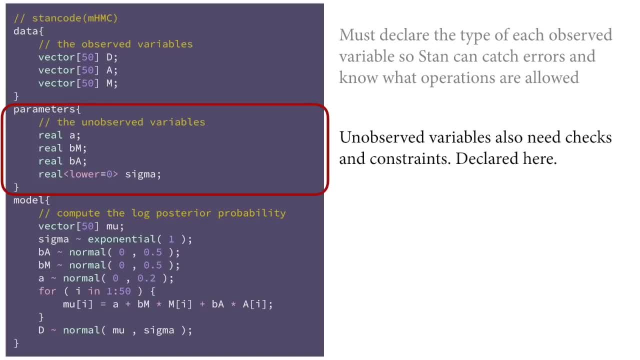 and which constraints exist. so notice, for example, that sigma here has a constraint: lower equals zero. it must be a positive real value. finally, there's the model block. this is the block that's most similar to the code you've been writing so far. it restates the distributional 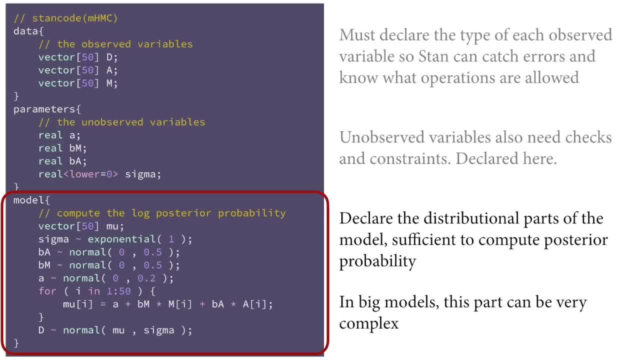 assumptions of the model, the squiggles we've been putting into our model formulas up to this point. but you can put a lot more kinds of code inside of a Stan model block than you can in a Quap or Ulam model, although you can do a lot in those as well. 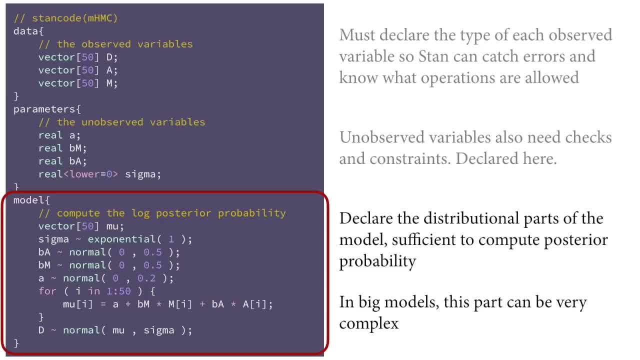 in very large models, complicated models like latent variable models. the model block can become very complicated. you can analyze multiple data sets at the same time, have complicated simultaneous equation systems, ordinary differential equations, large numbers of things. we're going to keep doing regression for a little while with this. 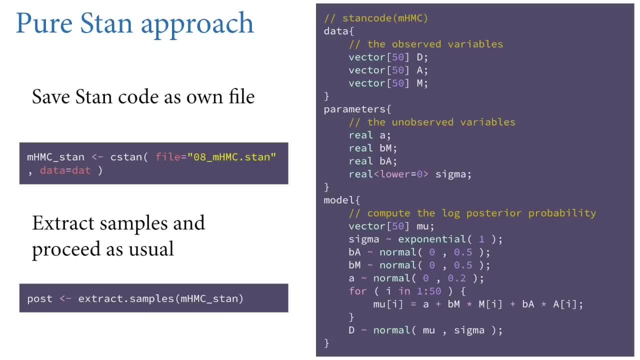 and we'll gradually build up the complexity, so there will be no sudden transition. okay, to run the Stan model. what do you do? well, you take that Stan code and you save it as its own text file, and this is a hygienic way to do scientific computing. 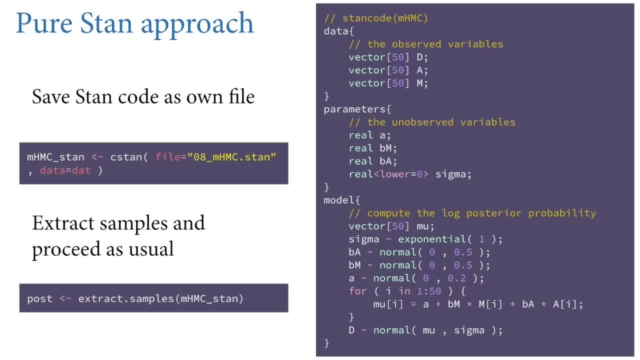 you make each, each Stan model its own independent text file so you can manage the complexity of your project. and then, if you're using rethinking, you can just pass this the name of this file, command C, Stan for command Stan, and it will sample just like Ulam does. 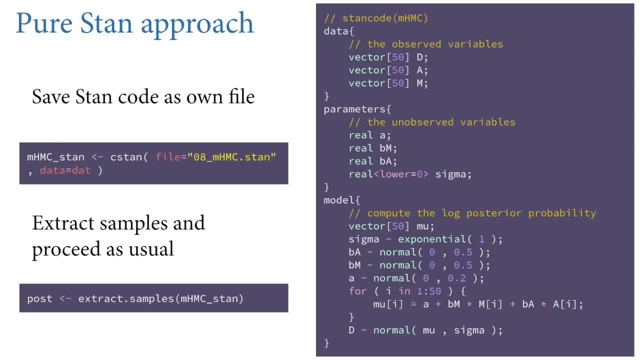 because this is what Ulam does, except Ulam builds the Stan code for you and then it passes it to command Stan and then returns the results to you. so you're just skipping the middle man here and hopefully understanding the underlying complexity a little better, and then you can work with samples. 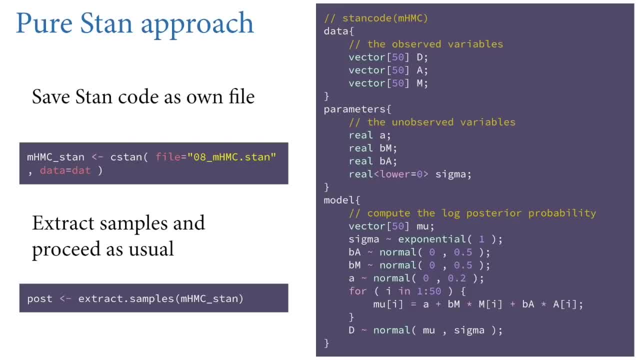 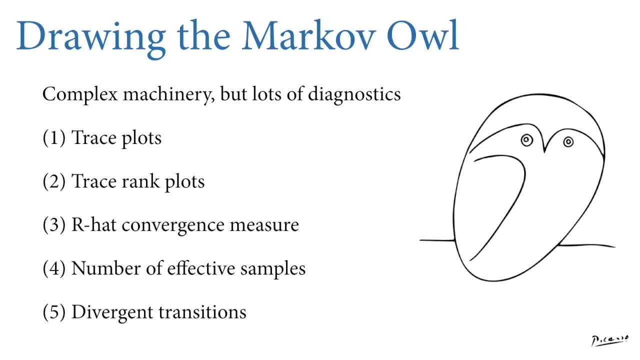 from pure Stan models, just like you did the others, because it's the same output, no matter what interface you use. if you're using Markov Chain, Monte Carlo, if you know the model, once you get the samples you can compute anything you need. okay, let's continue with. 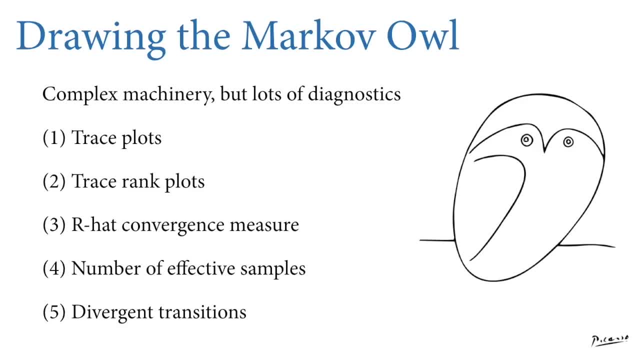 thinking about the workflow here and in particular, I want to emphasize sort of hygiene responsibilities that we have when working in scientific computing algorithms like Markov, Chain, Monte Carlo. these algorithms are seemingly magical when they work, but they're not magical because people have spent a lot of time. 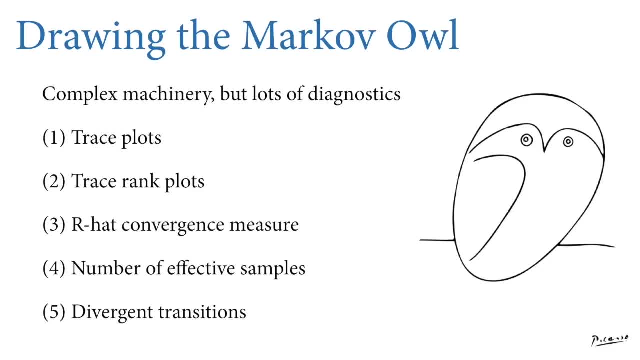 making them work and thinking about ways to diagnose when they don't work. so I want to spend a little bit of time introducing you to the diagnostics that we use in Markov Chain, Monte Carlo. this is really an essential part of the workflow. it's in the same sense that the other things are. 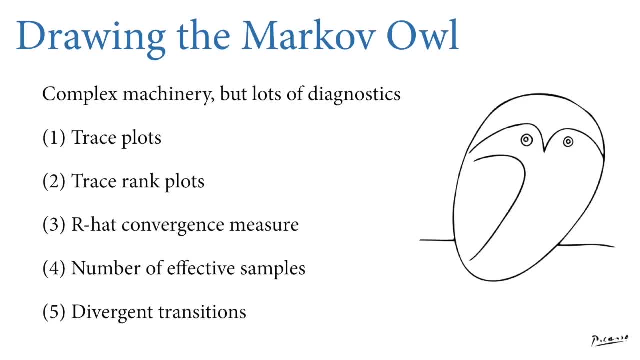 like stating your estimand and justifying the statistical strategy. those are general responsibilities. when you use Markov Chain, Monte Carlo, you have the responsibility to check that the algorithm functioned correctly and also to provide the information so your colleagues can trust that it functioned correctly. 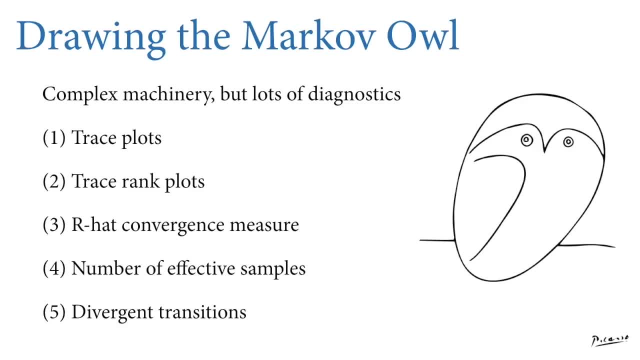 just like all the other parts of your analysis- and I'm going to go through five different things just to introduce them to you- and as you do this work yourself, you'll quickly become comfortable with each of these forms of diagnostics and understand the relationships among them. the first one, 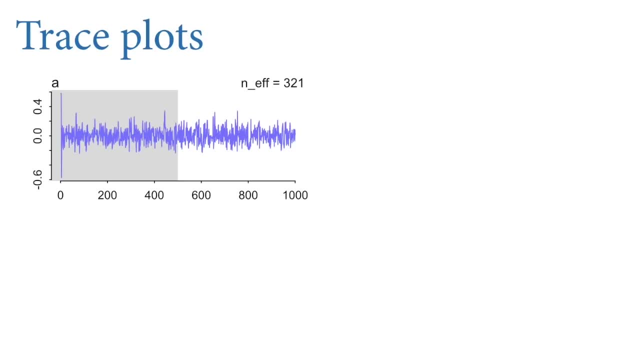 is called trace plots and in a sense this is the graphical display that people most associate with Markov Chain, Monte Carlo. in the trace plot, all we do is take the sequential samples from the Markov Chain for each parameter and we plot them as a timeline. so here for the divorce model. 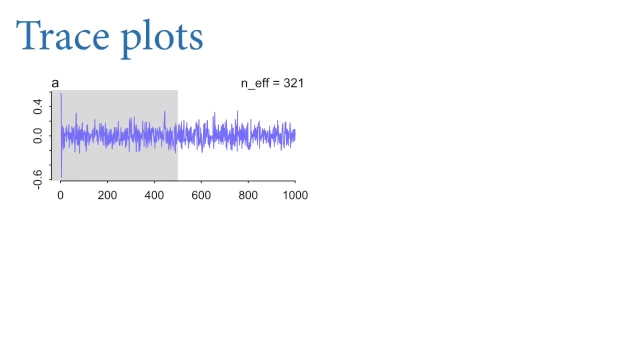 I've taken the intercept parameter alpha and I've just plotted the sequential samples. we took a thousand samples from the Markov Chain, starting on the left and going all the way to the right, and the gray region is a region that's called the warmup by Stan. 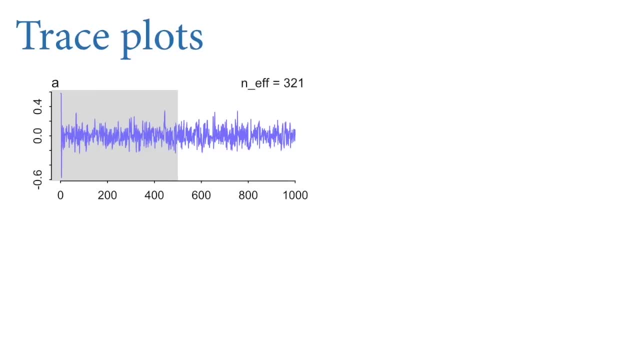 and the warmup is when Stan is figuring out step size and how long the trajectory should be. I say more about this in the book and you can read a lot more about it in the Stan manual, if you like. we don't usually use the warmup. 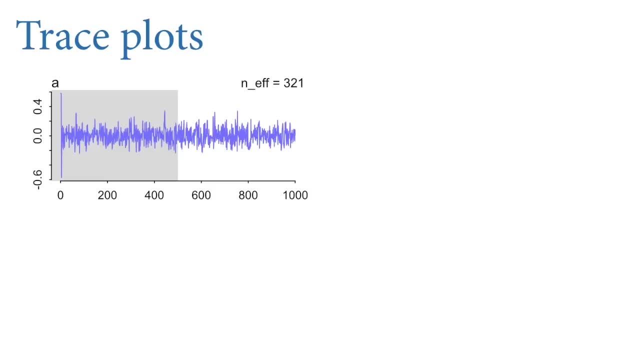 for inference. it's not necessarily a valid part of the posterior distribution, but it's nice to show it in the trace plot so you can see how the warmup phase proceeded outside of the warmup phase on the right half of this graph. those are the 500 samples. 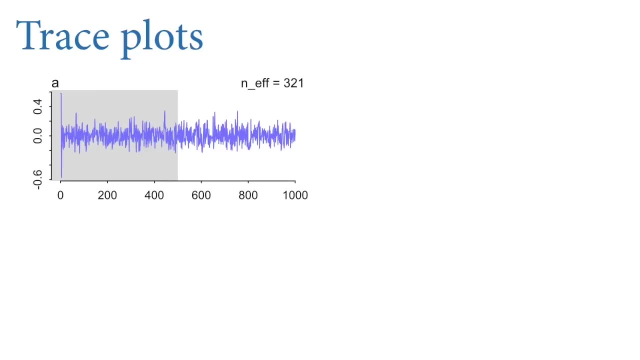 we have for inference, which in this case, is plenty. you'll see that there's an NF equals 321 displayed in the upper right. I'll talk about that in a minute. let's turn our gaze away from that for now. we don't just look at one parameter, though. 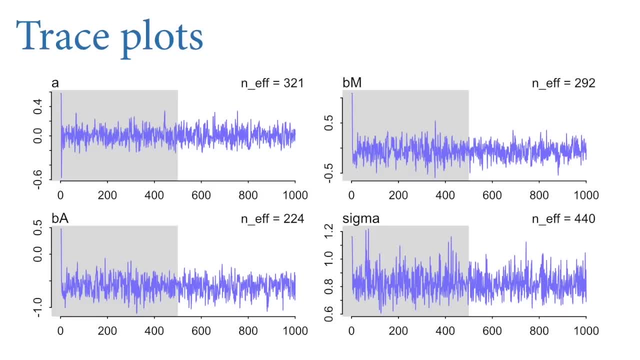 we look at all the parameters. we want to ensure that for every parameter that the trace plot looks healthy. and what does that mean? well, that means that it's stationary. it tends to stay in the same part of the distribution as these four do. you'll see that they're zigzagging around. 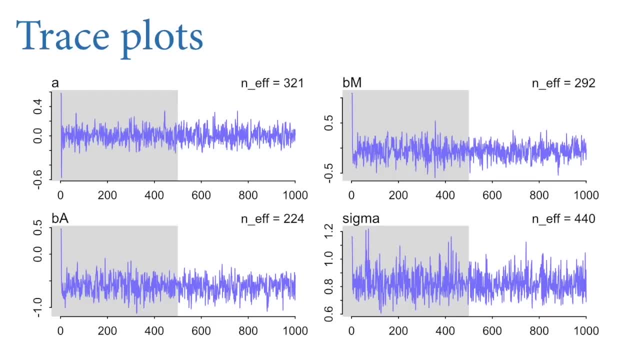 within the same area. they don't drift up and down. to a large extent as the simulation goes on. they're exploring the lower part of the half pipe, as it were. sometimes people say that it's the hairy caterpillar test you want the trace plots to look like. 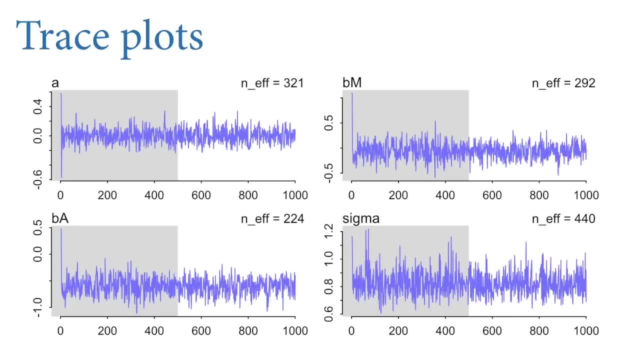 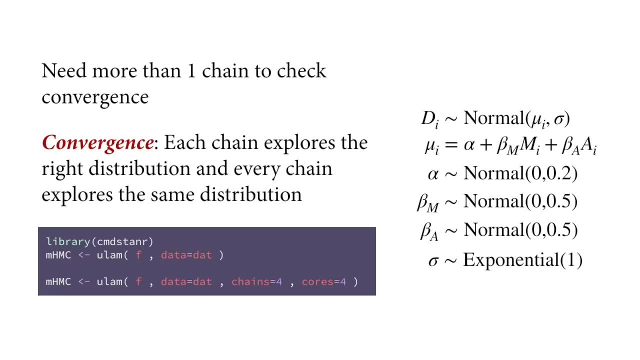 hairy caterpillars, if that's something that you're familiar with. so one chain is not enough. what I've just showed you is the trace plot for only one Markov chain, and typically we will run more than one Markov chain simultaneously, and we do that because 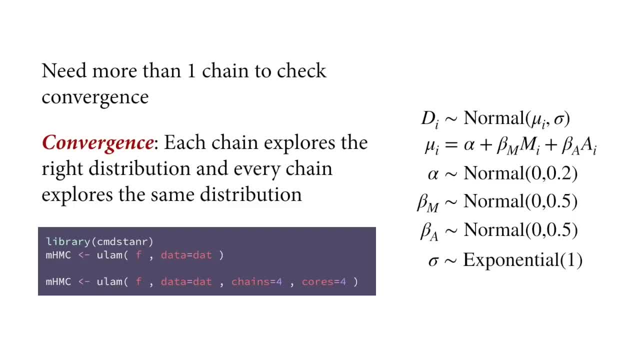 a strong test that the chain is healthy is that multiple chains converge to the same distribution. this is a criterion we call convergence. you want each chain to explore the correct distribution and stay there when it finds it, and you want every chain to explore the same distribution, that is, to be stationary in the same place. 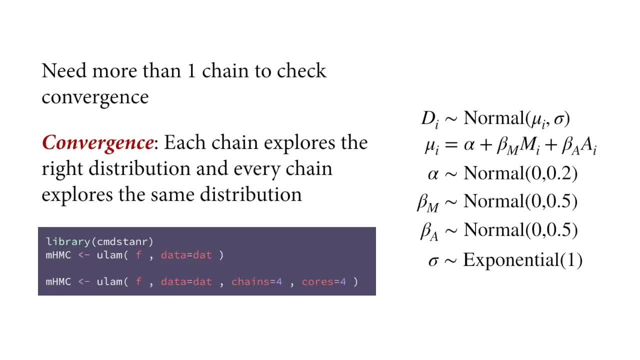 and that means starting multiple chains from independent, different starting locations- often quite dispersed starting locations- and ensure that they converge to the same distribution. this is easy to do in Ulam. you just add the chains argument. four is a good number. most computers have lots of cores these days. 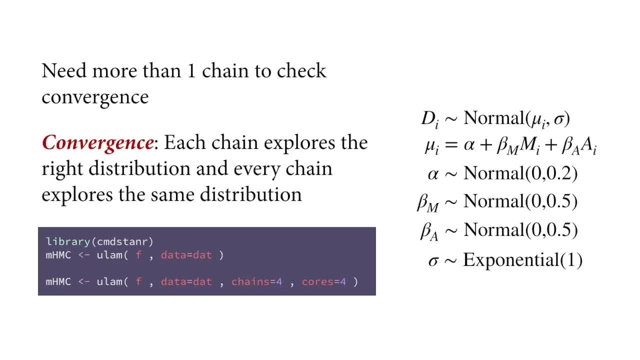 and you can run a different chain on every core in your computer, and if you want it to run them all simultaneously, be sure to add the cores command as well. so here I'm running four chains on four cores and they'll all run simultaneously. and this model runs very fast. 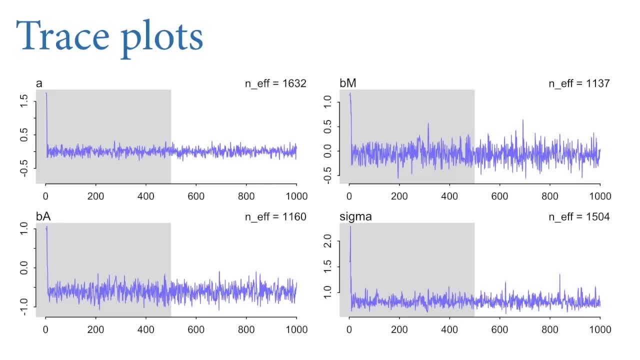 try it for yourself and see. and now I'm going to layer them in. this is what we showed before. it's the first chain from this model, and then the second one converges very quickly to the same place and stays in the same place, and then the third one, and then the fourth one. 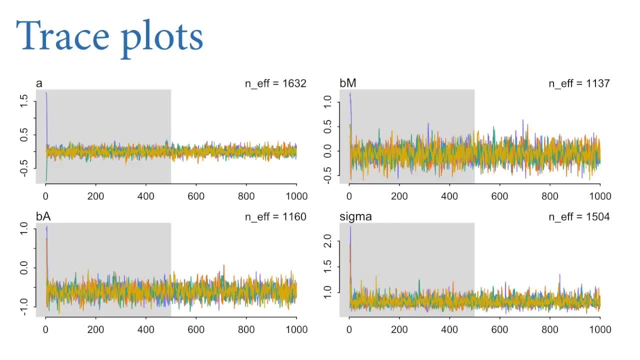 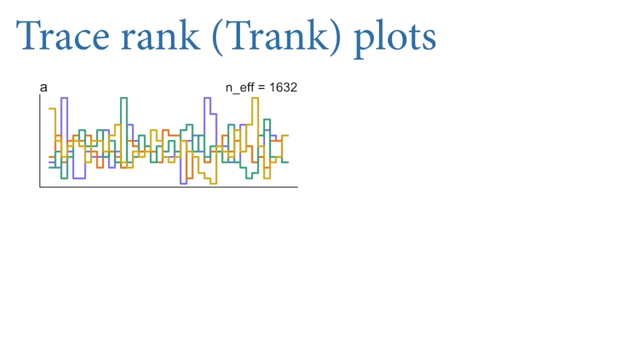 and this is what you want to see now. this is not a guarantee that the Markov chain function correctly, but if the Markov chain functions correctly, this is what you should see. trace plots are pretty limited, though. one of the things about them is that the chains overlap. 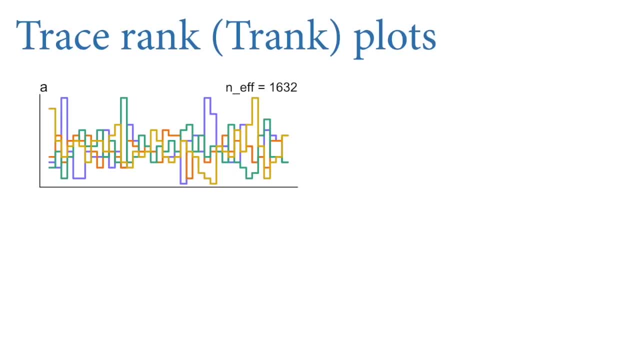 the fuzzy caterpillar is too complicated, and so there could be a chain in there. that's misbehaving and you can't see it because it's occluded by the other parts of the caterpillar, if that makes any sense. so a more recent graphical innovation. 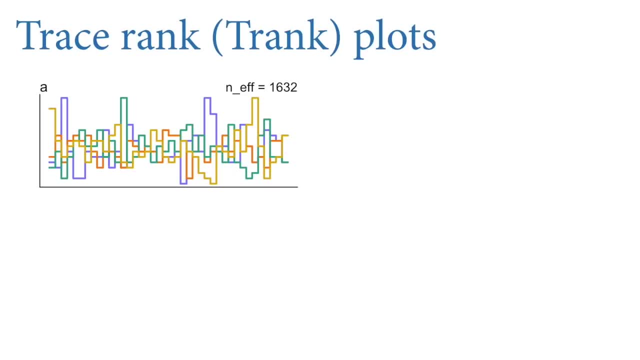 that I like a lot more are these normalized trace rank plots. I call them tranq plots. no one else does, but I'm going to keep trying to make fetch happen. and tranq plots? well, first of all, they're just gorgeous. I hope you agree to the one on this slide. 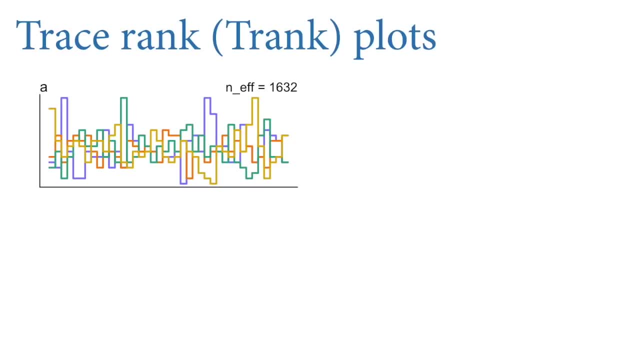 what are they, though? so, again, they're trace plots, so the horizontal axis is sequential samples. on the far left is the start of the simulation and then on the right the end, and this is just a post warmup sample, so I'm not showing the grey region for the tranq plot. 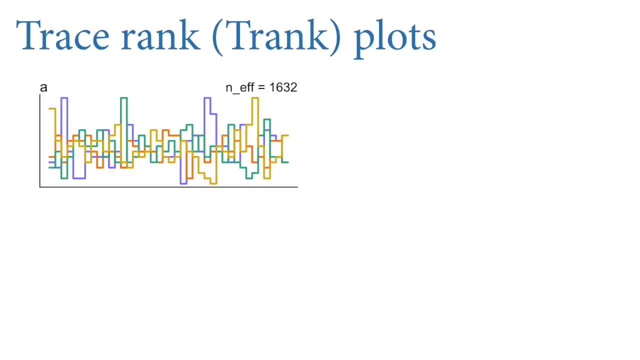 and then, instead of the vertical axis representing the actual parameter value, we've converted all the values to ranks, relative rank orders across the chains. and why would we do this? well, because it makes a quick, heuristic way. well, I should say it's good for the calculations of the later criteria, like R, hat and F. 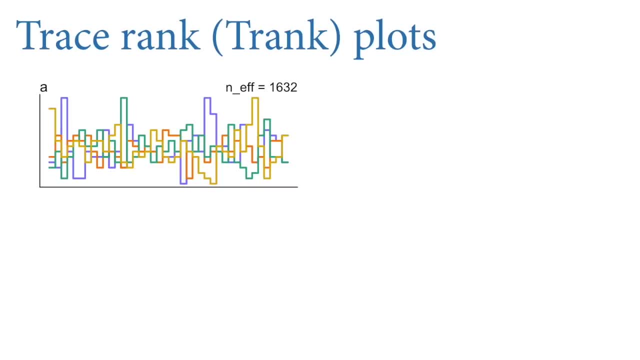 that we're going to talk about in a bit, but it makes a great visual, heuristic way to quickly assess whether any chain is consistently above or below the others. I'll say that again: it creates a quick, heuristic, visual way to assess if any one of the chains 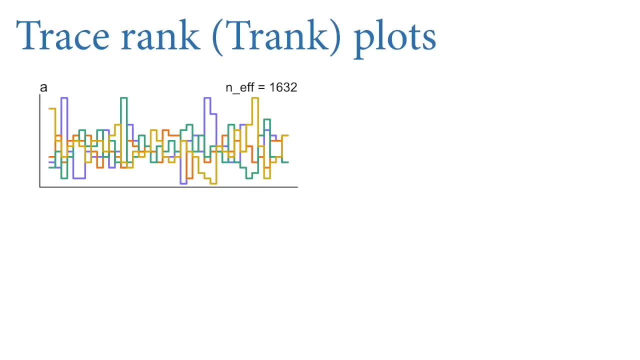 is consistently above or below the others. what you want to see is what I'm showing here, which is that the colors zigzag in and out of one another in this mosaic fashion, so which chain is on top is constantly switching, and that means that the chains are exploring the same space. 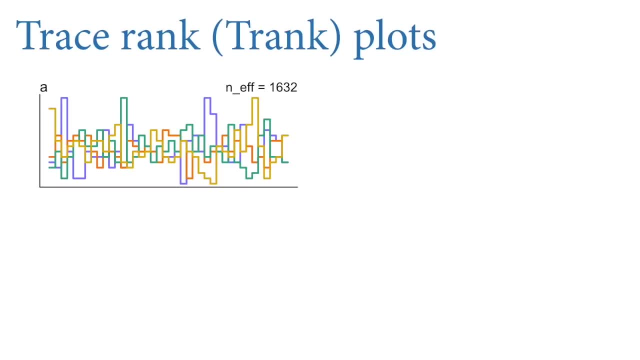 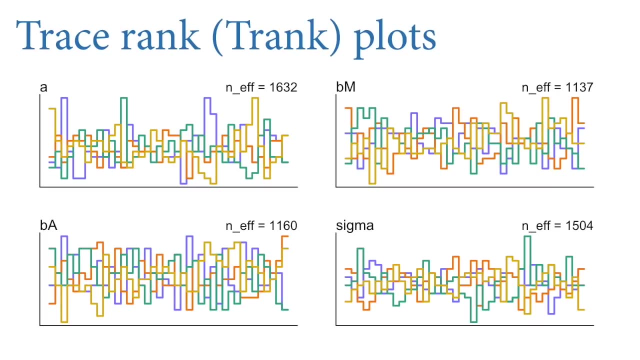 I'll show you what a bad one looks like in a few slides, so hang on and you can see. for the other parameters, the same sort of pattern. this is a nice, healthy chain. you get this mosaic switching of all the different chain colors, because no chain is consistently. 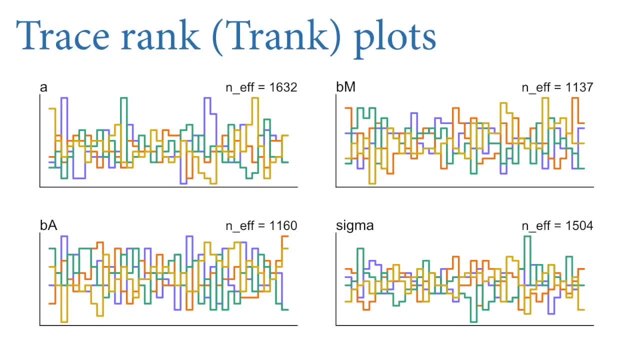 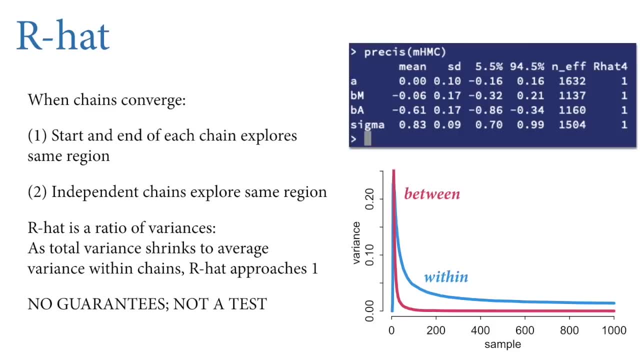 occupying a higher space in parameter values than the others. they quickly switch and dodge and weave among one another. okay, it's time to talk about these two numerical diagnostics that are displayed in the PRACY output: NF and RHAT. let's start with RHAT. RHAT is quite common. 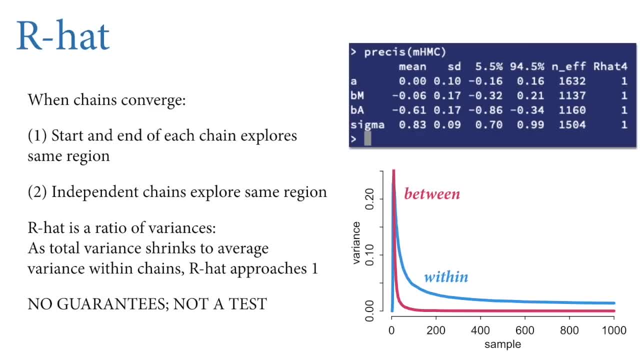 and maybe you've already heard of it: when chains converge, we want them to converge in two ways. first, we want to check that the start and end of each chain is exploring the same region. that means they're stationary. the second thing is, we want to be sure that 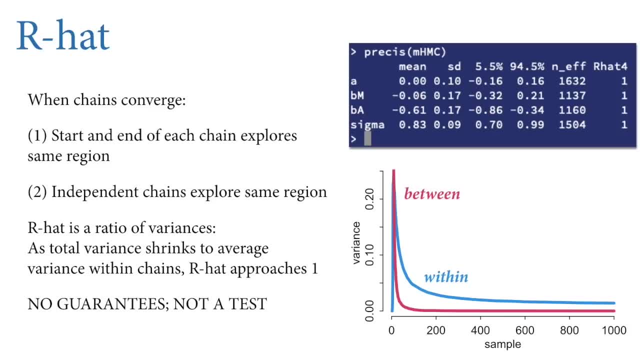 independent chains explore the same region. so we want the chain to sort of converge with itself. that is its start and its end to be in the same place. and we want different chains to converge to the same location as well- independent chains. so RHAT is a statistical 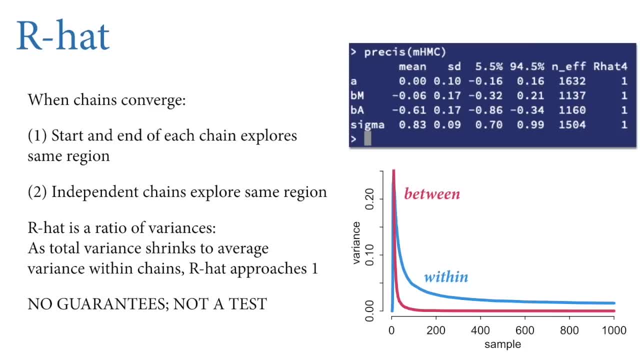 criterion for assessing this, but it's not a test and it provides no guarantees. nevertheless, it's really useful. what is it? if the total variance among all the chains for some particular parameter shrinks to be the same as the average variance within chains, then RHAT approaches one. 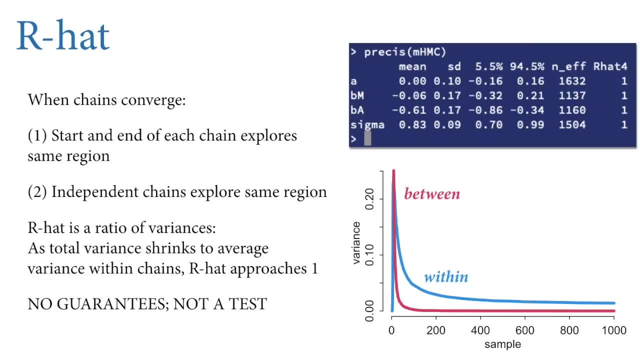 that's just the way RHAT is, because it's a ratio of these two things: the total variance over the variance within chains, one way to think about this. I'll try to help you with this plot on the right I've shown you for the chains that came out of this divorce model. 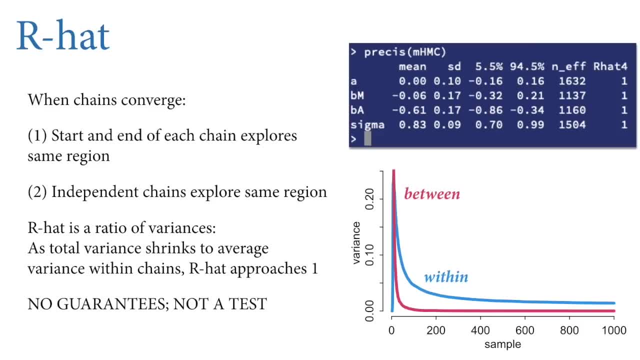 samples on the horizontal, sequential samples on the horizontal, and then variance on the vertical, and I've computed in red the between-chain variance. what does that mean? it means the variance among the means of the chains, the mean parameter values of the different chains, and then the blue trend. 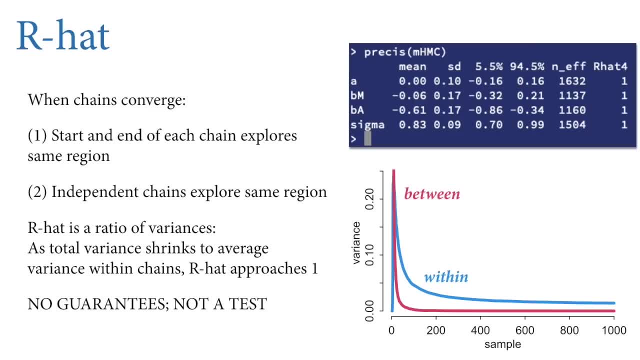 is the average variance within chains. so we compute the variance of each chain and then we average those variances. that's the blue trend. so what you see is that both of these converges. so initially they're very high because the chains are in different places and they haven't settled down yet. 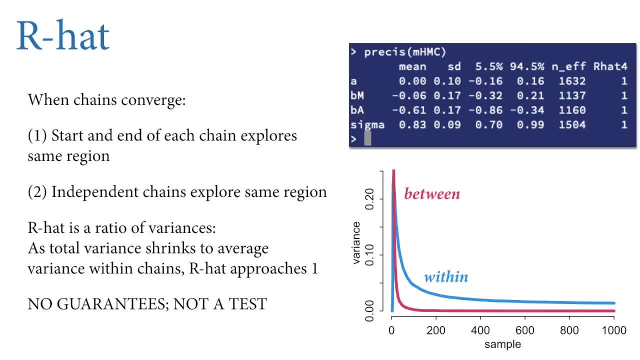 and then the variances decline as they stabilize and become stationary, but the red collapses much faster, because these are good chains, and that's what you want to see, is that the variance, almost all the variance- among the chains is within them, not between them, because they've converged to the same place. 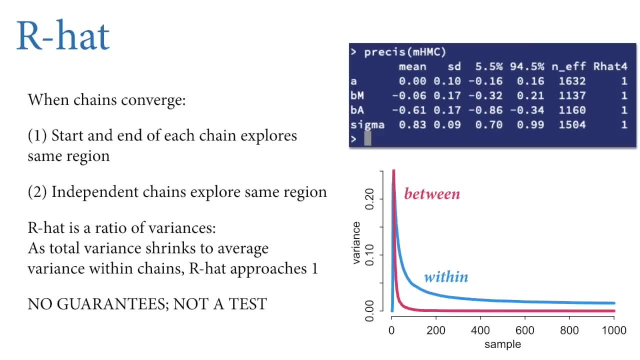 and so this is what RHAT does. large values above 1 are bad, and if you run the chain long enough, you want to see it shrink down to 1 or just above 1, like 1.01 or 1.02, but there's no threshold. 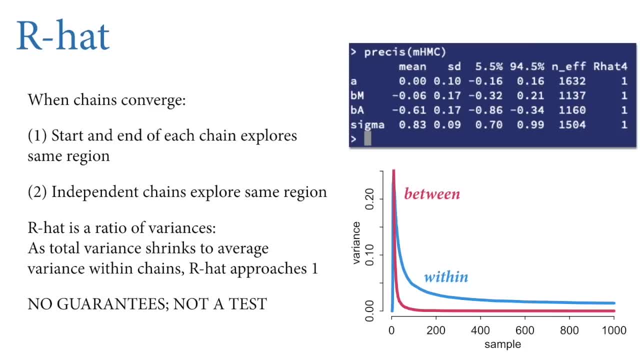 this is not a test. it's not a significance test or anything like that. it's a diagnostic criterion to help you as a warning signal. RHAT can equal 1 and chains can still be bad, but every little bit of information helps us. NF is the last one of these criteria. 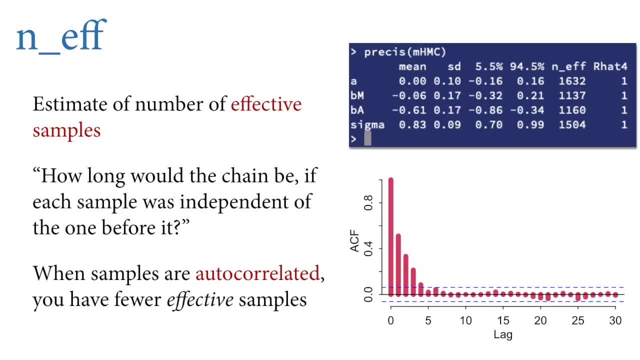 this is the often called the effective number of samples. so what does this mean? one way to think about this is that NF is the answer to the question: how long would a chain be if each sample from that chain was independent of the one just before it? this is a weird question. 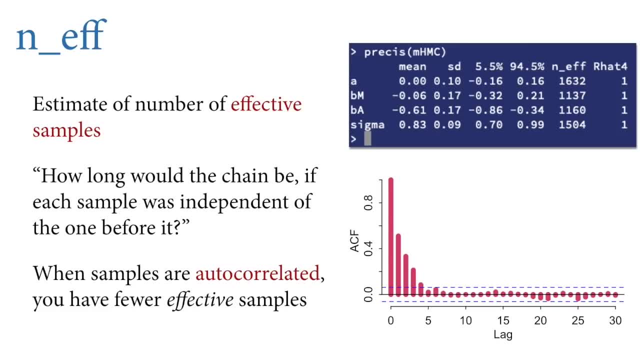 what kind of maniac would ask a question like this? it's actually a really important question because Markov chains are sequential. well, they're Markov chains, they're sequential. the next parameter sample is only on the most recent one. and what can happen as a consequence? 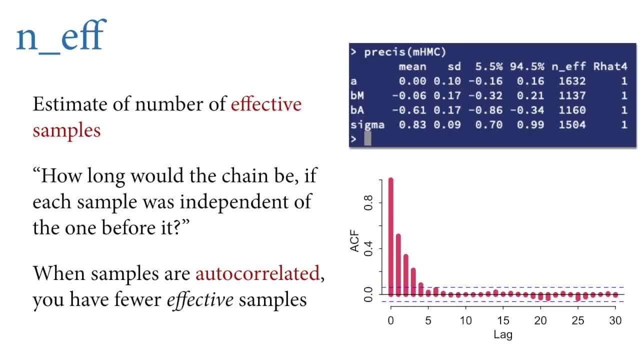 if the chain is not exploring the posterior distribution efficiently is that the sequential samples will be correlated with one another, and we usually call this autocorrelation, that is, self-correlation. so what I've shown you in the graph in the lower right of this slide is something called the 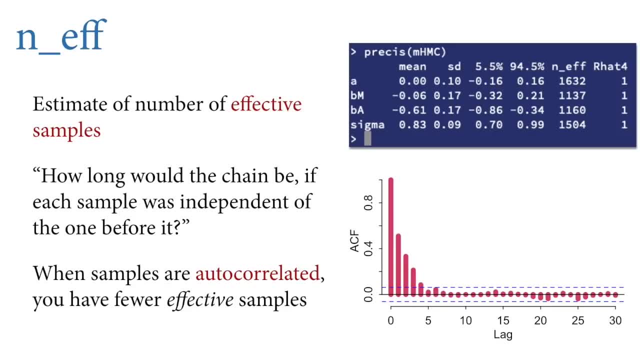 autocorrelation function for the chain, the Markov chain for the intercept and the divorce model, and the way to read these autocorrelation function graphs is that on the far left at zero lag, the horizontal axis is lag. you've got any location in the chain? 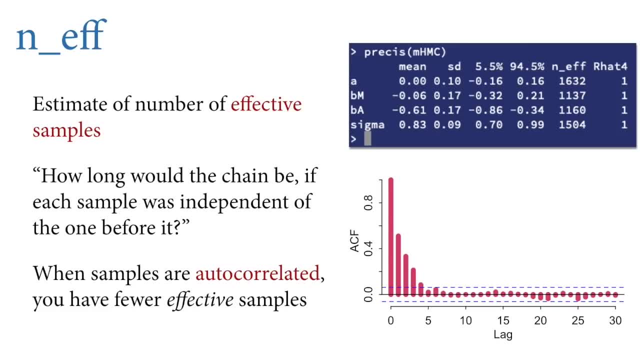 this is like: zero means self, and then the vertical axis is correlation, and so you'll see that the red bar there goes all the way up to one. that means each sample is 100% correlated with itself. yeah well, thank you, but the next sample, the one at lag. 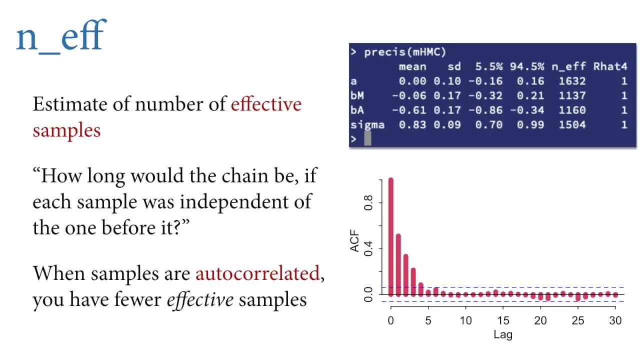 one right next to it, to the right, has a correlation about 0.5 and that means that each sequential sample is 50% correlated and then that correlation declines as we move away, so that by the time we're five samples away, there's essentially no. 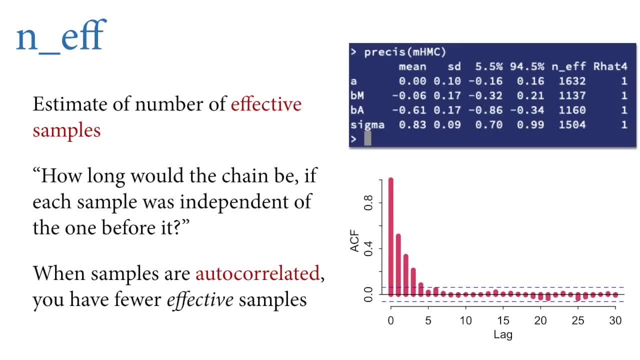 correlation between the parameter values that are sampled, and that's good. this could be better. often Stan will do even better than this and the autocorrelation will drop to almost zero after one sample. but Markov chains often show some autocorrelation of this kind. 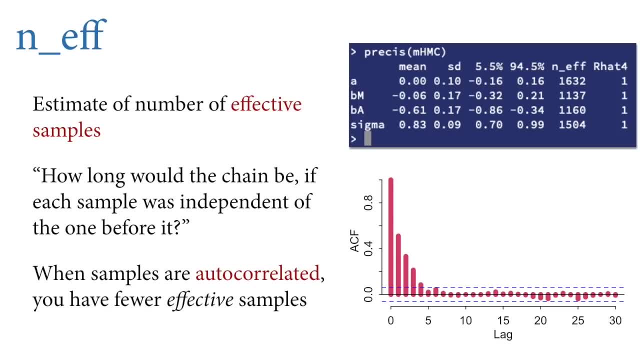 but you don't want it to go too far out. why it's not doom? it doesn't mean the chain's bad. after all, the metropolis algorithm generates really highly autocorrelated samples, but it still works. it doesn't mean anything's not working. 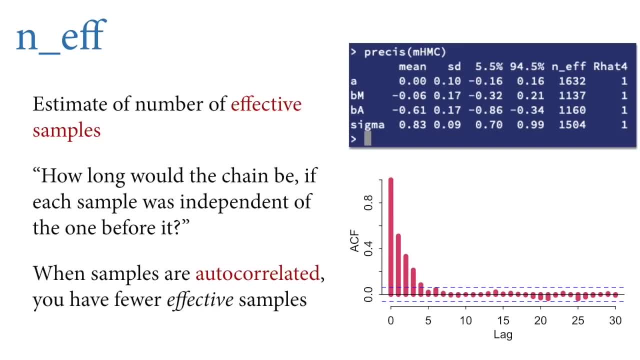 it just means it's less efficient and that means you have to sample longer. so NF is the answer to if we could imagine a chain- and we can- where there was no autocorrelation at all, so the autocorrelation function had a spike at zero. 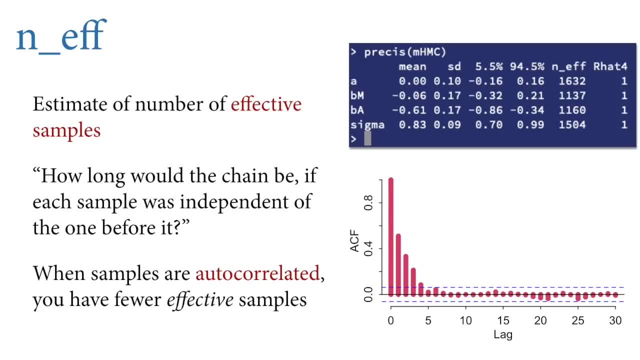 and then it was zero everywhere else had a spike to one at the zero lag, and then lag one was zero. correlation and so on. NF tells you how long that chain would be. so this is why it's called the effective number of samples and the effective number of samples. 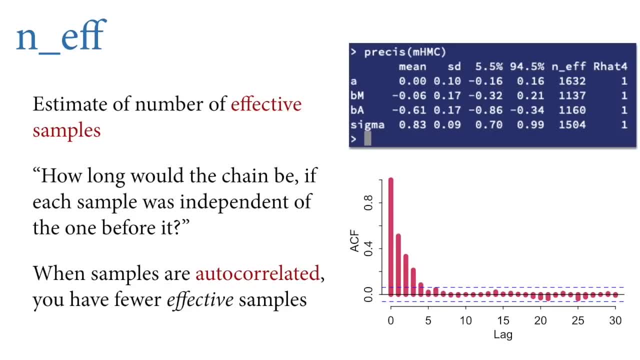 is nearly always- not always, but nearly always- smaller than the actual number of samples you took, because your chain has autocorrelation in it and that means sequential samples share information, so they overlap in the information they provide. if they were totally uncorrelated, they provide more information. 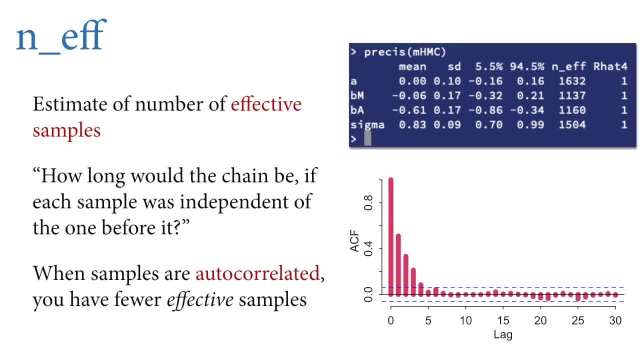 and so you'll see in the Precy output in the upper right the NF. so for this particular model we drew 2,000 samples. there are four chains and we're getting 500 samples from each, so that's 2,000 samples that we get to work with. 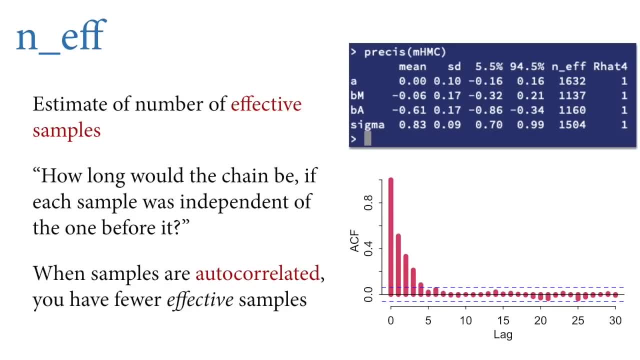 but all the NF values are less than 2,000. still, you don't need a lot of effective samples to get a good estimate of a posterior mean or even higher moments, some of the outer quartiles. so these are good NFs. how big should NF be? 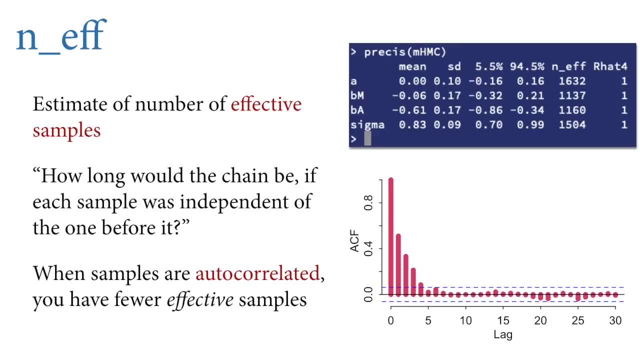 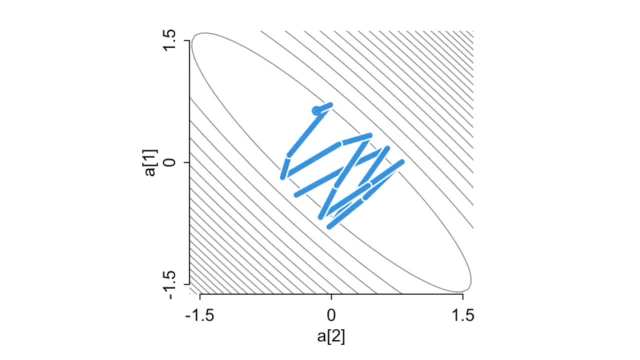 well, that depends upon your problem. I can't give you a general answer to that, but I say some more about it in the book. okay, last one to talk about in our hygienic workflow is this thing called divergent transitions, and I'm just going to say a little bit about them today. 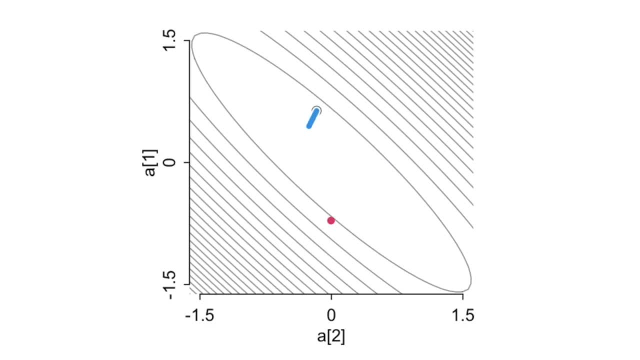 and we'll talk a lot more about them in a future lecture. the animation I'm showing you here is our skatepark example, again with a complicated shape, but I've changed the trajectories so that they're very jagged, so that I can show you what it looks like. 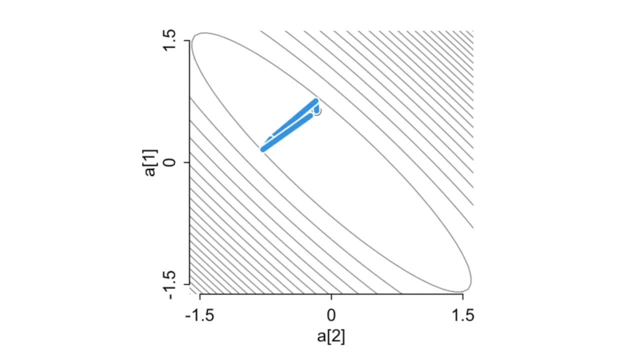 when Hamiltonian Monte Carlo rejects a proposal. so in this simulation you'll see this red point appears right there, and then when the simulation continues after it, it doesn't continue from the red point but from where it started the previous time. so watch it see. 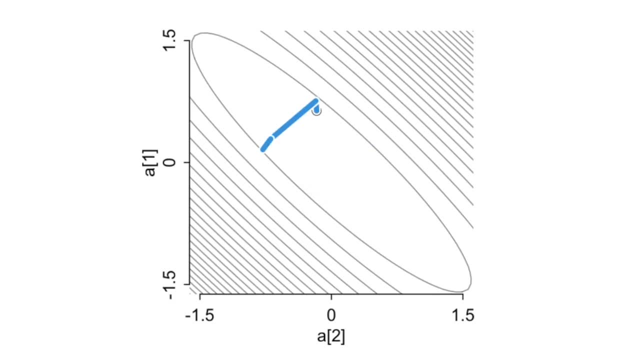 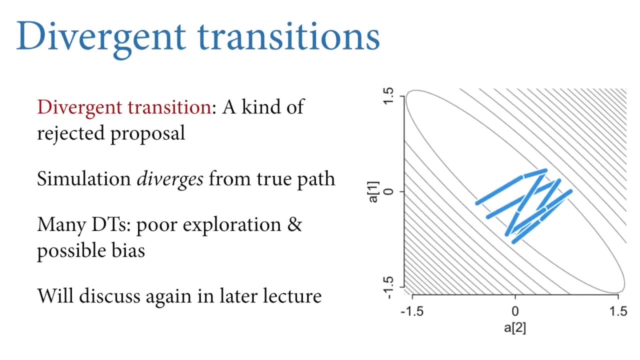 it starts over from where it was before. the red point is the end of a divergent transition. it's a rejected proposal. what is a divergent transition? well, so you learned that Metropolis, the Metropolis algorithm, rejects a lot of proposals, sometimes most of them, unfortunately. 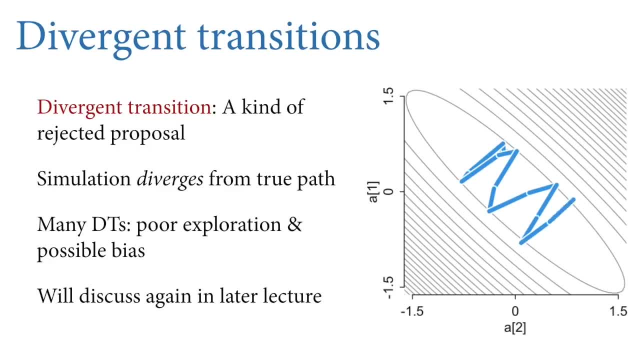 and that makes it inefficient. one of the reasons Hamiltonian Monte Carlo is so efficient is that it it can accept. let's say it makes really good proposals because it follows the contours, the gradient of the posterior probability. it can find good proposals, but it still occasionally makes a proposal. 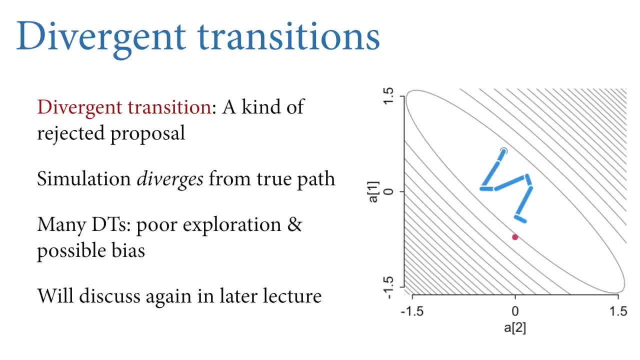 that it won't accept, and these happen when the simulation malfunctions. in a sense, it diverges from the true path. so what does that mean? so there's a smooth skatepark distribution that we're actually trying to sample from, but we can't see it. 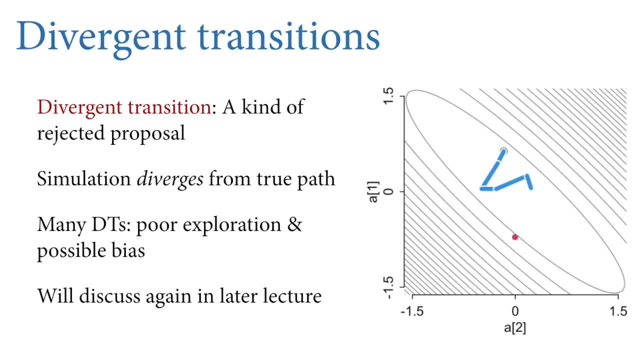 and the simulation we're running is actually discrete. that's what those little bar segments are in the path, and I've made them really big here to exaggerate the point. why? because when the line segments are smaller, we get a smoother approximation of the posterior distribution. 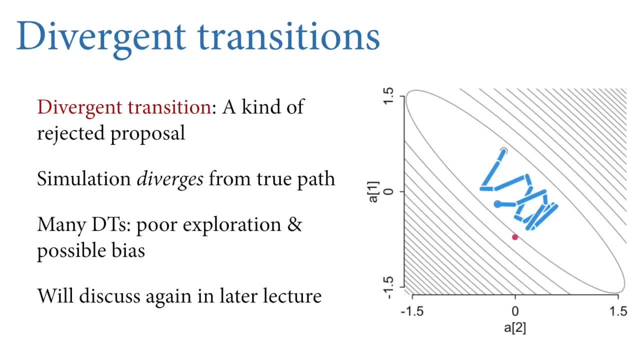 of its curvature, we can roll more smoothly on the halfpipe. but if the halfpipe is very steep in some particular location, which means of course the posterior distribution has a place where it changes very rapidly in posterior probability, then the simulation might have time turning that fast. 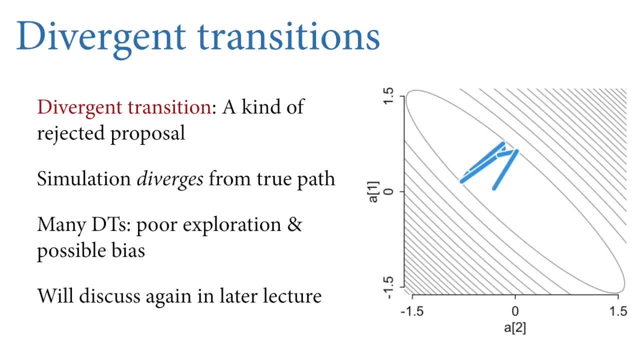 and it could crash into the wall, in a sense, inside the computer, and nothing bad is going to happen there, except that the algorithm will detect that, it has a way to detect this. and because this is a physical system, a simulation of a physical system and in physical systems, 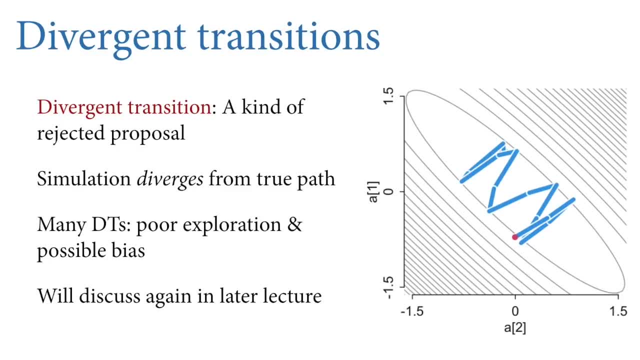 the total energy is constant. there's no friction in the system. nothing's lost to heat, and so if the energy at the start of the path is different from the energy at the end, it's a divergent transition. and then those proposals are rejected and they're called divergent transitions. 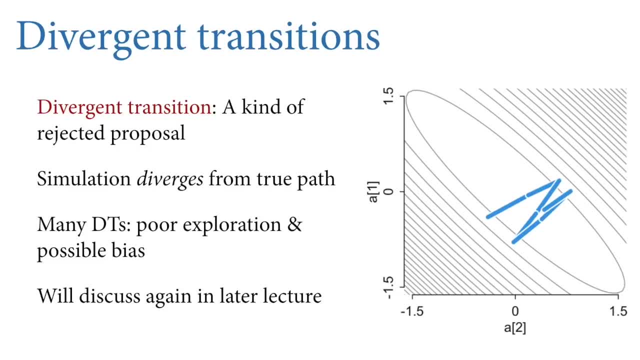 in Hamiltonian Monte Carlo algorithms, so having rejected proposals is not a bad thing. like I said, Metropolis will often reject most proposals, but if you've got a lot of divergent transitions, it could be that the algorithm is exploring the posterior distribution very poorly and it's inefficient. 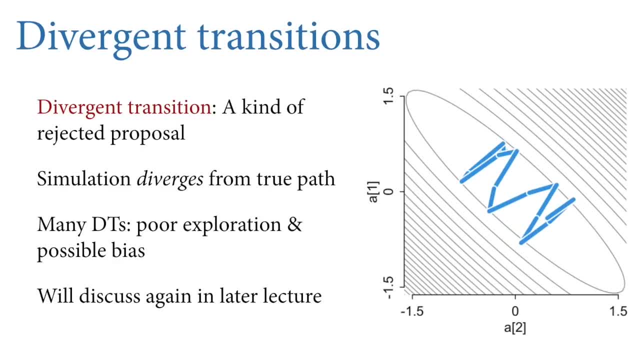 and it could result in bias. if it's always the same region of the posterior where the divergent transitions are happening, then you're not taking samples from that region, and that may not be very good at all. so that's all I'm going to say about divergent transitions for now. 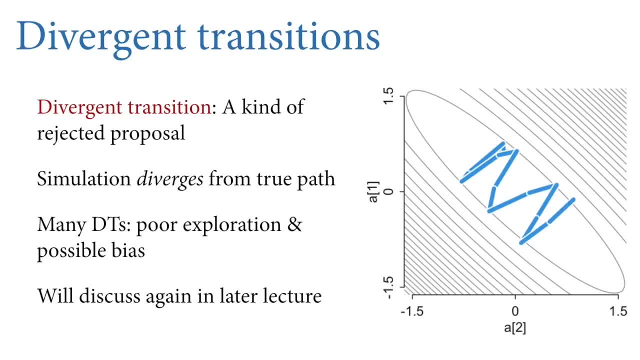 but in a later lecture, when we start talking about multilevel models, I'm going to come back to this and I'm going to show you ways to program around divergent transitions, because they're a fact of life, but we live with them and they're not poison. 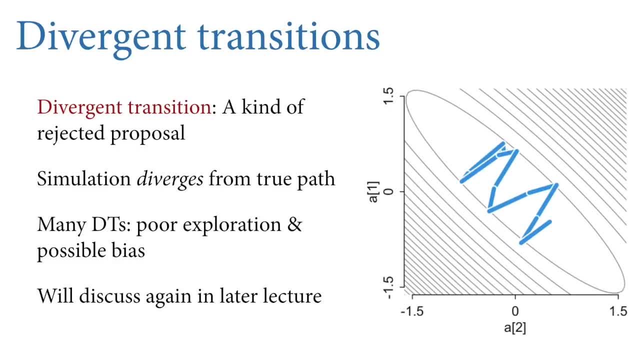 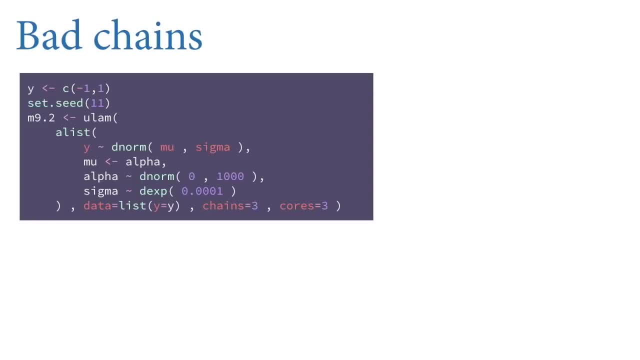 they don't destroy your project and we avoid possible bias. okay, before I end this lecture, I want to show you some examples of badly behaving chains, not just good ones. if you know what to recognize, that'll make you a lot more comfortable. I hope so. here's an example from chapter 9 of the book. 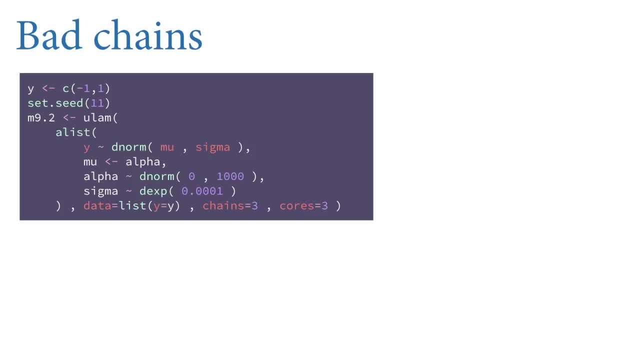 model 9.2. it's a very simple example: two Gaussian observations minus one in one and we're just going to estimate the mean and standard deviation. this is to complain. wait, it's only two data points. you can't do that. remember, this is Bayes. 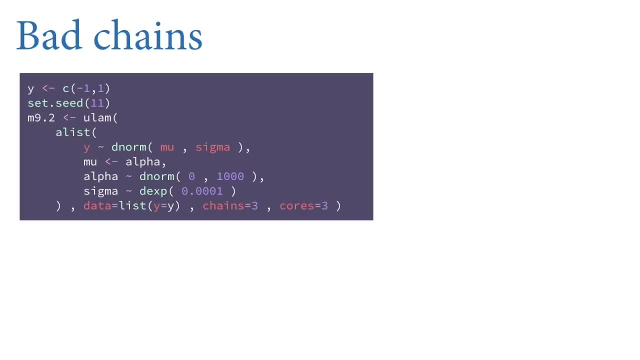 we can do that. the minimum sample size for Bayes is zero. we can simulate from the prior even if we have no data, and we can update the posterior distribution. with one data point, here we have two. this is like luxury. but what's unusual in this model? 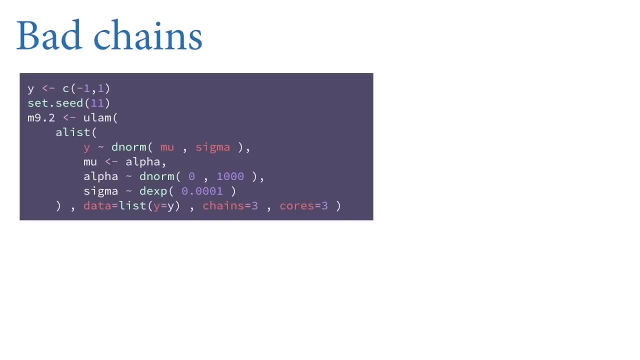 that I've never done before is I've used extremely flat priors with a deviation of a thousand, so that's a huge variance, and this is an extremely flat normal distribution relative to the scale of the data, and then, similarly, for the standard deviation, I've given it an exponential distribution. 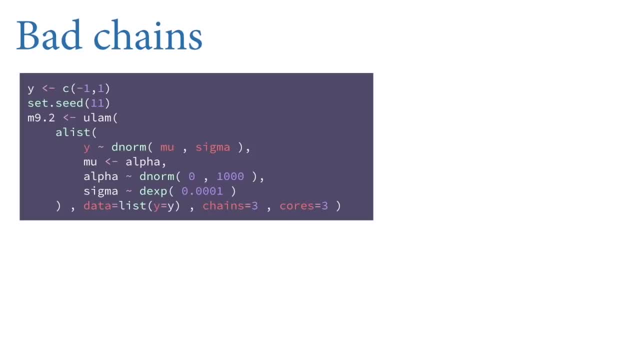 with a rate to 0.0001, which means it declines very, very slowly. so it's very, very flat out to very high values. we run this model using Hamiltonian, Monte Carlo and Ulam, and the pricey output is monstrous. now you know what the mean should be. 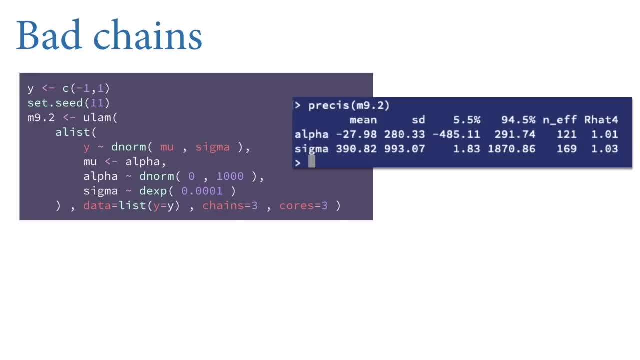 it should be about zero. what's the average of minus 1 and 1? you can fit this posterior distribution with your eyeballs almost. if you look at this, the mean of alpha is about minus 30 and the standard deviation is 280. this model has no idea. 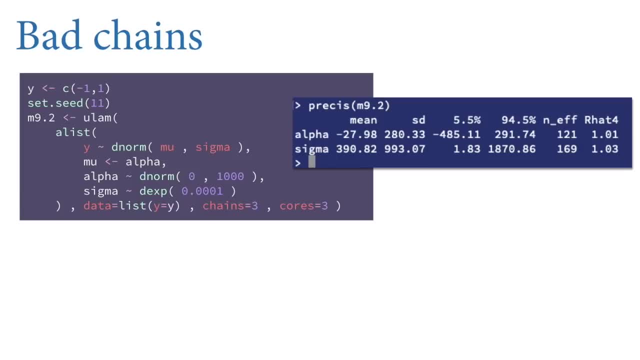 where alpha is, and it likewise has no idea where sigma is, has a mean of 390 and a standard deviation of about 1000. you'll see that these are quite low. actually, the R hats aren't so bad, so this is to give you an idea. 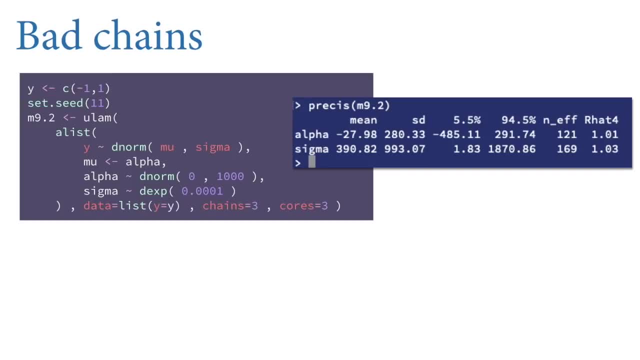 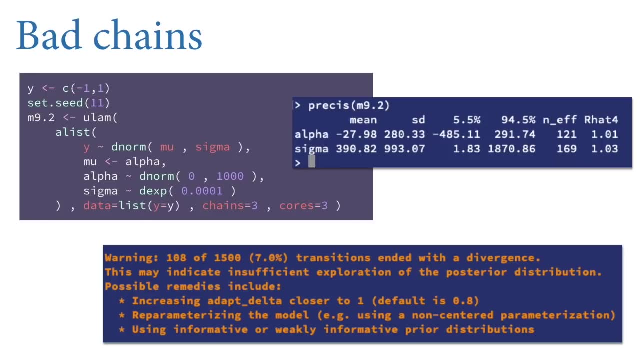 just because R hat is near 1 doesn't mean the chain worked, but the NFs are way below the actual samples that we took. before I move to the next slide, you'll also get a warning when you run this model about divergent transitions, and this is to say that 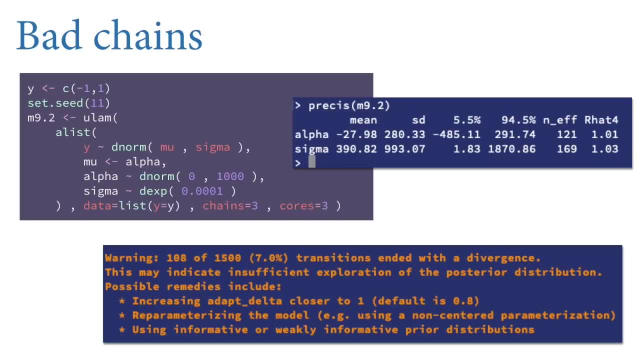 the algorithm was having a hard time exploring this posterior distribution, and that resulted in 108 divergent transitions. it tells you this so that you might want to try to do something about them. you'll see that there's some possible remedies suggested by this warning message, and the third one is using informative 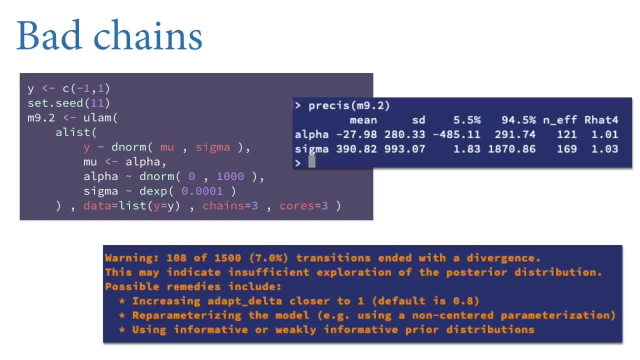 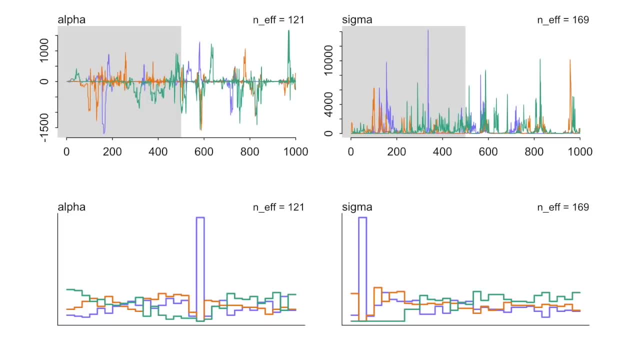 or weakly informative prior distributions, and that's what we're going to do. the problem here is that these priors basically say: the whole real number line is open game for these parameters, and that's not true. what do the trace plots look like? I show them at the top of this slide. 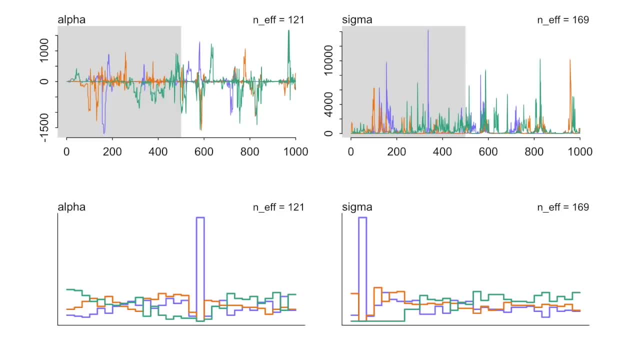 and you'll see that these are not nice, healthy chains. this is a caterpillar illusion here. chains like this maybe in the really long run will give you a reasonable representation of the posterior distribution, but you shouldn't trust them and no one else should trust them either. 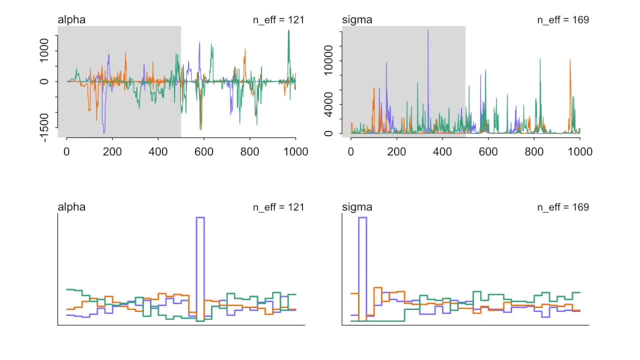 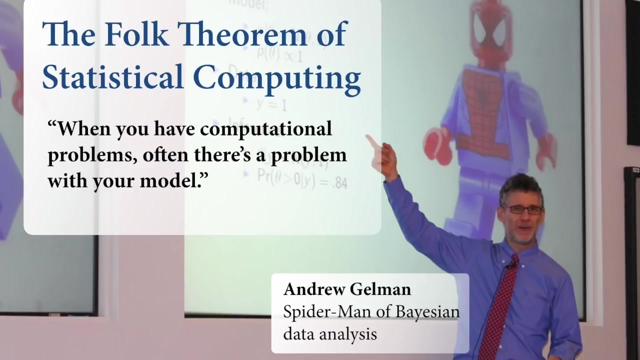 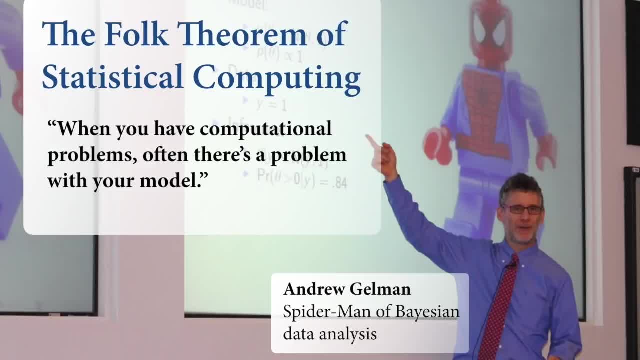 well, you'll see the spider-man above him. um, i think the saying goes that with great power comes great responsibility, and that's the thing about these algorithms. you, we use them because they do really powerful things for us, but we have this responsibility to use them for appropriate. 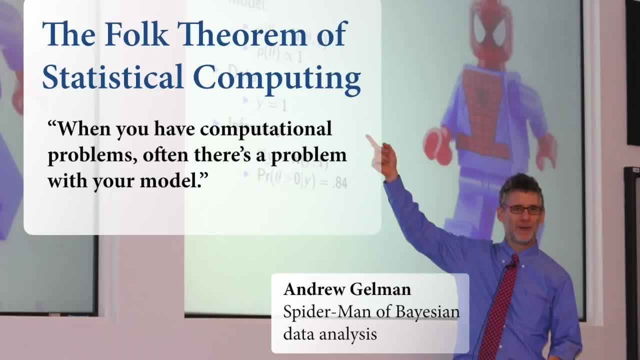 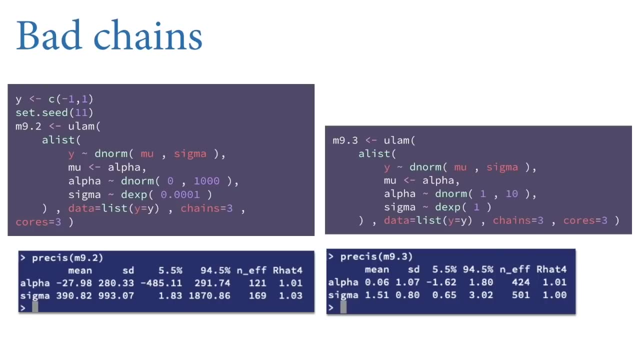 ends for appropriate goals, and that means educating ourselves on what good scientific assumptions are to put into them. you can, you can't fit any arbitrary, uh, scientifically ill-formed model with these algorithms. so that's the folk theorem of statistical computing, and it applies in this case quite well. so on the left of this slide i've showed you the same model. 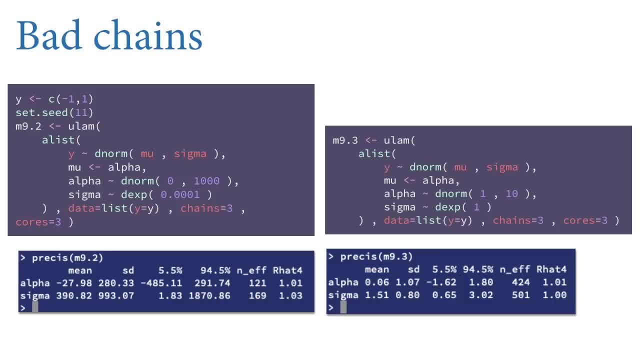 that that gives you bad chains. and on the right i've changed it just so the priors are narrower but they're not all that narrow. so now alpha has a normal prior with a mean of one and a and a a standard deviation of 10.. why did i make it a mean of one? i'm being a bit cheeky here it's going. 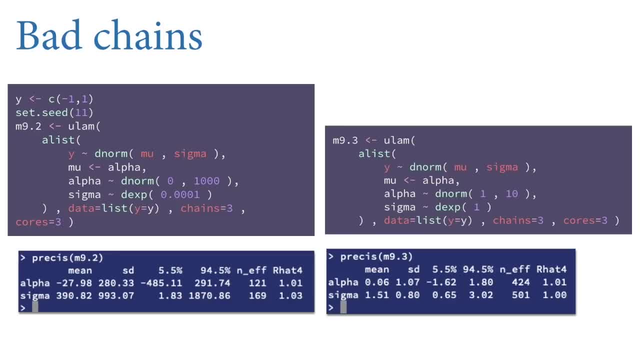 to end up near zero. i just wanted to show you that the prior being wrong does not destroy the inference and a standard deviation of 10 is still a big standard deviation. that's a variance of 100. this is still a very flat uh prior distribution, but it's not a standard deviation of a thousand. 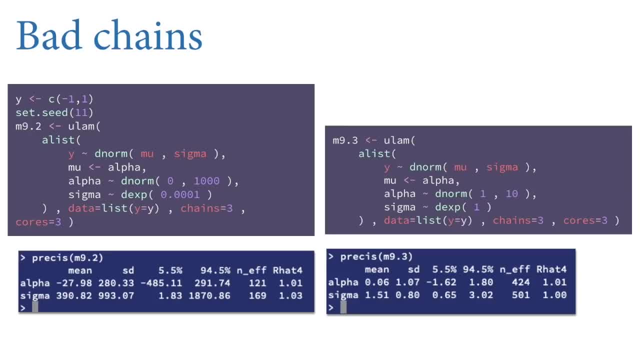 it's, it's qualitatively different, and sigma to have a rate of one, so that means that the the expected average standard deviation is about one. and for standard- uh, for standardized data, of course you that makes a lot of sense, right, but still, this is not a very informative prior either. and when we fit this 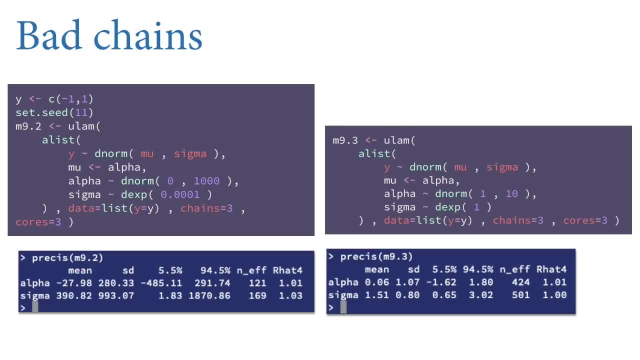 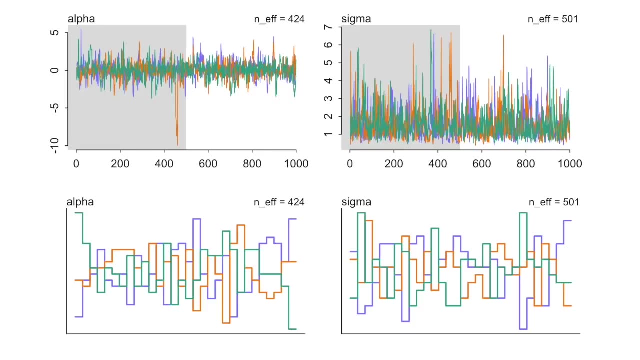 again. now we get quite sensible results and we learn the mean and standard deviation of the data as they were provided. the r hats are very close to one, 1.01 and one exactly, and the nfs are much higher. the trace plots look much better. here we have the hairy caterpillar plots that we see here. uh, you'll see that for sigma. 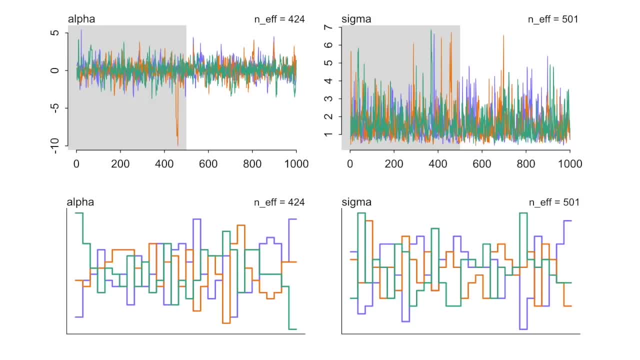 it has an upward, uh, a trend upward right. that the upward tail there is longer. that's very normal for scale parameters. that's, that's not a pathology. that's what the posterior distribution actually looks like. and then the tranq plots on the bottom row look as they should. you see that zigzagging? 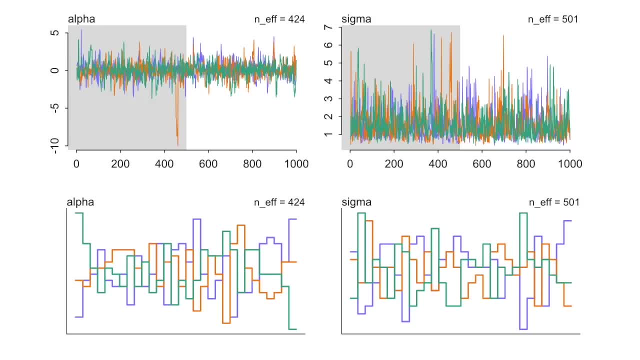 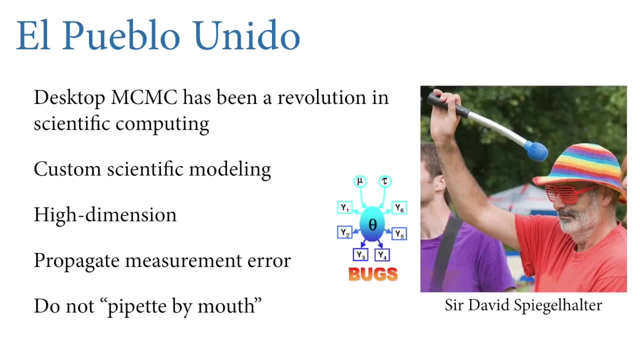 mosaic kind of pattern as the chains swap off. who's on top? okay, we've covered a lot of ground in this lecture. i want to kind of loop back to the big historical picture of these methods. desktop markov chain. monte carlo really has been a revolution in scientific computing and it's not very old, it's only since the 1980s. 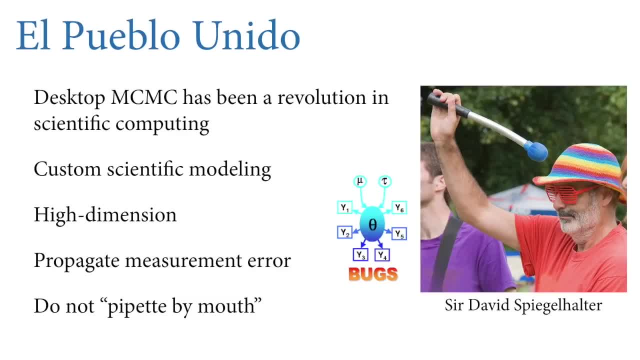 the end of the cold war, really when this desktop markov chain monte carlo revolution began, and it was begun by statisticians like sir david spiegelhalter, pictured there on the right, and his colleagues who had this wild idea to start a project called winbucks. 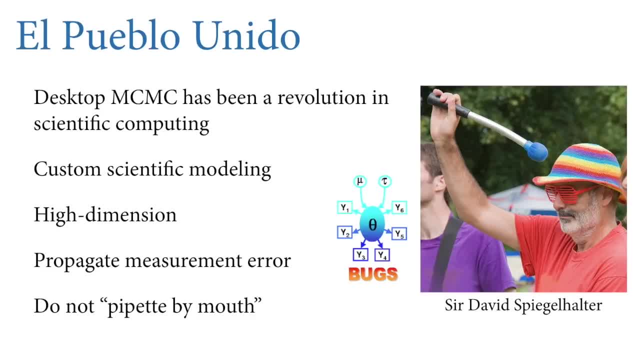 where the user, the scientist or the consulting statistician could specify arbitrary statistical models in the forms of probabilistic assumptions and, like we've been doing in this course, and then the software itself would would figure out the problem of designing a markov chain sampler for it, so that you didn't have to muck around with that part of it, and this radically accelerates. 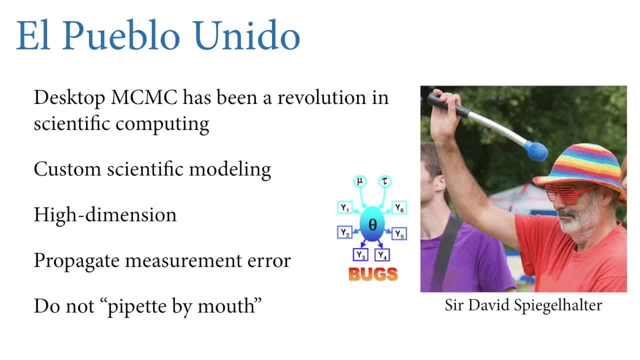 uh, scientific discovery and it catalyzed a bunch of of later computer software development and also stimulated a bunch of really deep mathematical research into markov chain algorithms. this has been a fantastic thing and in all of this scientific computing has been in the forefront, something that's not often given as much credit as it deserves, because it's really enabled. 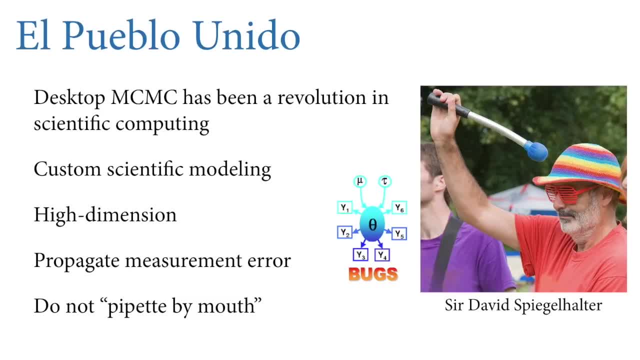 scientists to take charge of their research projects. they're no longer hostage to the sorts of algorithms that any particular statistician wants to program for them. they can come to their problems with their models and they can program them directly in software like bugs. i don't think very many people use bugs anymore, or stan, or turing or some other kind of modern. 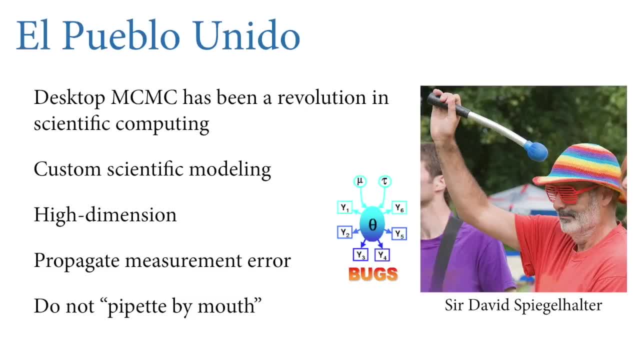 probabilistic programming language and we can work in high dimensional problems and many insights. important scientific problems are high dimension. we can do very important things like propagate measurement error. we can do very important things like propagate measurement error. we'll talk about that near the end of this course, but all along, of course, for this to work for us.